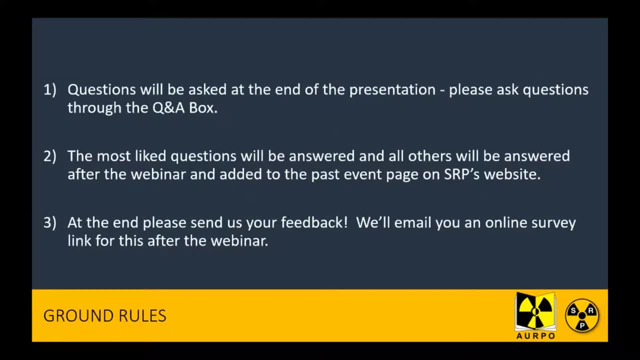 If you click on there, you can ask any questions throughout the event. If you see a question that you particularly like and want answered, please click on the like buttons, because we normally get so many questions throughout the event. We will try and answer as many of those which are highest liked. 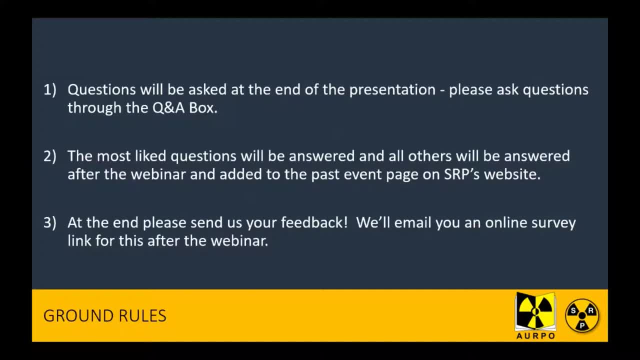 Anything else we'll take away at the end of the event and we'll email out something which is the answers to all of those questions. If you have any questions, please feel free to reach out to us through the Q&A box at the end of the event and we'll try to answer them later on. if you also would like to claim CPD points from these webinar programs, then what you need to do is, within that Q&A box, you will see Charlene's put up a statement at the start which gives you a code. 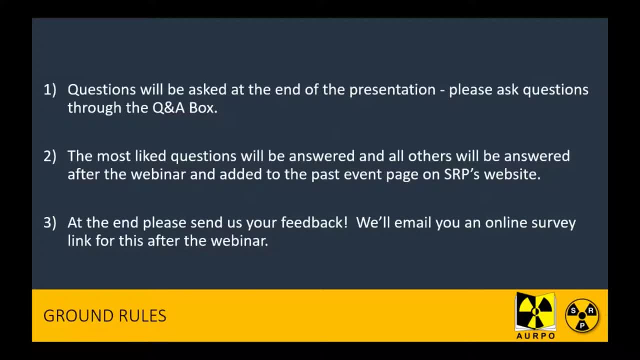 What you need to do is email that code to Charlene, and she will send you a confirmation email that you attended the webinar. This can then be used for CPD purposes. As always, please also send your feedback at the very end of the event. 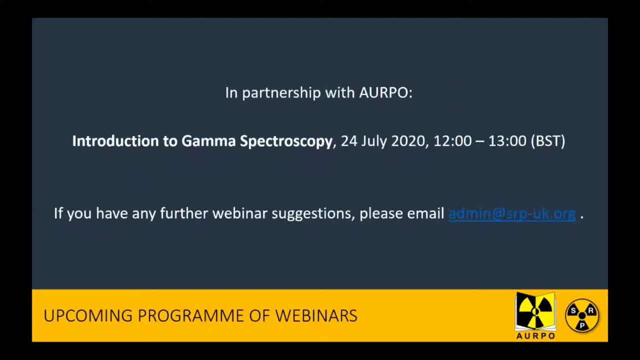 We always want to hear about new webinar suggestions And also what you thought about the event as well and how we can improve it. We've got a new webinar coming up shortly, which would be also in partnership with AURPO, on an introduction to Gamma Spec, and that will be on the 24th of July between 12 and 1.. 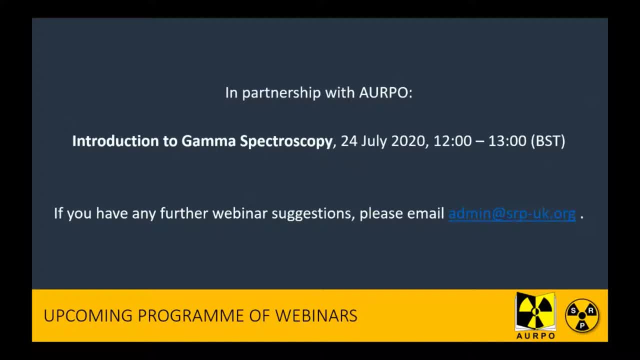 But we've also got many other topics in discussion at the moment which we're looking at running as well. So, don't worry, the webinar program will keep on going. But with that in mind, I'd like to introduce our next speaker. just to do a quick introduction. 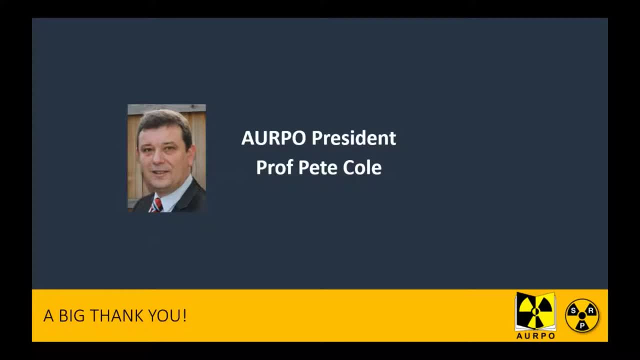 His name is AURPO President, Professor Peter Cole, which I'm sure a lot of you already know. So with that, over to Pete. Hello everybody. Thank you, Pete. Welcome to those attending this webinar from the UK and also to those attending from various different countries around the world. 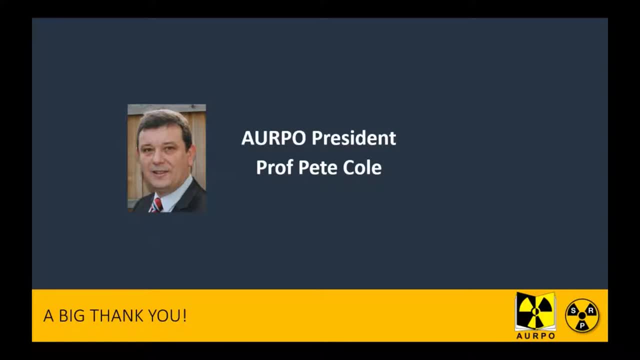 Everyone is most, most welcome. Once again, it gives me great pleasure To say that AURPO is collaborating with SRP on the provision of this series of free online training webinars. These are not only aimed at the needs of our membership, but are also hoped that we hope, aspire to support the wider radiation protection community and promote knowledge exchange both nationally and internationally. 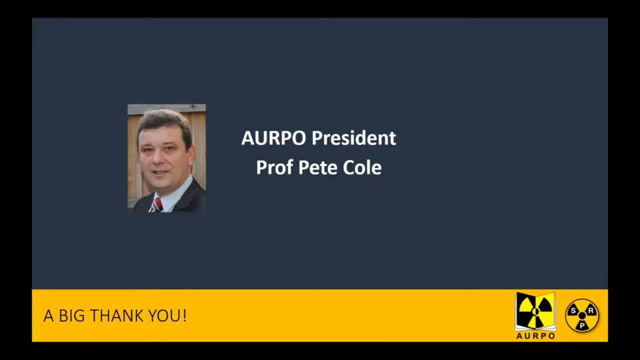 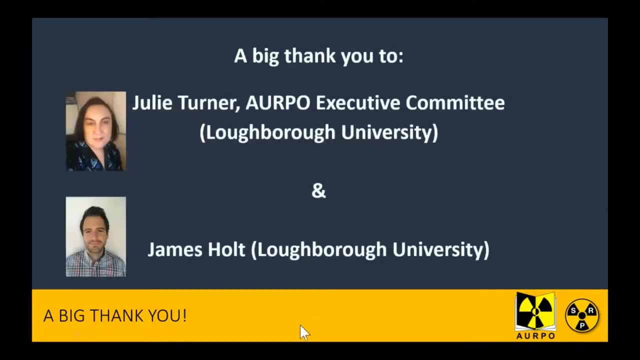 So today's webinar Will be presented by Miss Julie Turner from Loughborough University, where she is a strategic scientific development officer and radioactive waste advisor. At Loughborough she leads on radiological, biological and chemical safety and has worked in the field of radiation protection for over 20 years. 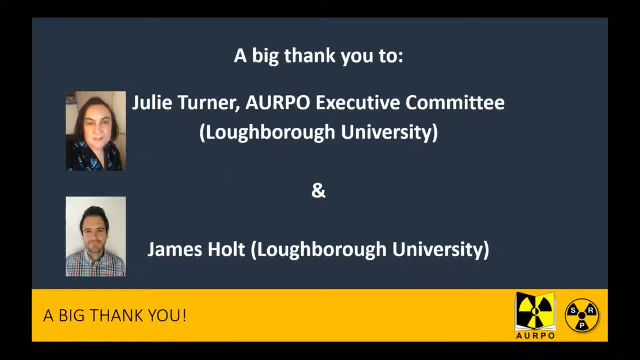 Julie is my colleague on the AURPO executive committee, Where indeed she is the AURPO RPO Treasurer and Membership Secretary. So today's webinar is all to do with decommissioning of non-nuclear radiation facilities, and Julie's going to draw examples from a Loughborough project which 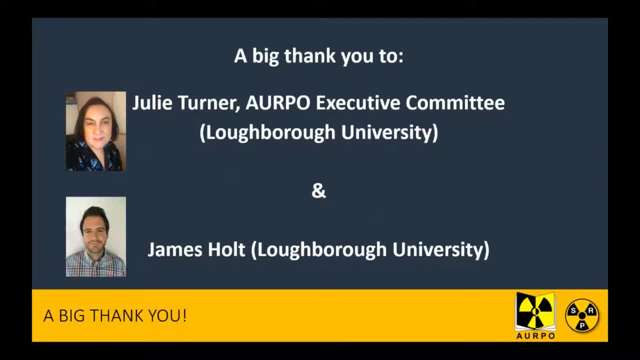 was the decommissioning of a 60 year old radiochemistry facility. She'll be assisted today by Dr James Holt, who is a radiochemist and is part of Julie's team at Loughborough where he is a radiation decommissioning officer. James will join in towards the end in the Q&A session. 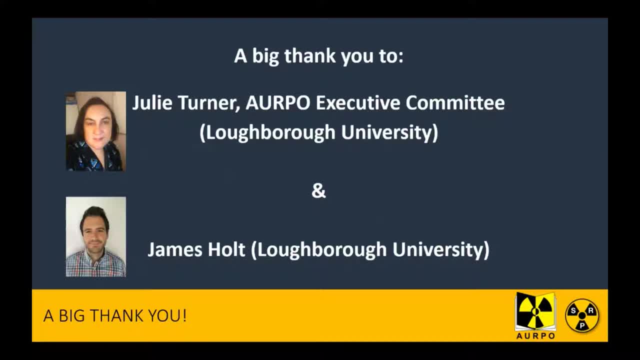 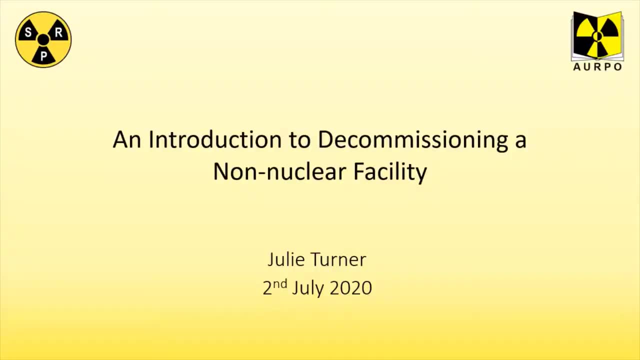 at the end of this presentation. So, without any further ado, I shall hand you over to Julie. So thanks for Pete, for the introduction. As mentioned, this is an introduction to the decommissioning, a non-nuclear facility, which is indeed a 60 year old radiochemistry building. 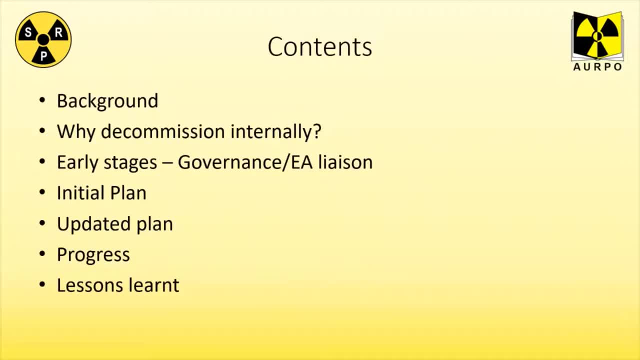 I'm going to talk to you about the background. So the background of the decommissioning of a 60 year old radiochemistry facility, Why it was there, how it's been used, why we decided to decommission internally- because that's quite unusual for a university, for a whole building. What the early stages of that process. 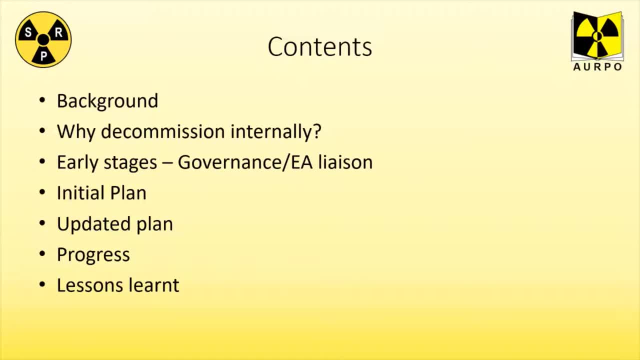 was the governance and our involvement with the Environment Agency around this, our initial plan and then our updated plan once we'd actually done some historical research, the progress throughout this decommissioning and, some of the importantly, some of the lessons learned and some of the experience we've gained from doing this. It is going to be a whistle-stop. 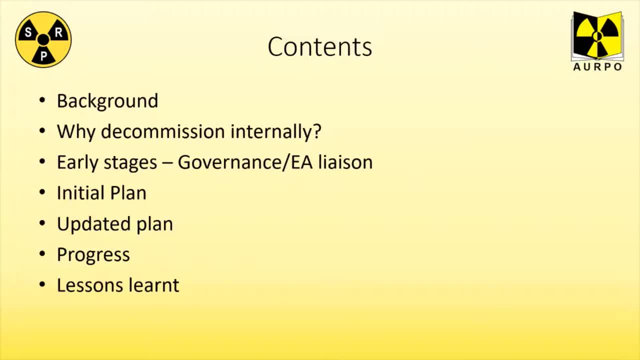 tour because obviously the timing- this project's been going on for two years and there's so many things we could tell you about, So I've tried to condense it down into interesting areas that you might find useful. So the Graham Oldham building is in the middle of our university campus, in our 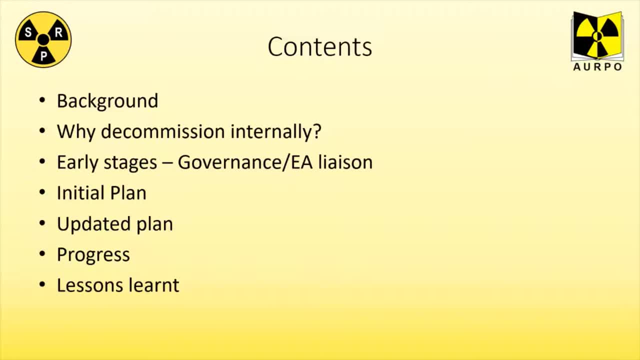 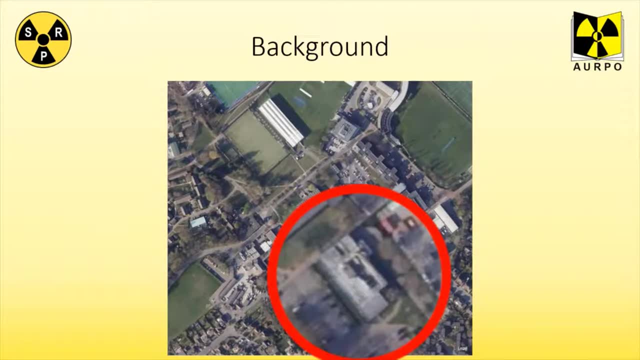 Central Park and it's got a little circle coming up now. So it's right in the middle. it's got a chemistry building next to it, it's got lots of other areas, so it's not really away from anywhere else. It was built in 1990 and it's been used for a long time. It's been used for a long time and 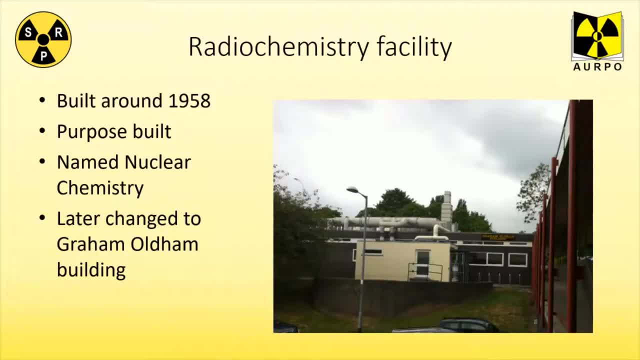 it was built in 1958 and it was purpose-built for radiochemistry work, So it was actually built for that purpose. Originally it was named the Nuclear Chemistry Building, which did cause some anxiety for the local neighbours around the Loughborough area and later because of those kind of challenges. 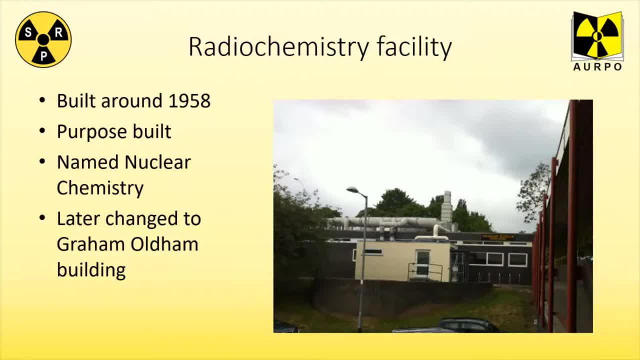 it was changed to the Graham Oldham Building, named after the first radiation protection officer who worked within there, And you can see from the photos. you can see the extraction and the chimney circle that was in front of the building, which was there to provide shielding for a cobalt-60. 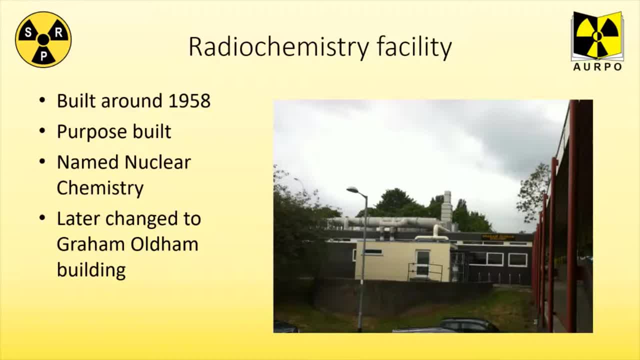 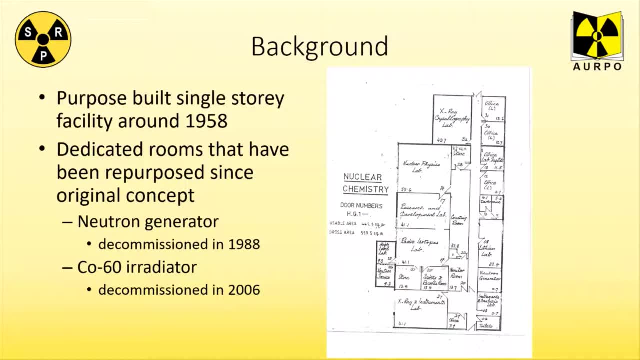 irradiator source. So the purpose: it was purpose-built and- it's one story- It had dedicated rooms that had been repurposed since the original concept. So on the original map here we had a radioisotope lab, nuclear physics lab, but we also had a neutron generator which had tritium targets. 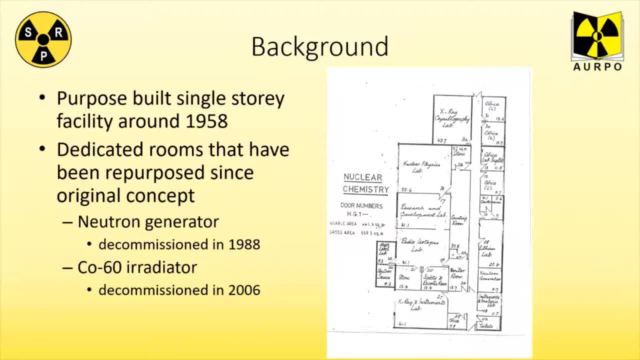 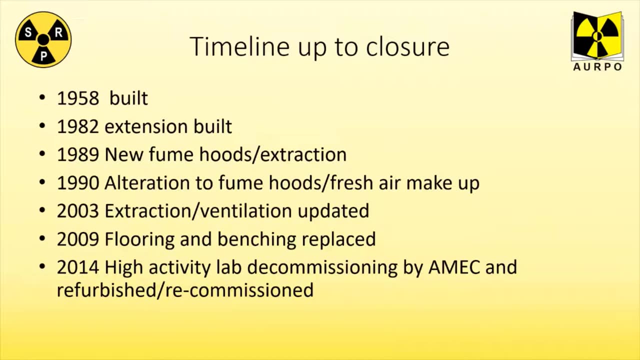 that was decommissioned in 1988 and the cobalt-60 irradiator which was decommissioned in 1988. And we have the records for those. so we know that was successfully done. The timeline up to the closure: we had the extension built in 1982 which added on a. 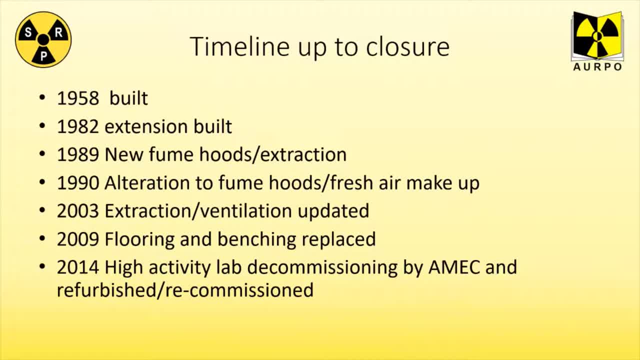 x-ray facility and more offices. Then between 1989 and 2003, we had additional extraction and ventilation updates and you'll see these in some of the plans. In 2009 they completely replaced all the flooring and changed the wooden benches to trespass benches. So we had a lot of work. 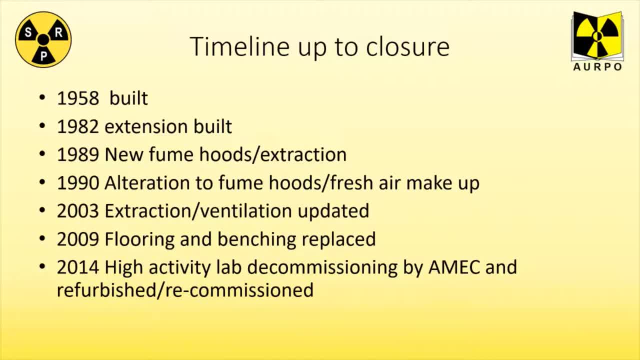 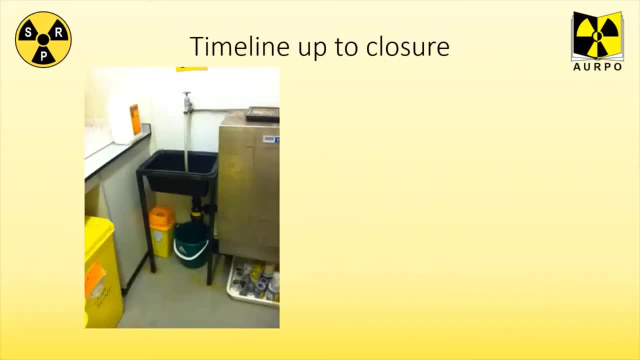 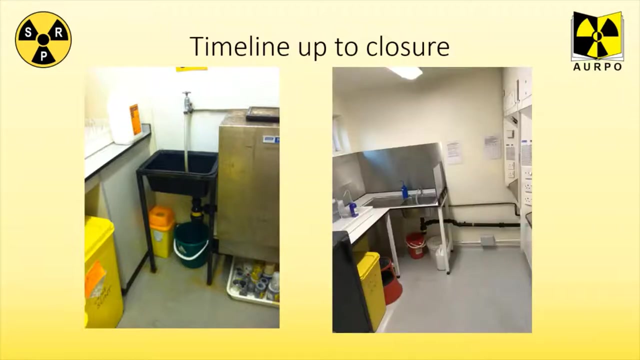 on the interior, We had access to all the methods of defecation and, of course, also to the, a much more modern facility with splashbacks and much brighter. we changed the lights and everything, so that work was done in 2014.. So this is the current building. I'm just going to take you. 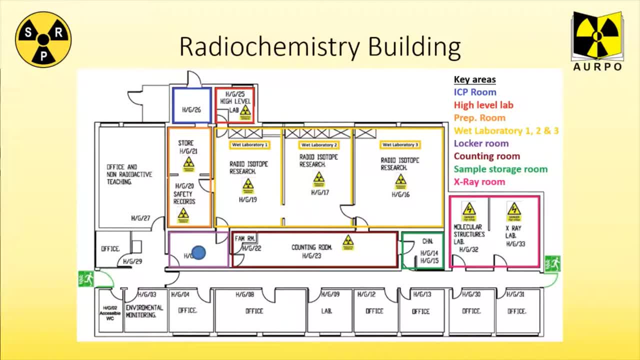 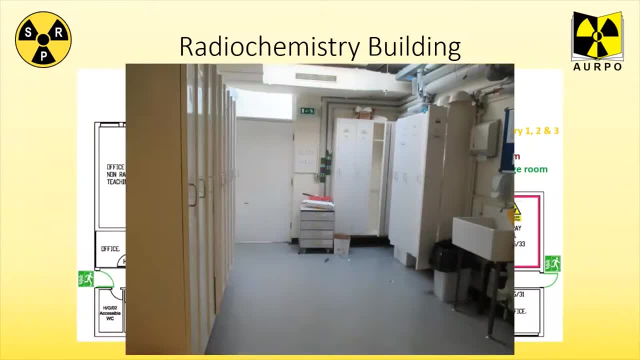 through it so you can see what we were up to when we had to decommission. So as you go into our radiochemistry facility, you would go into the locker room which obviously had all the lab coats, it had cleanup kit, emergency spill areas and also was the entrance to the supervised areas. 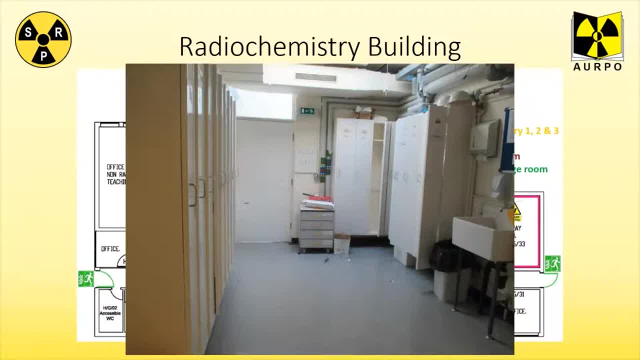 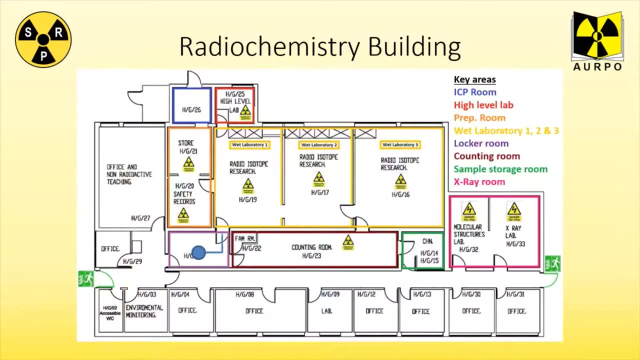 Now some of these photos have been taken since we started the decommissioning, so it'd be less busy than what it was when it was actively being used. But if you go into the map you'd go into the first of our three main laboratory areas, which you can see, hopefully, on the picture coming up. 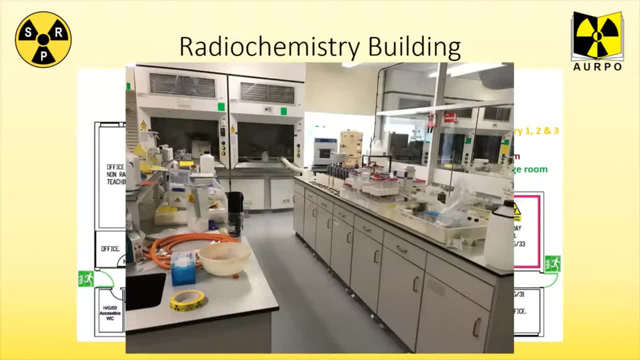 these had the labs, so the students would work at benches that have all their radioactive items in those trays. but because this whole area was used for radiation work, it was assumed that most things in this area could possibly be radioactive. So in fact we actually labelled non-radioactive things more than the rest, because we knew 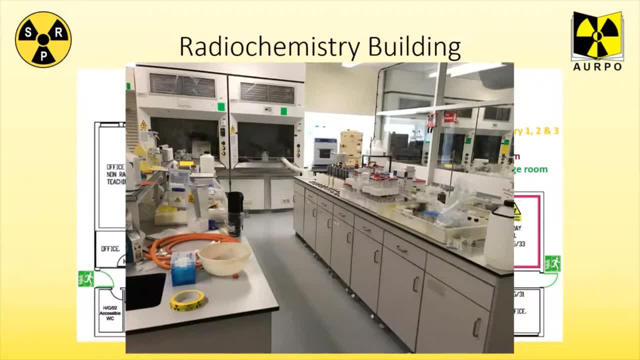 most things were radioactive. We had fube hoods that the students were constantly use, lots of pipettes, lots of tubes, of course, as you would expect, We then went into sort of a prep area, which originally had a biosafety cabinet in it as well. 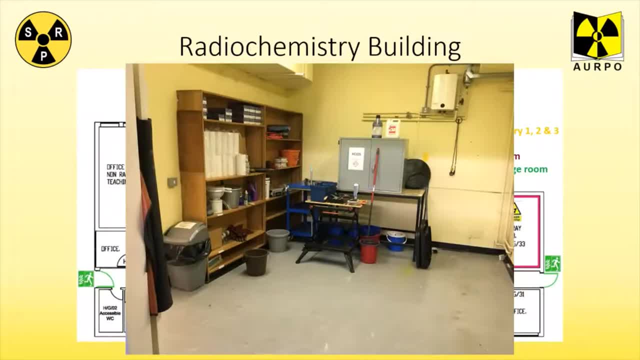 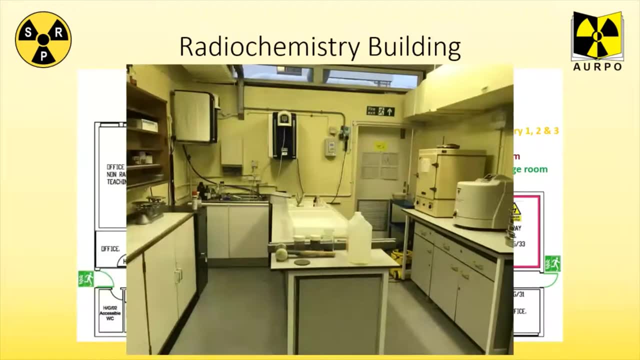 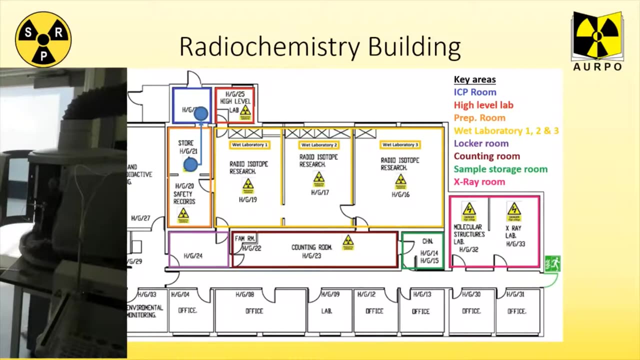 had lots of files, chemicals, incubators and also purified water- all the things you would expect in a modern chemistry practice. So we could not quite go as far as the low and low and low camp area. I had a little room coming off that, which is where the ICPs had sat. So we had an MS-ICP and an OES-ICP. 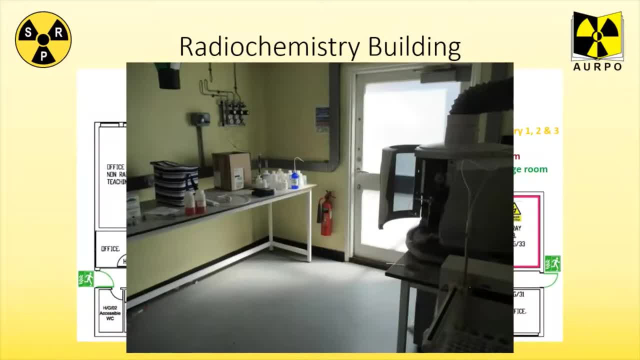 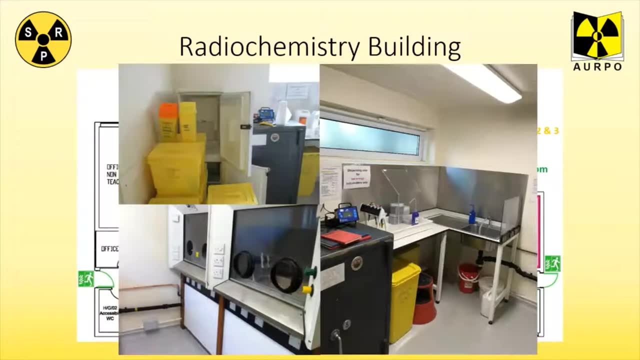 which has been gone in this photograph, but that was used for some of the students samples And then back into the high activity lab that I showed you on the previous slide. but this also shows you the fume hoods where they did the dispensing. we also had a lead cave for some of the really active gamma emitters. 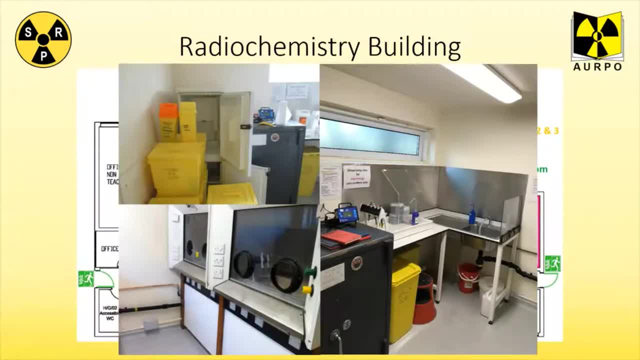 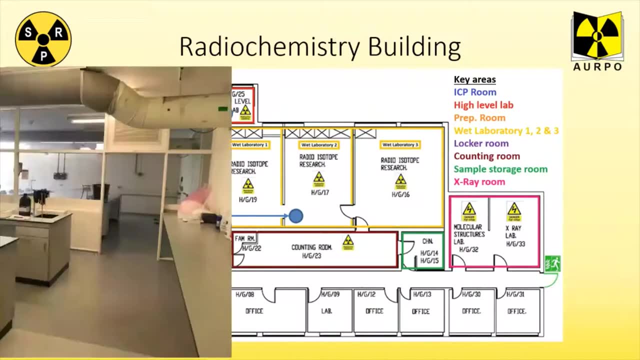 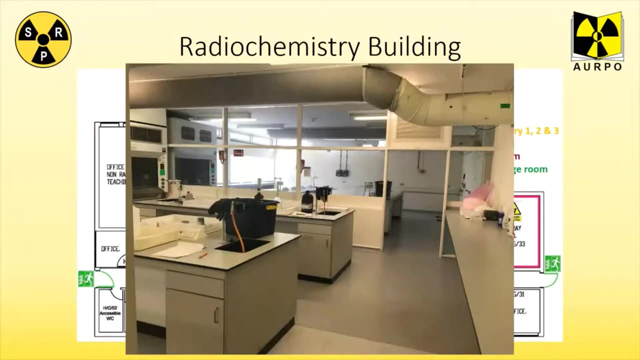 for the sealed sources and it's also where they kept some of the waste sim bins. then across to the second main area again. you can imagine this would have had all the trays of all the student samples in the side bench would have been full with phd, ph meters, balances completely in use. 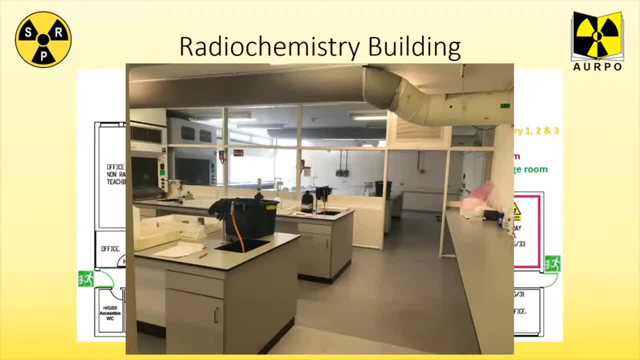 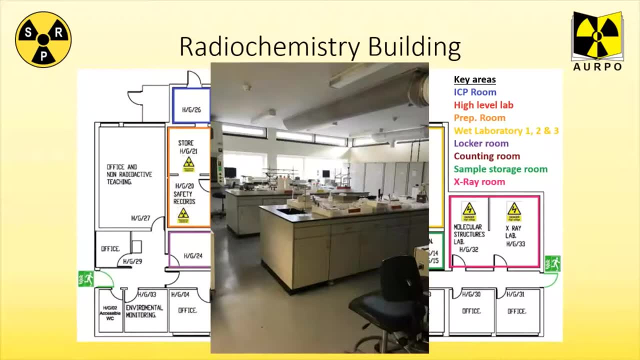 this is after we started decommissioning, so it's quite empty, appearing then into the final section of the lab again trays of student works. we used to have a glove box in this area for alpha emitting radionuclides, and you can also see on the ceiling the air socks brought the fresh air into the lab. 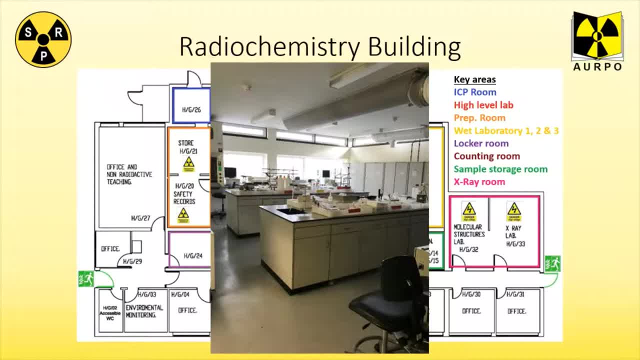 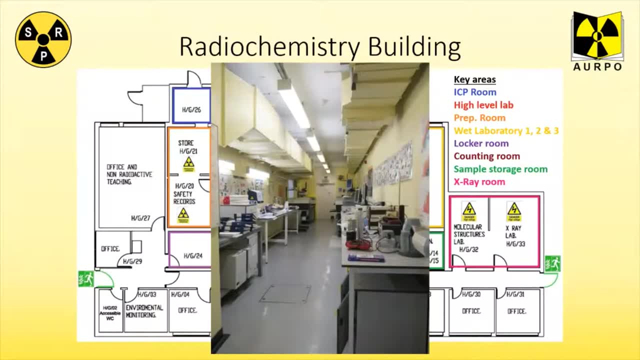 as the fume has drew out the older air. we had a county room which had liquid scintillation counters in gamma counters- icps- uh sorry, not icps- um, gamma spec, alpha spec and also an xrf which we've had a lot of work on. so we've had a lot of work on this area and we've had a lot of. 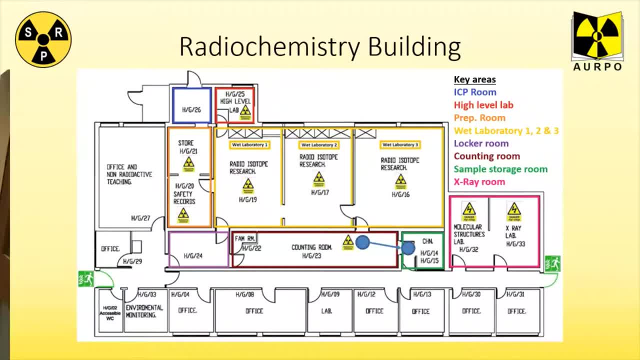 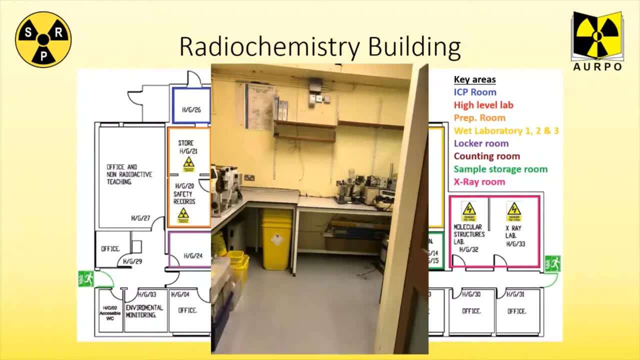 work on this area and we've had a lot of work on this area and we've had a lot of work on this area. we used for the analysis. there was a storeroom which had additional equipment and extra samples, but did used to have a glove box that had long-term air sensitive experiments in as well. 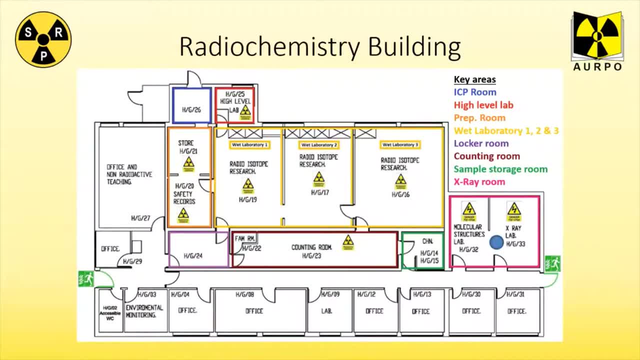 and then, finally, on the end- this is part of the extension- there was a new x-ray lab built which had four xrd units, the typical modern ones, which are completely enclosed and interlocked. so they are on the extension. at the end, what did they do in the radiochemistry? 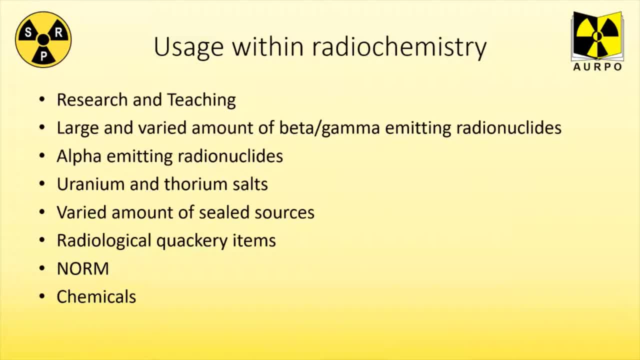 buildings. well, they did lots of research. radionuclides specific to the nuclear industry and their transportation throughout cement was a big focus on a lot of research, relationship between radionuclides and polymers as part of the potential cleanup operations, absorption experiments of clay in the presence of humic acid. so lots of different types of research, particularly around 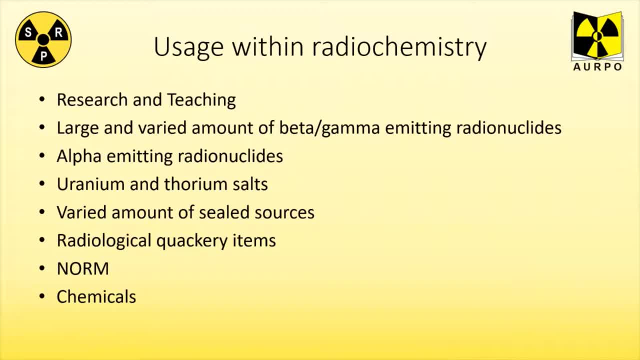 the nuclear industry. um, then we also had lots of teaching. so there was teaching with carbon 14 labeled paracetamol, ion exchange experiments, and a lot of the teaching was carried out within that laboratory. so they had undergraduate practicals of sort of around 20 to 30 students in there and they also 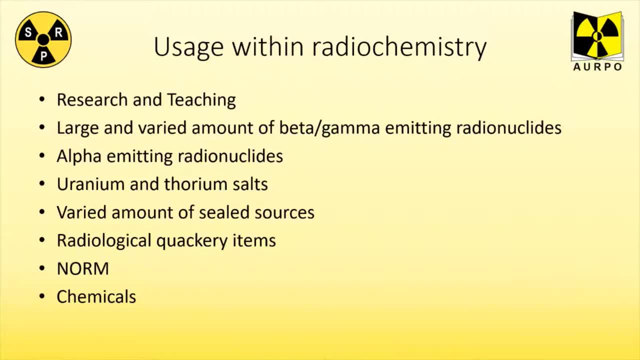 had project students doing very specific work, so that meant this building had everything from really low energy beaters like tritium and carbon 14 right up to uranium, plutonium and radium sources. we also had natural uranium and thorium salts that were used for experiments. 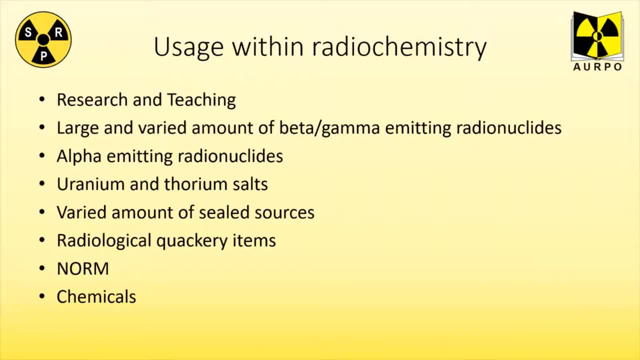 sealed source is mostly the seal sources. after the cobalt 60 source was decommissioned were sources for calibrating radiation monitors or calibration sources for the equipment. so quite low level sealed sources. we also have quackery items, so radiological interesting items like old. 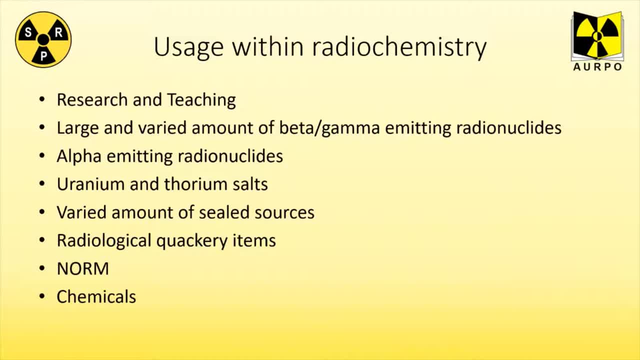 items that could have been used for radium, so sort of suppositories and courses and all types of things you've seen in uh in museums. we had quite a few selections of these which students would look at and be interested in. we had norm, so we had sand samples, rocks, oil and gas scale. 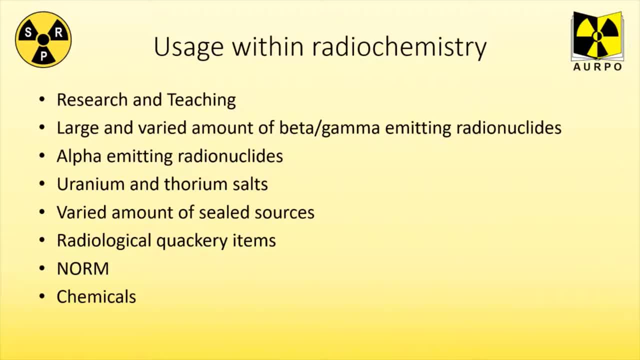 all sorts of types of norm, and then typical chemicals that you would associate with a chemistry department. so lots of different things. so why, then, did we decide to close this facility? well, first of all, the academics- the main academics within this area- left to go to other organizations. 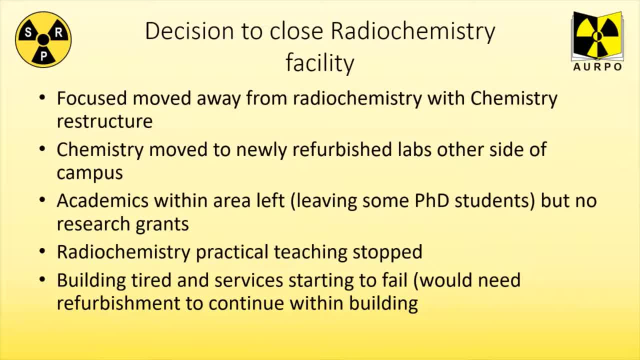 and this at the same time. chemistry were asked to restructure and to simplify what they did. so it made sense to stop the radiochemistry element because it's quite an expensive part, but also the academics were leaving that area anyway. chemistry- the main chemistry builder- was moving to a new refurbished labs on the other side of campus. that would have left a massive gap. 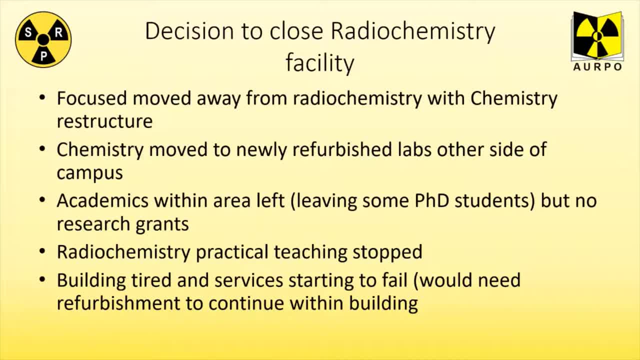 about a mile distance between the chemistry and the radiochemistry area. radiochemistry practical teaching had also stopped at this point and with the building was starting to look tired, we would have had to refurbish. you would have had to replace the first one in the flooring and done some refurbishment. so it's a good time to say: okay, let's stop. 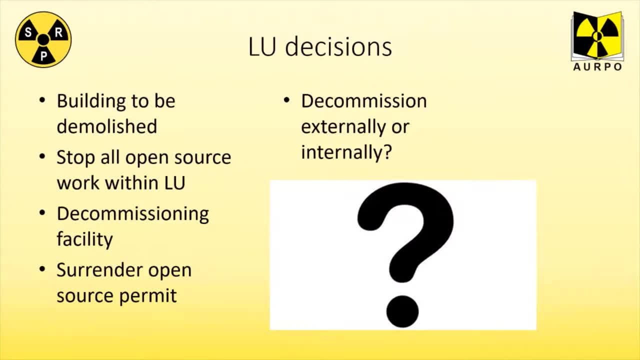 So that meant Loughborough University had to make some decisions If we were going to stop open source work- and this was the only building which had open source radioactive work in Loughborough. so if we were going to stop all open source, then we may- then we're going to have to surrender our 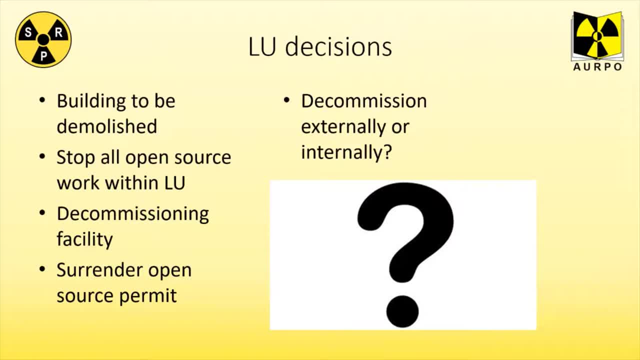 open source permit and to do that we're going to have to decommission this facility. They also decided they wanted to demolish the building, so the building that the area could be used for further development if needed. So we needed to decide whether we were going to decommission. 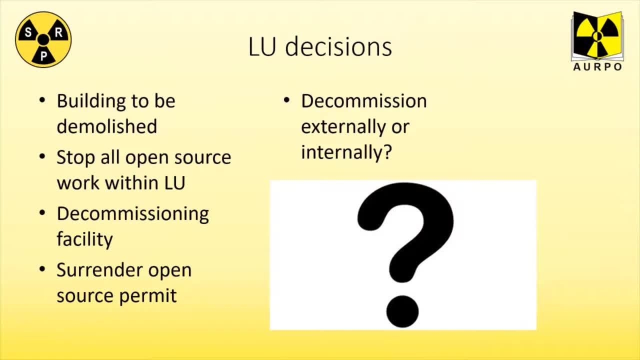 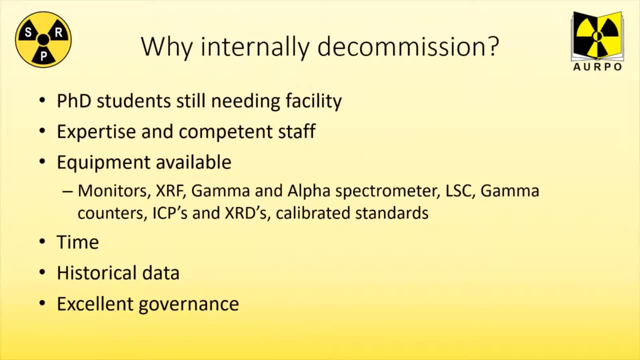 externally or internally, and the reason why we decided to decommission internally was partly based on the fact we still had PhD students. So the academics left, but there were still some PhD students who remained at Loughborough and they were going to be there for another 12 months or so. 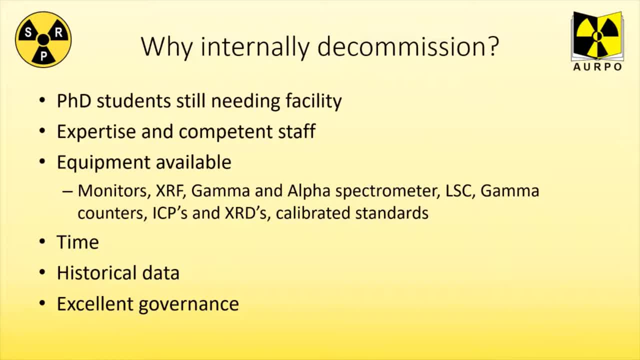 So we could start decommissioning around those students, leave them doing their work. we could start taking out some of the consumables and some of the other items around the area. We also had the expertise and competence in our staff. We had three postdoctoral researchers who have got PhDs in radiochemistry. 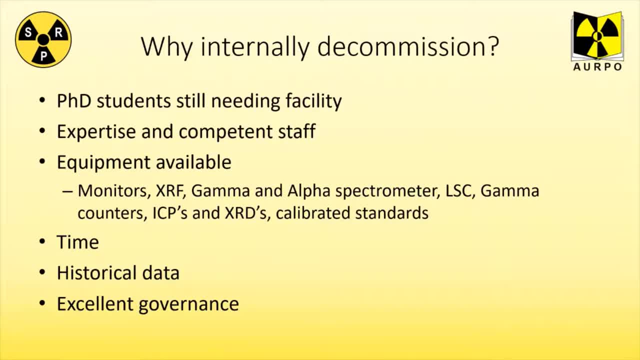 we had an extremely experienced technical staff and, of course, radioactive waste advisor and an external RPA, So we had all the people that we needed. We also had chemists and other competent people. We have all the equipment. we have the radiation. we have the radiation. 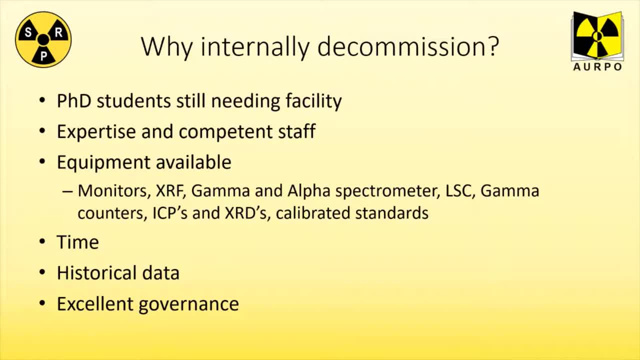 monitors. we had XRF, gamma and alpha spectrometry, liquid scintillation counters and, importantly, we had the calibrated standards to go with those. Another important factor is we had time. There was no rush for this building. there was no rush for the university to get us to surrender the 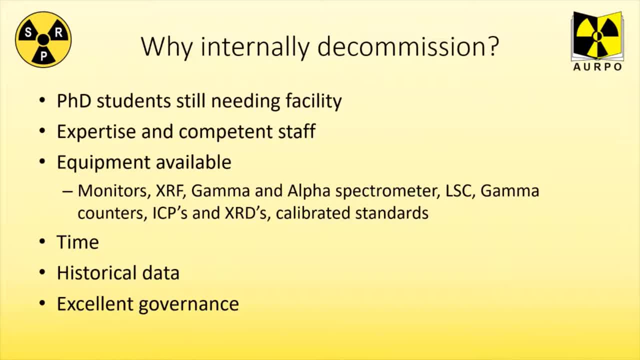 permit or knock the building down, So we could do this quietly and carefully over a couple of years. We had brilliant historical data, and I cannot tell you how important historical data is. It means we could prove where things were decommissioned previously, we could have a look at what went wrong previously and we found out some quite surprising things. 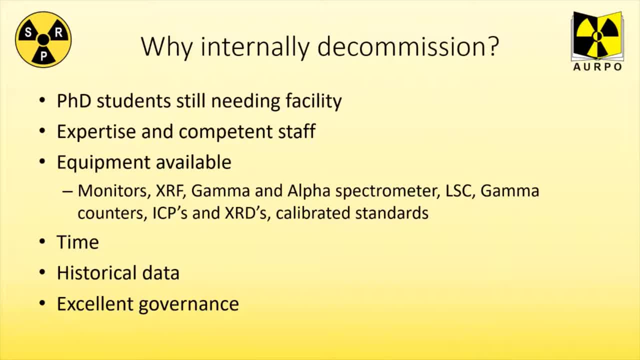 looking back at the historical data. We also had a good governance system in place to keep it all and make sure that we have the correct scrutiny to do the job successfully. So once we decided we were going to do it internally, we had to look at what we needed. 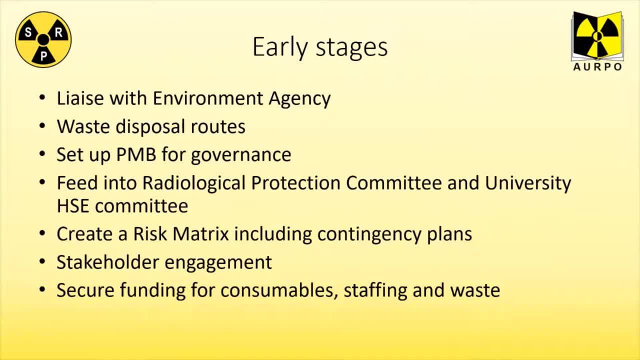 to do in the early stages. The most important thing we needed to do was liaise with the environment agency, and I'll speak more about that in a moment. We needed to look at all our waste disposal routes. How are we going to get the waste away from the area? What were we going to do? 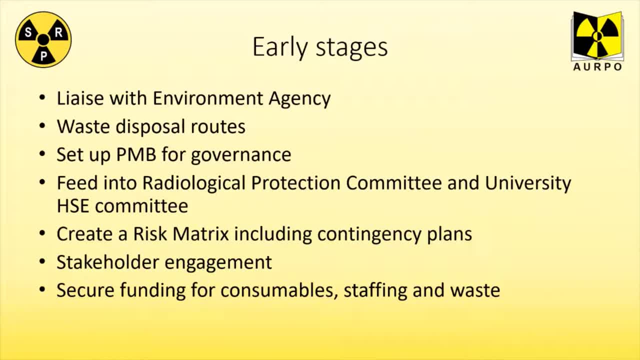 We needed to set up a project management board to give governance and apply that scrutiny that we needed. So on this project management board we had chemists, so we had professors to give us that scrutiny around the science that we were suggesting. we had the people from the decommissioning team. 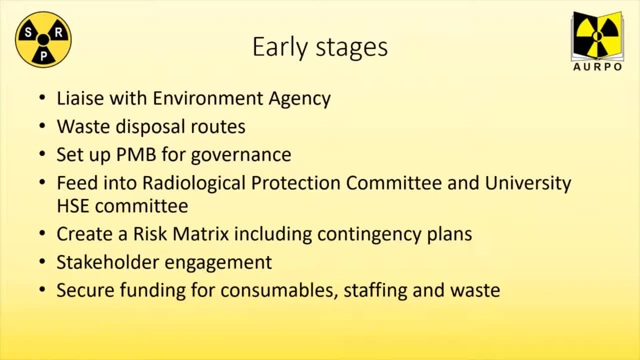 we had the head of our health and safety service, we had myself, we had the facility finance and planning team, and that was chaired by a member of the senior leadership team who actually was our finance director in this case. But we also needed to. 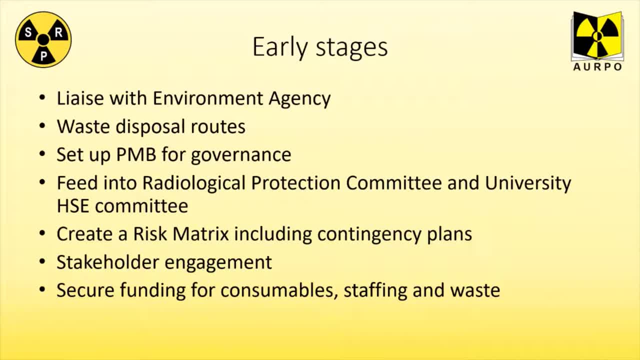 feed into the radiological protection committee because we needed to make sure that we were doing everything safe and in accordance to our permits. So it fed into our RP committee, which was chaired by our chief operating officer, and into the university health and safety environment committee. so it had a lot of governance around it. We were required to have reports going out to all these. 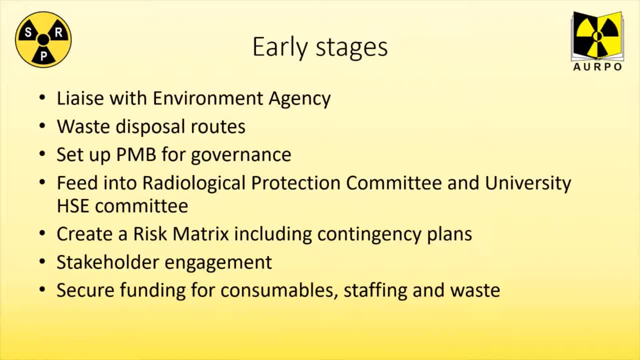 departments on a regular basis. We created a risk matrix so we could really understand what happens if things went wrong. If we started to take the flooring off in an area, what would we find? Would we have the waste capacity on our permits to dispose of it? All those kind of questions were 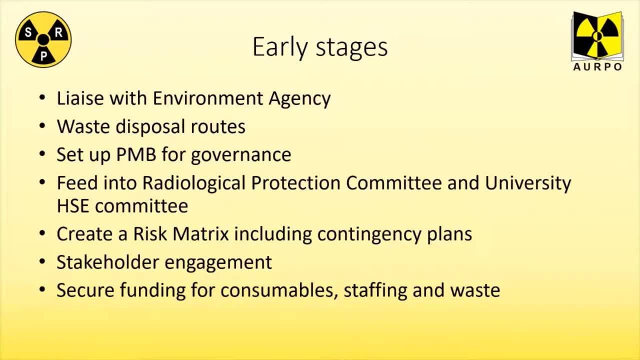 there. We then engaged with some stakeholders- the neighbours, the PhD students who were still in the lab, the chemists, all the people around- and make sure that everyone knew what we were doing and were happy. And then, of course, we had to secure funding for the consumables. 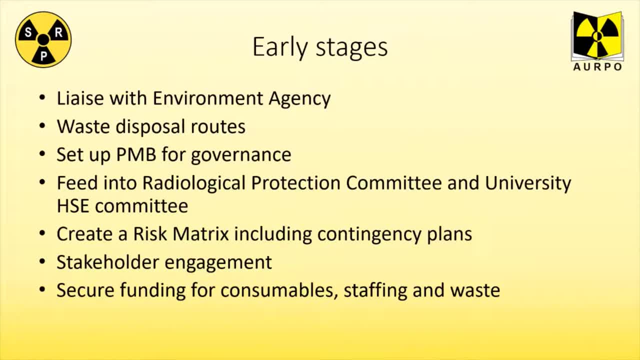 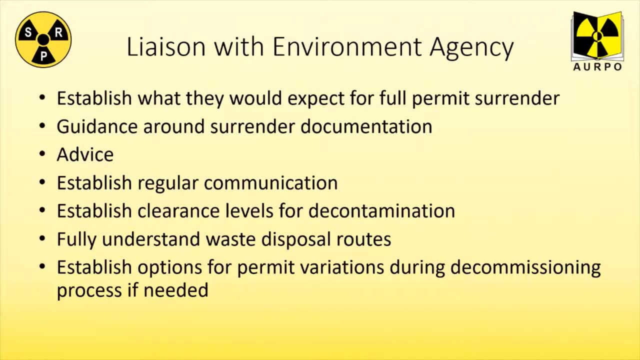 liquid scintillation vials. We've probably used thousands of liquid scintillation vials, so that's a really important thing to cost up staffing time and, of course, the waste disposal costs. So liaison with the environment agency, as I said, extremely important. We needed to know if 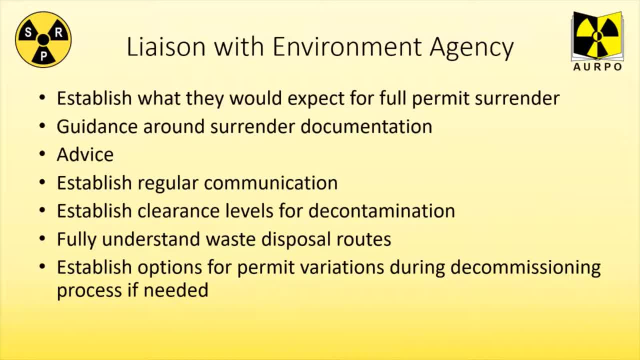 they were happy for us to do it internally. what they would expect for our full permit surrender, what they would want to see, what they would want to see evidenced. We also wanted to get guidance around the documentation. There's lots of forms you need to fill out. We wanted to be clear, right. 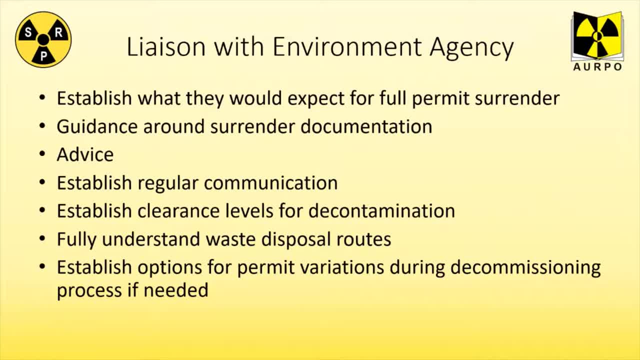 from the start what we needed to do, So we got some really good advice from them. We wanted to establish regular communication so they knew what we were doing and they were happy and they could come to us with questions or vice versa. We needed to establish clearance levels for the decontamination. 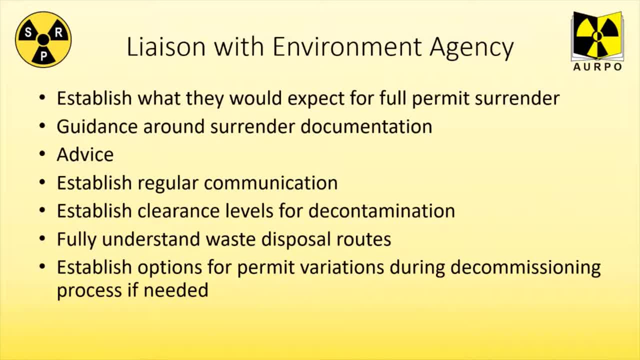 Now we've had it easier than some places because we decided we would go for we would not leave any radioactivity there, so we would go for out of scope We would dispose of or decontaminate. Now we might need to readdress that if we'd actually found something that we couldn't deal. 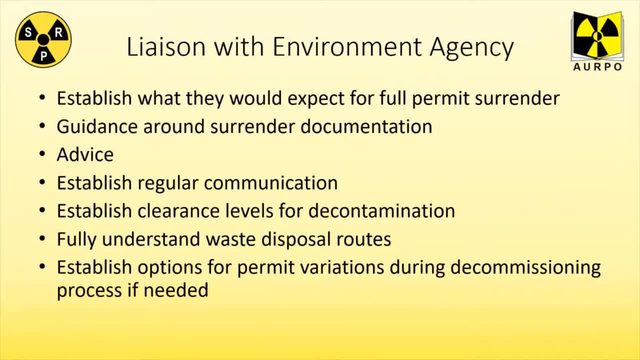 with. but that was our starting point. We wanted to discuss with them our waste disposal routes, which I'll talk to you about in a moment, and also the process if we needed to permit vary our permit if we found some problems with something we needed to deal with. 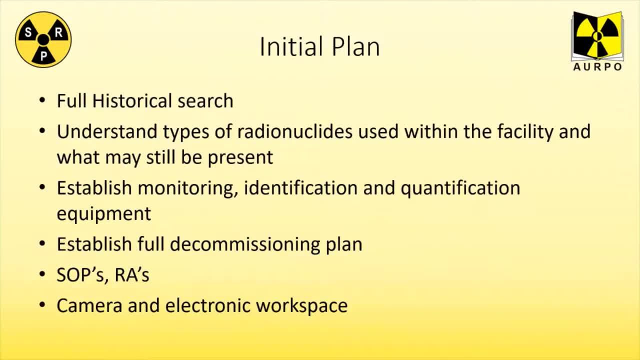 So from that we decided we'd have our. we created our initial plan. We do a full historical search, understand the types of radio radio nuclear as we've used within the facility over the 60 year period and what may still be present in. 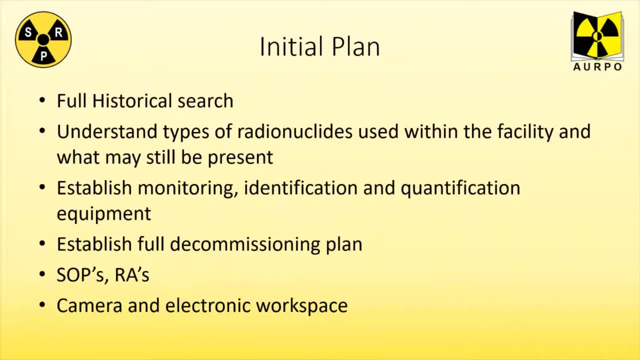 our drains and extraction. Establish the monitoring, identification and quantification equipment that we would need and the processes around that- A full decommissioning plan. write the assets so the standard operating procedures and RAs risk assessments, and do little things like make sure we had electronic workspace where we could put all. 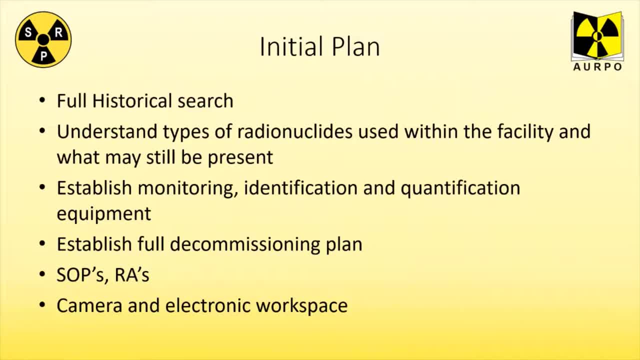 the data. Buy a camera. you need to take photographs of everything, so we bought a high quality camera where we can do this. So that's what we've done. So that's what we've done. So that's what we've done. 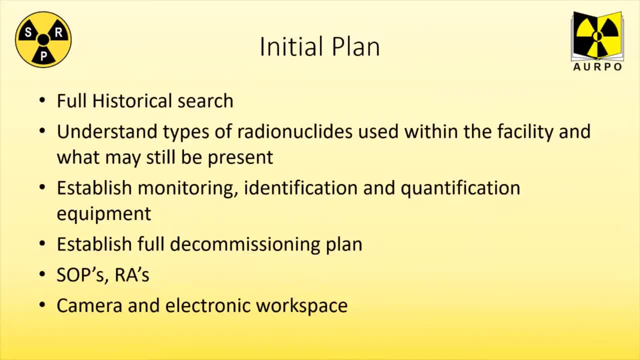 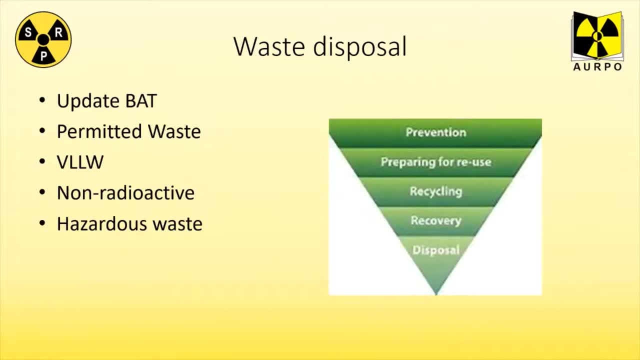 So the first thing we did is we looked at the waste disposal. We updated our best available technique, the BAT, to make sure it incorporated what we wanted to achieve through the decommissioning, And we wanted a process where where we could reuse the equipment. 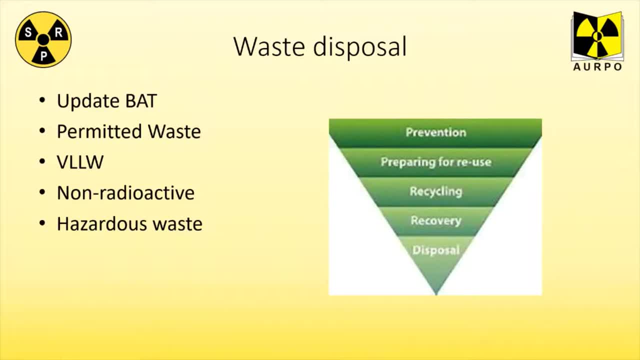 we could decontaminate it and take it out and reuse it in other areas- Glassware, for example, was checked and decontaminated and if it was clean it could be donated to local secondary schools. So also then we'd want to recycle where we could recover and then finally use the disposal for 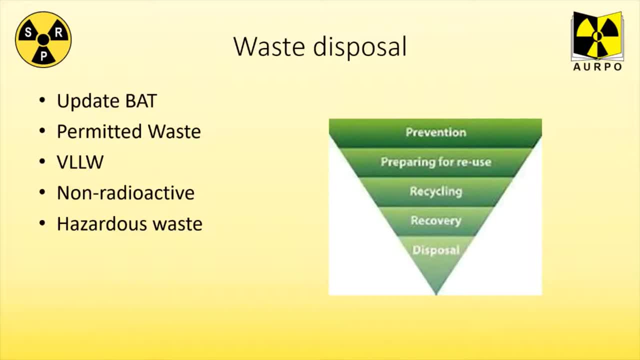 where we just couldn't do anything else. We then needed to look at our permitted waste routes. So what could we dispose of with gaseous and aqueous discharge and our solid waste routes. Also how we could use the very low level waste exemption. But then, really importantly, 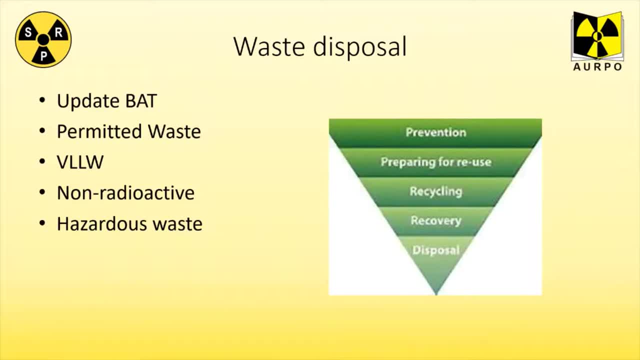 what do we do with the non-radioactive waste? Are we going to recycle that? Do we have a process? There's lots of things in that building we need to get rid of And then critically hazardous waste, chemical waste, nasty things that we need to deal with in the correct legal way. 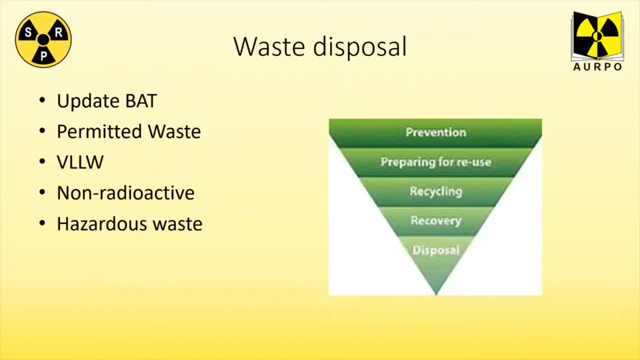 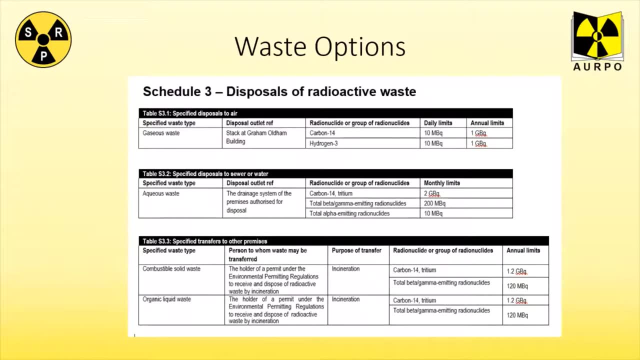 but might not be radioactive. So here are the permitted waste options: well, permitted, sorry, our permit waste options for our permit, our current permit. We've got gaseous waste. If you'll notice, it's only carbon 14 and tritium. That's the only thing that we could ever dispose of fire, gaseous waste through. 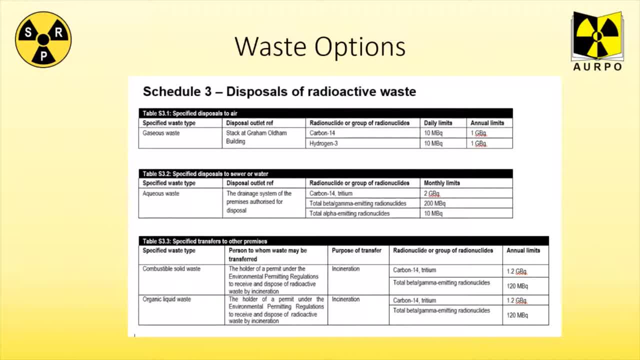 the fume hoods. Then we've got aqueous waste. We've got aqueous waste. We've got aqueous waste Which was split into carbon 14 and tritium, Another group which is beta and gamma emitters, and another which was alpha emitted radionuclides. So, importantly, we had alpha emitting on our 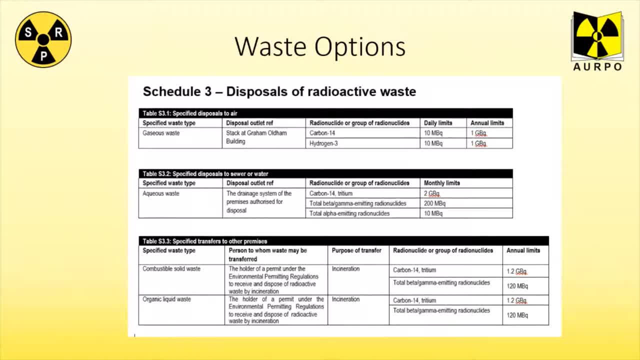 aqueous disposal waste routes and we had quite a good capacity for beta and gamma. Then we also had liquid scintillation and solid waste routes which go to a specialised waste contractor. So we were, we had faith that we had some really good permitted limits, that 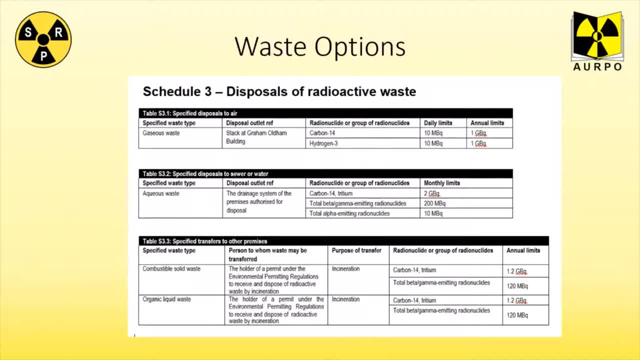 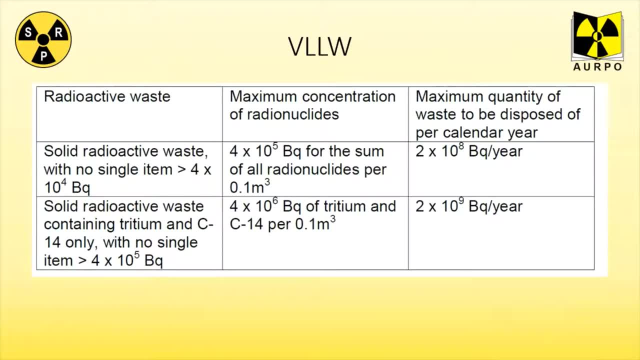 did not need changing at this point. Then we had very low level waste. So, as you'll be aware, we've got very low level waste exemptions. We could dispose of 40 kilo becquerels a single item or up to 400 kilo becquerels per 0.1 meter squared cube. sorry, 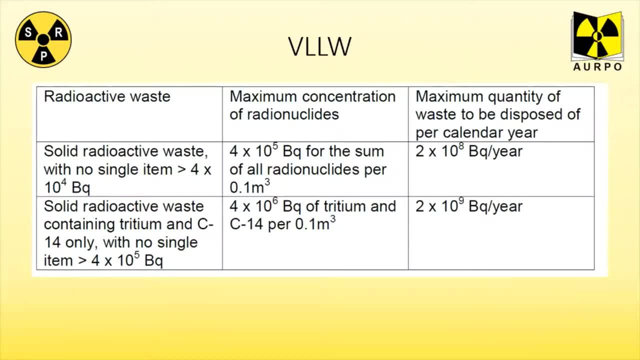 And or tritium. obviously 400 kilo becquerels And there's a maximum you can do per year. but that doesn't explain all about very low level waste. You have to be really careful that you consider things like the concentration of activity measured before you mix it with other. 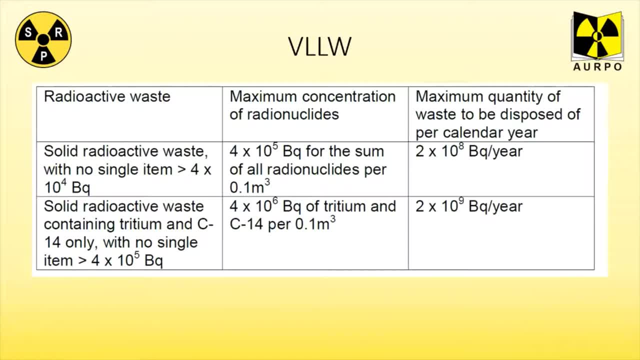 waste. How are you going to add it into non-radioactive waste? You have to consider the on the right hand side there you see you've got maximum limits. You need to make sure that you don't mix it with permitted waste, where you can, But also is it appropriate to go in very low. 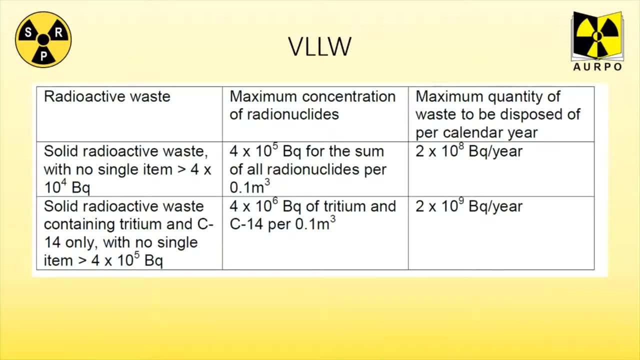 level waste? Is it hazardous? Is it got chemical hazards that we don't want it going in there? Is the dose rate too high? All of these things need to be considered to make sure that we only use this route when it was appropriate to do so. 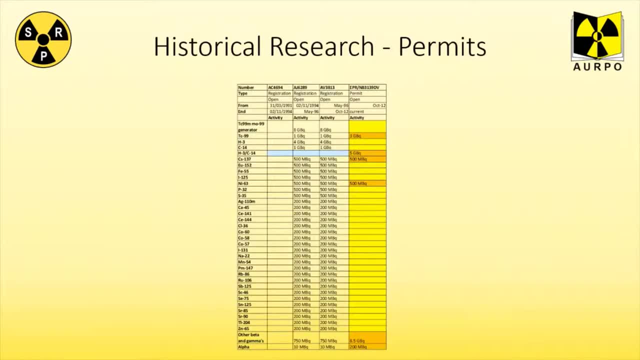 So then we looked at our permits And, if you remember, before the EPR permits came out, you have a registration for your holdings and an authorisation for your disposals. So this is our holdings And we went back to all the permits that we could find. I started in 2011,, but I had 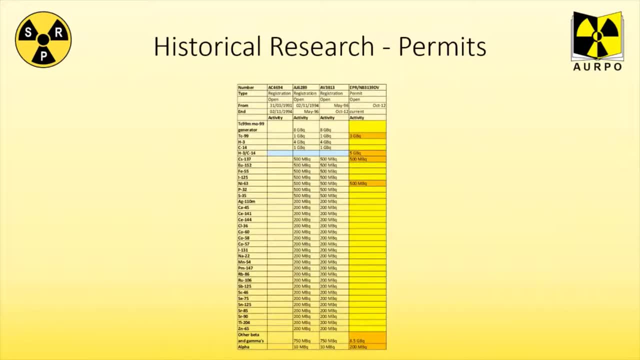 to go back and find any data that we had. We also went to the Environment Agency to see what data they had on this And, as you can see- probably unusual for university- we've used lots of different isotopes which were listed on these permits over the years. Then we've also got the 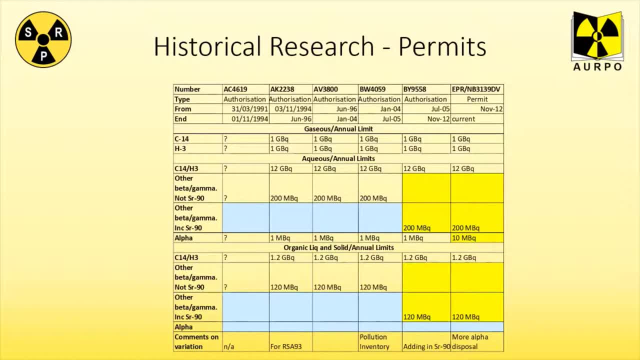 EPR permits And again that went back to roughly 1991.. And this is pretty similar, Pretty standard across the years. Strontium 90 is added in 2012.. Yeah, 2012 and sorry. 2005,, sorry. And then we had an increase in alpha emitting disposals. 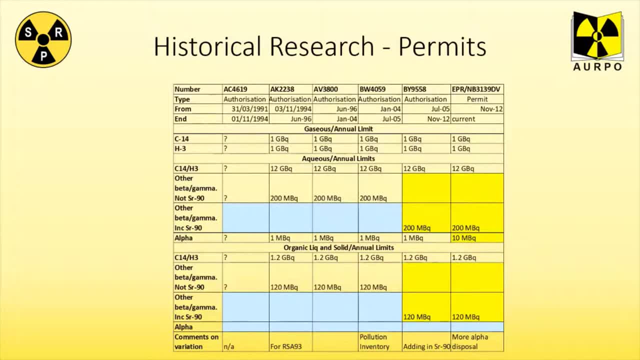 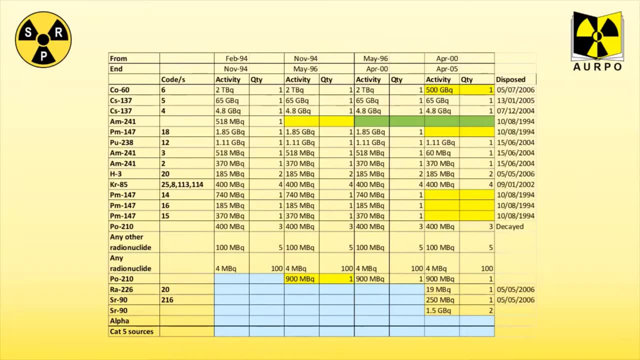 in 2012.. So pretty static. other than that, across the time, We did also look at our sealed source permits. Now I spoke to our Environment Agency inspector this week to make sure I could show you this slide, because, of course, sealed source permits are restricted. So you'll notice I've taken the permit numbers off, but I've also 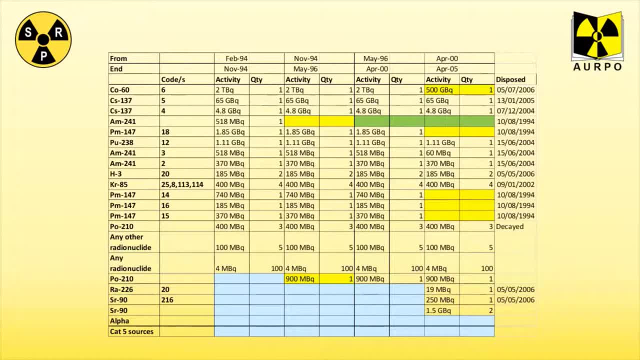 not included our most two current permits, So these are legacy permits, that we no longer have any of these sources, So that's why I'm okay to talk to you about them. And what I wanted to show you about the sealed source permit is: we wanted to be sure, if you look at all the historical permits, 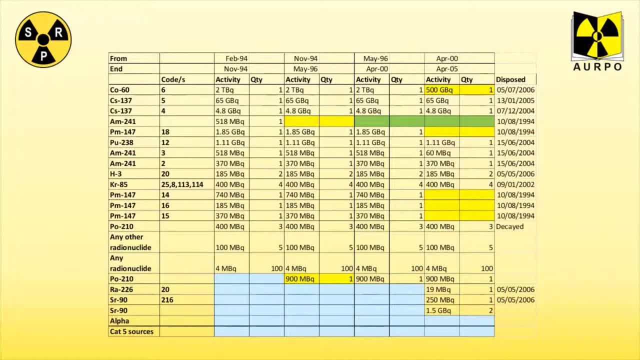 that we have disposed of these sources and we've got the evidence to prove that we've disposed of these sources. So if you see the top line, the Cobalt 60, code number six, two terabeckels originally. We know we had that through our permits In 2000, it was changed to a 500 gigabeckel. 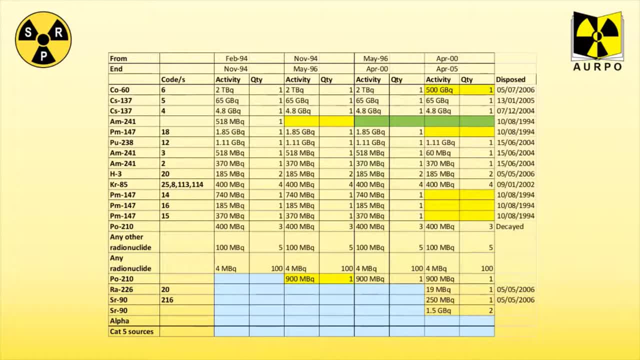 This is the Cobalt 60 radiator source, of course, And we've got the disposal date, I've got the records, I've got the sheet from the company that took it. We know that's gone And we did that for every single legacy source that we had to ensure that we have the proof and the records to show. 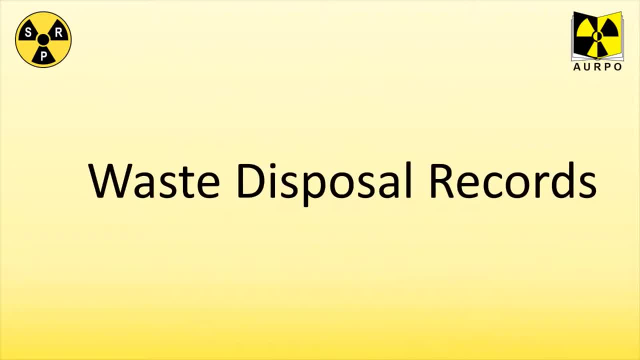 that it had been disposed of correctly. So what have we disposed of then? How do we know what's gone down our acres disposal routes? So this was a big piece of work looking at our disposal records, And we luckily had handwritten disposal records dating back to 1976.. And what I did? you've just got a snapshot here. 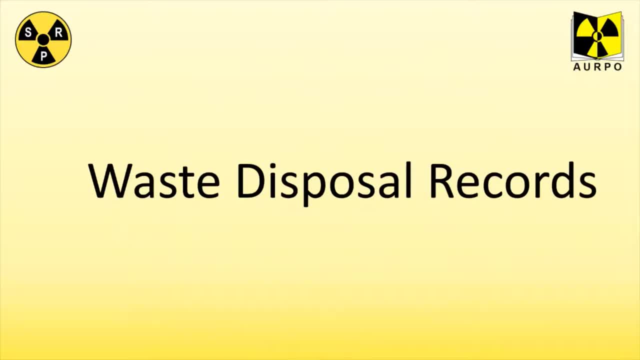 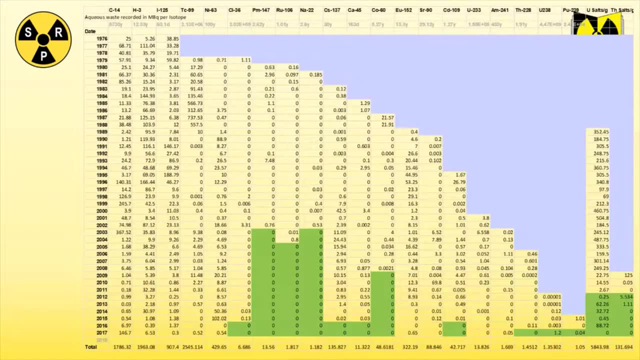 which is a very busy slide, I agree, but you don't need to worry too much. It's actually four pages, this slide of all the isotopes that have been disposed of down our acres- waste discharge. So on the left hand side you've got the dates and on the top you've got the isotopes. 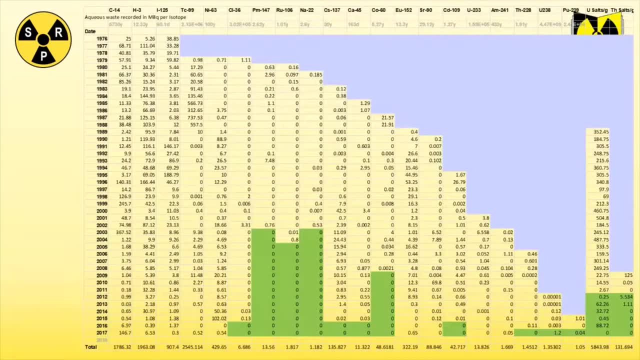 So initially we did everything. Then we removed all the short half-lives that no longer would be an issue in our drains. They would have decayed by now, So we took those out and we were left with this. As you can see, there's lots: Carbon 14, tritium iodine, right up to different types of 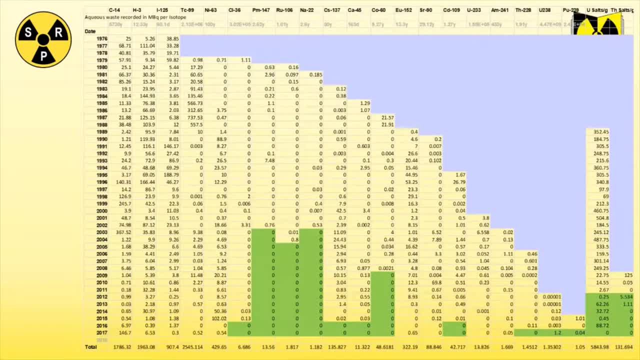 uranium. You'll notice interesting things like nickel 63 we started using in 79, and fascinating things like copper 14, tritium iodine, right up to different types of uranium, And then we started using it again in 79 and then stopped using it for ages and started using it. 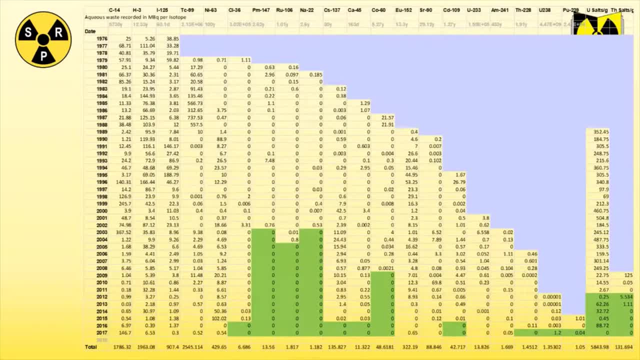 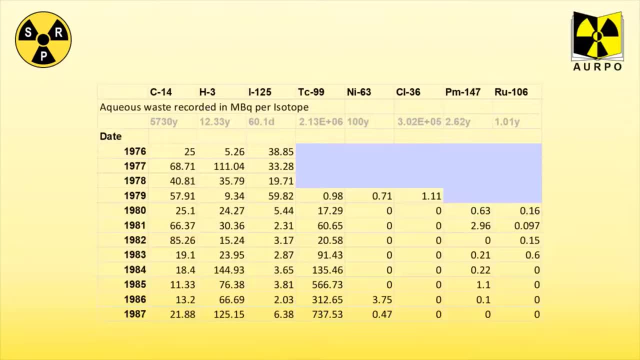 again. So there was interesting patterns of usage And if you're a radiation protection geek, it was quite interesting to see the pattern of usage across the years. And if you take a closer look- this is just zoomed into the top hand- You can see this is in mega becquerels. We weren't 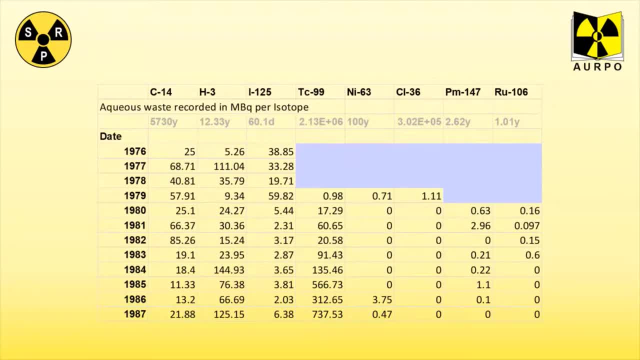 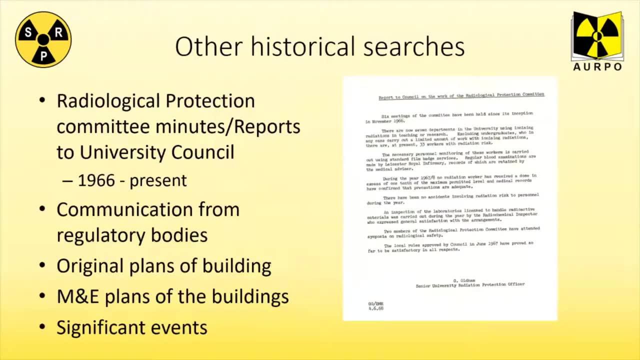 disposing of a great deal each year, even our carbon 14 and tritium. So what else did we look at? So this is a photograph of the radiation protection committee. It was actually written by Graham Oldham, our first RPO, And here you can see that they had 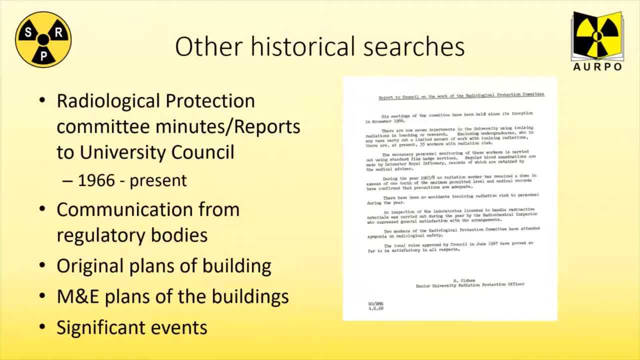 an inspection and the inspector said it was expressed their general satisfaction. It tells you how many radiation workers there were And this would provide us any information of anything interesting or anything that had happened that we might need to know about doing our decommissioning. We also have a photograph of the radiation protection committee. 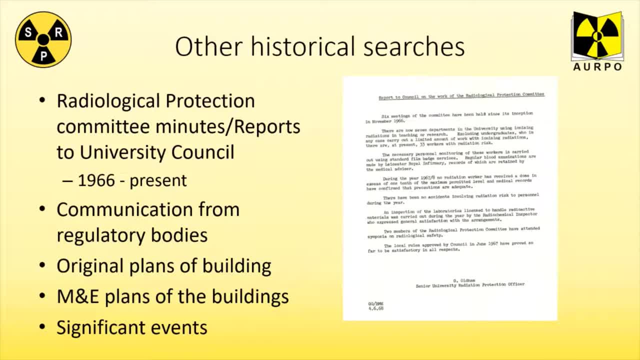 So this is a photograph of the radiation protection committee. It was actually written by Graham Oldham. We've also got communication from the regulatory bodies back to the 60s. So every time we were inspected by the HSC or the Environment Agency or whatever they were called at that time. 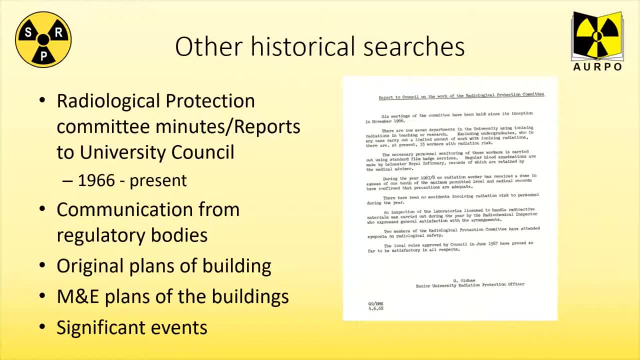 we have letters and communication from them, which is really good And again informs you of any issues they might have had with Loughborough University's use of radiation. across that time We had original plans of the building, mechanical and engineering plans of the extraction and drainage and some information on our significant events. So for 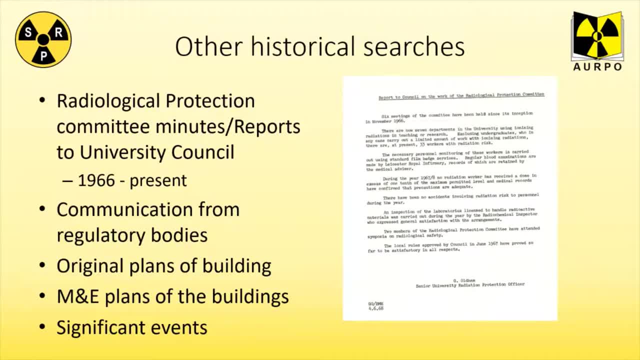 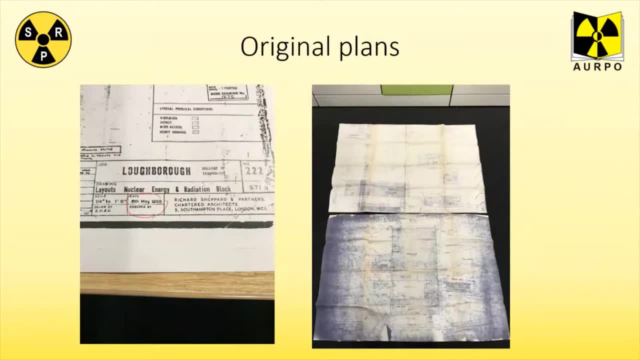 example, on the right hand side of this slide you'll see the original blueprint for the building. Very hard to see what's going on there. I've had to take it from a stall because it's A0 size, but it just shows you we've got those original plans And the one on the left is a sort 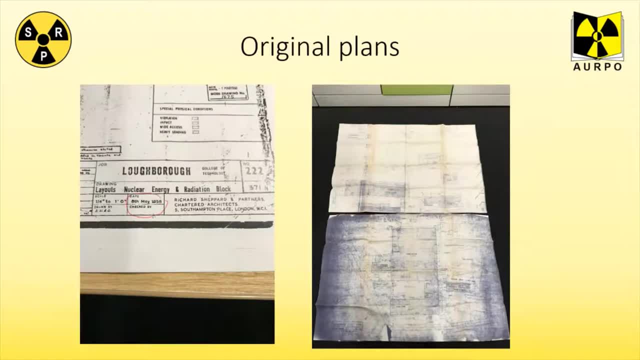 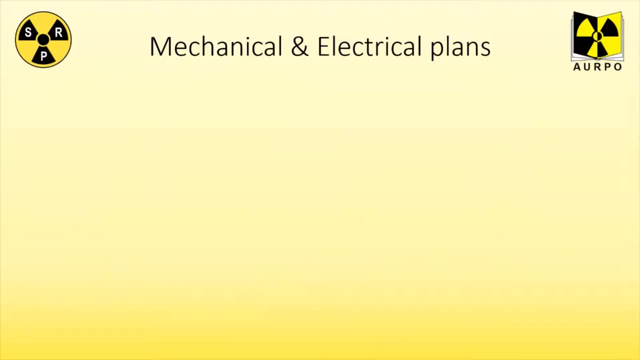 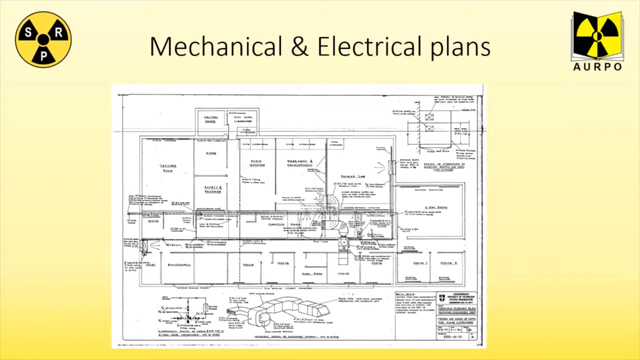 of CAD style plan from 1958. So we had really good basic plans And we also had good mechanical, electrical plans. So the first picture here is a CAD plan of the first extraction of the building, And then we have the last slide which shows you the. 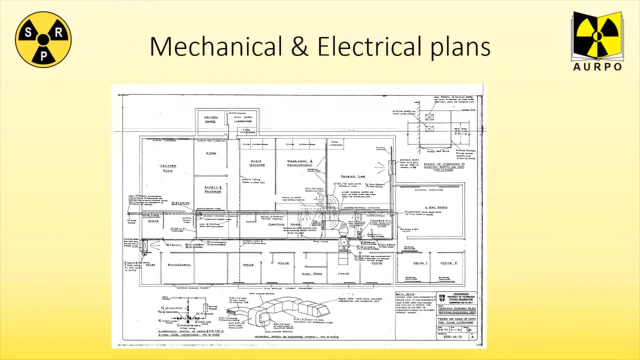 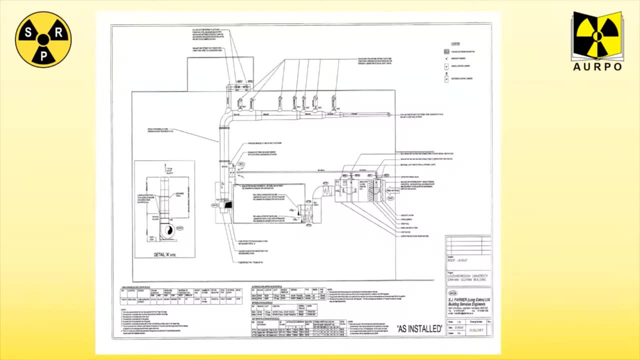 amendments and adjustments they did in the 90s, which shows you where they are. And then this later slide shows you the latest and this is the most modern extraction plan that we've got. This is what's on our roof currently, So this shows you the. 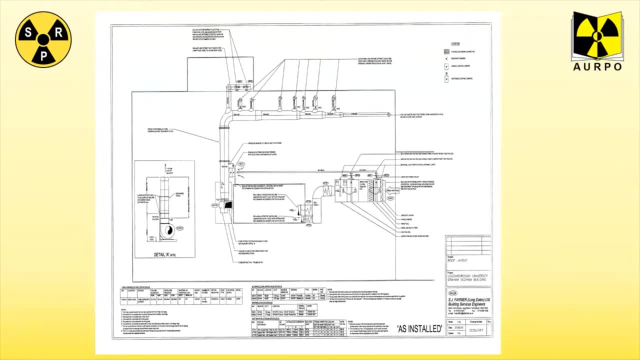 extraction coming out of our fume hoods. It shows you where the fan is and it shows you how the fresh air gets into the building. So when we're decommissioning this, we know how this extraction could be broken down and checked and monitored. So this was a really good piece of information. 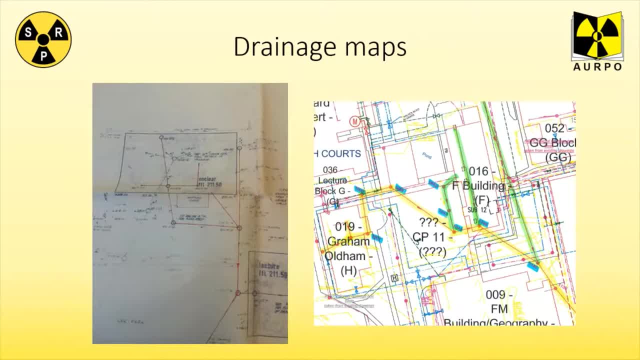 Again handwritten and drawn where the foul drain goes to from the building, And then later on we had sort of CAD style diagrams as well. So we were pretty confident that we knew where the drains were going, And later on I'll talk to you about the drainage survey and how we proved that. 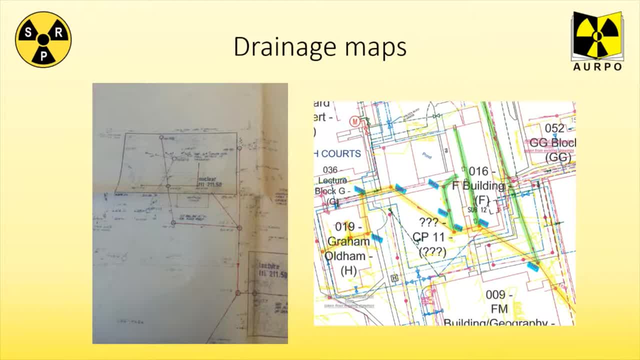 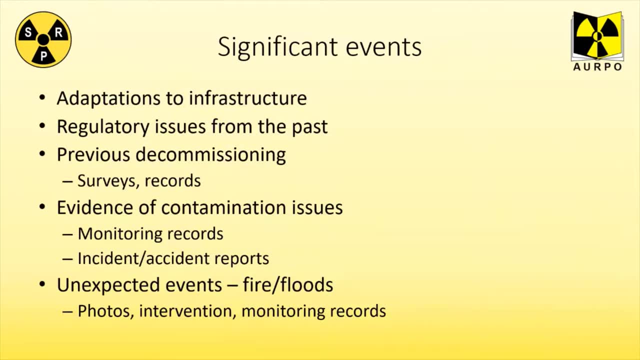 the drains were going where we expected them to be going. So we also had significant events which we mentioned from the regulatory issues that we found out, or adaptions to infrastructure, to the infrastructure. But we also had the previous decommissioning report. So when AMEC 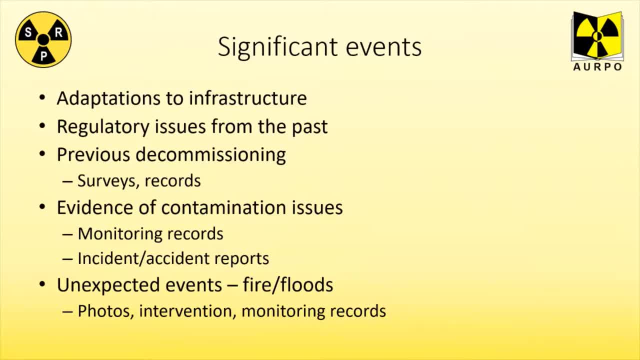 did the high activity lab in 2014,. we've got that survey records, We've got monitoring records and incident accident reports from time working in the lab, So we know if there were contamination issues and how these were dealt with. And then we've got reports on unexpected events. 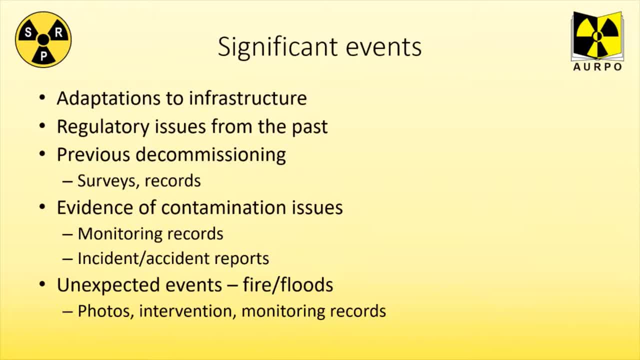 fires and floods. But what we have got is the photos, the intervention and the monitoring records to show you these were dealt with correctly. So one of the surprises that I found, they had a fire in October 1983. And here you've got sort of a slide show which I found in the 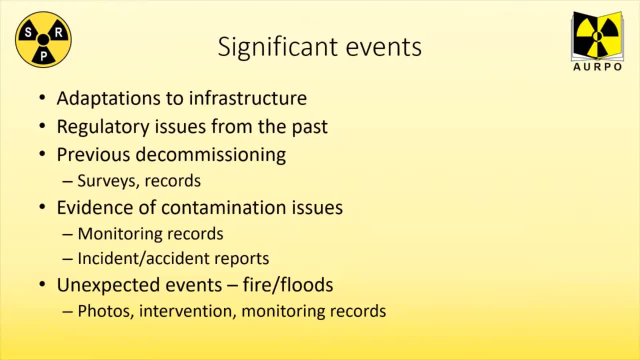 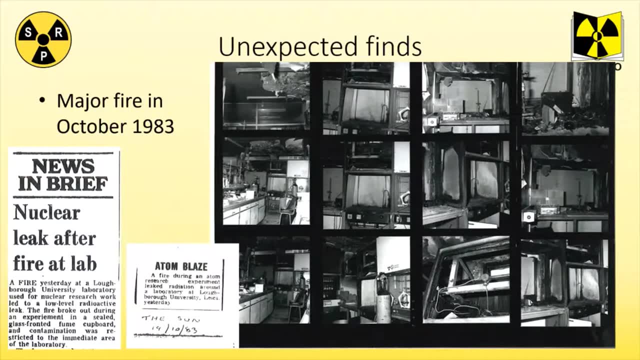 archives of the destruction it did to the lab. It was a pressure cooker in a fume hood that caught fire And they're working with Technetium 99M at the time, As you can also tell, because it was called the nuclear chemistry building. the newspapers at the time had a bit of fun with it. 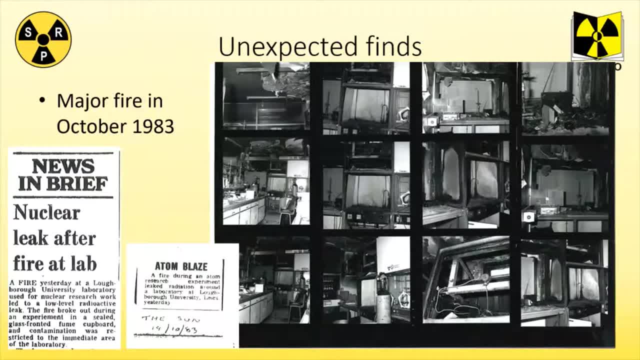 And of course said there was a nuclear leak in the lab and etc. Which I think around this time is when they decided to change the name of the lab. So we've got a lot of information about the fire. So we have the monitoring records to prove it was monitored. We have the fire brigades. 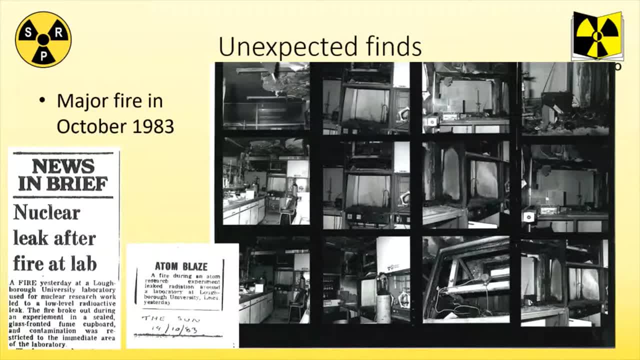 report on this. We have the regulatory bodies talking to us about this, So we had all the information to know that this fire wouldn't have left any contamination within the building. now We've had a few flooding issues. The one on the left is a storm that Loughborough University had. 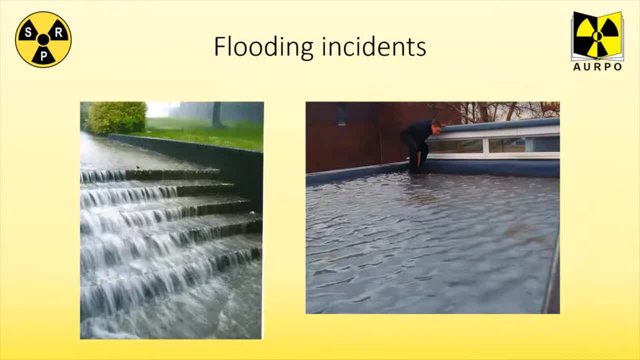 in 2012.. Most of Leicestershire had it Massive storm. Virtually every building Loughborough University had some kind of water egress in this And what we've got from the photographs and the evidence is that it didn't penetrate the. 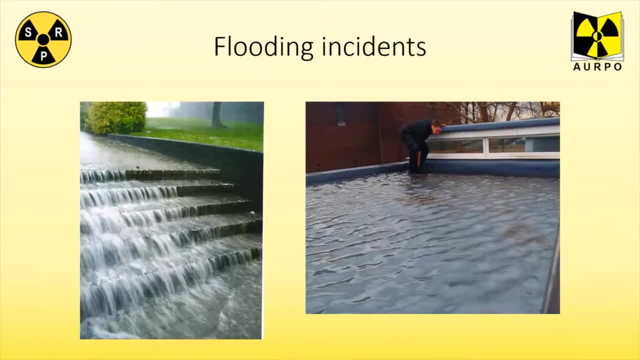 radiochemistry facility, just all the offices around it. So that was good that we had that information. We also had water dripping into our equipment room, which you've got the photographs and some monitor records. When we went up to the roof we noticed we had a paddling pool. 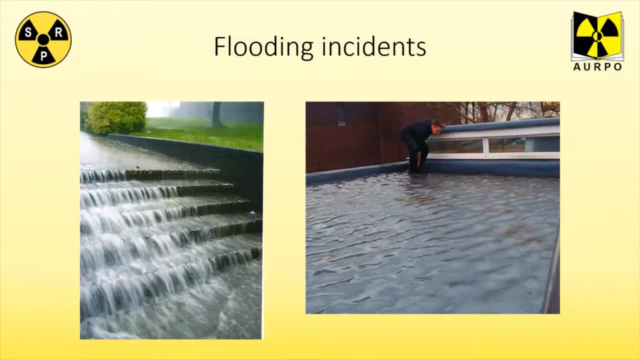 And that was because the leaves had been blocked in the drain. So the good thing is we had the photographs to show- yes, these incidents happened- but also the trail of how we showed it was safe. So that leaves us with what is still in the building that we need to be aware of. 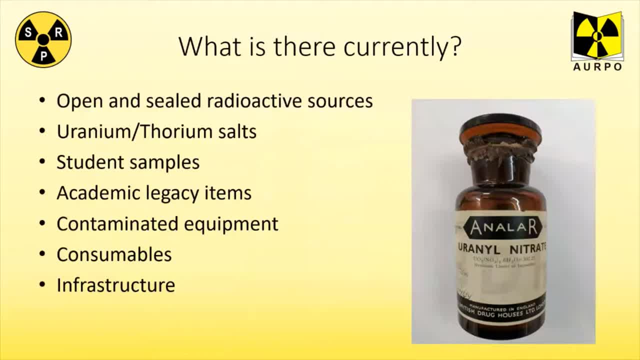 Obviously, we still got the open and sealed radioactive sources: uranium and thorium salts. This photograph shows you a source from 1939.. So that's how some of our uranium nitrate stocks are quite old but used for a very long time. We had academic legacy items. where the academics left, We still had some of their items And student. 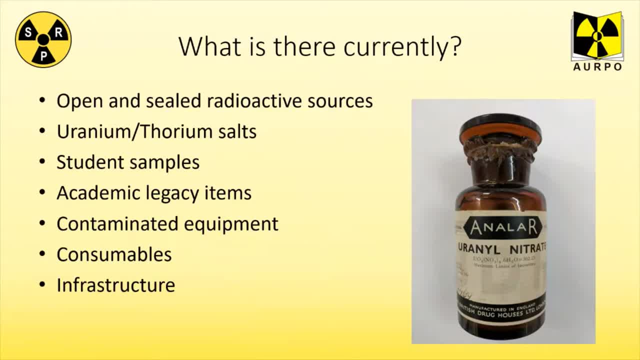 samples, students who'd left or gone, with the academics- we still had some of their samples- And, of course, the PhD students who were still present. We had contaminated equipment that needed to be dealt with before we could get rid of it, And then we had all the consumables, the pets, 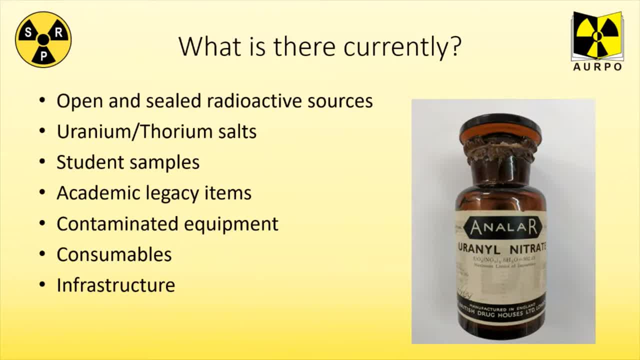 measuring jugs, bottles, you name it, we had it. And then, of course, the infrastructure itself: the benches, the sinks, the pipework, the fume hoods. So just bear with me a minute, because My slide's not moving. 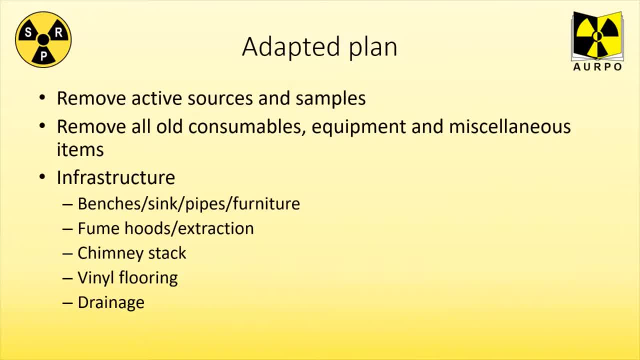 Okay. so we adapted the plan to incorporate removing all the active sources and samples and then how we're going to deal with all the infrastructure. So we wanted to create a system to know what we're going to do, how we're going to dispose of and dismantle the bench, the sink. 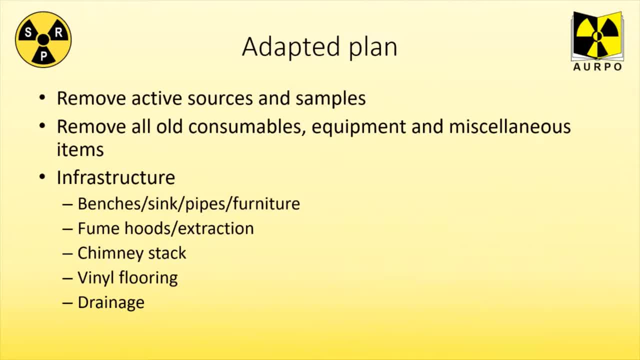 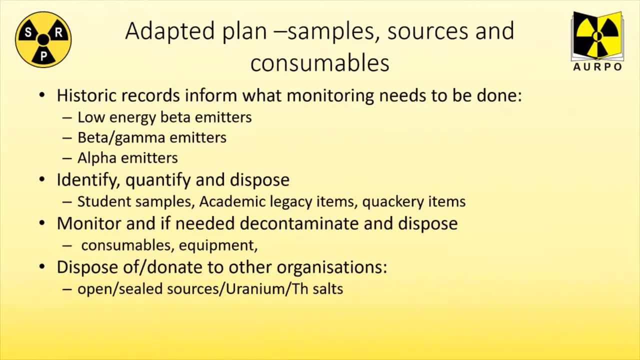 the pipes and how we're going to deal with all the equipment and the miscellaneous items. But, most importantly, now we have those historical records, we could look at what needed to be monitored. What do we need to do to ensure that we have disposed? we haven't got contamination So unfortunately, because we know we've used low? 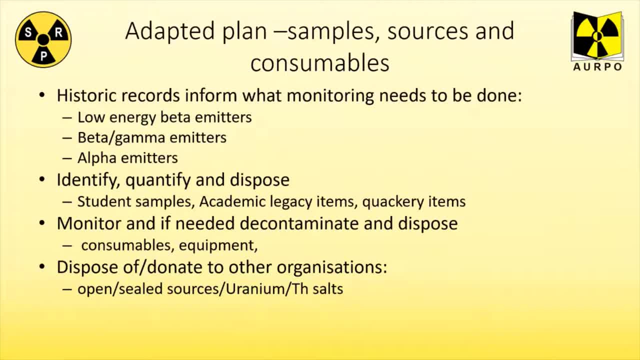 energy betas, beta gamma emitters, themselves alpha emitters. we know we need to monitor for everything, So we need to do wipe tests for those low energy betas, We need to use gamma monitors, but we also need to monitor for alphas. So we had to do everything We needed to ensure. 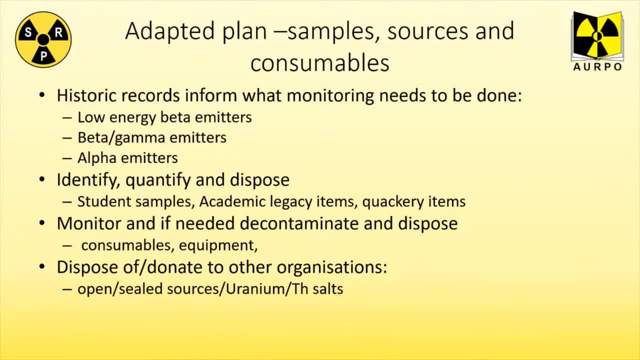 that we could identify and quantify what the student samples were, and so we could dispose of them accordingly. We also had those quackery items. Could they just be disposed of, or were they still radioactive? What do we need to do about those? We had to decide how we're. 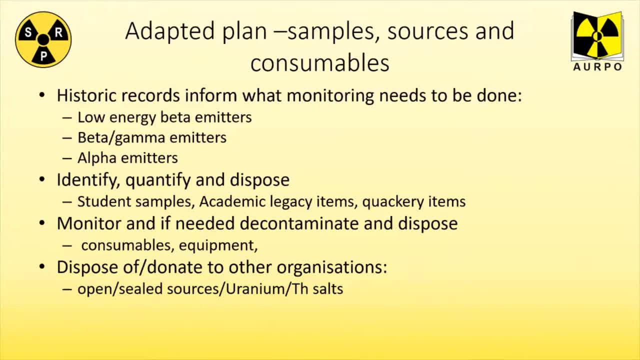 going to monitor and decontaminate and what we're going to donate to other organisations and what we could give to other places. So this very busy slide of lots of photos just kind of shows you the amount of considerable amounts we were talking about. I'm sure all who's worked in a 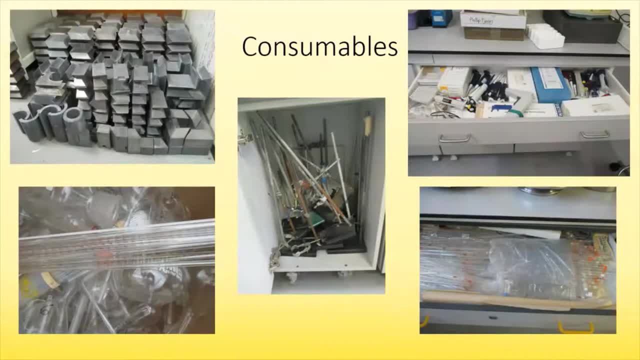 a university lab will be familiar with the cupboards we're looking at here: lots and lots of glassware, lots of pipettes, lots of retort stands. everything here had to be wiped, test and monitored, and you can imagine how long that can take. all the lead blocks that we used to protect. 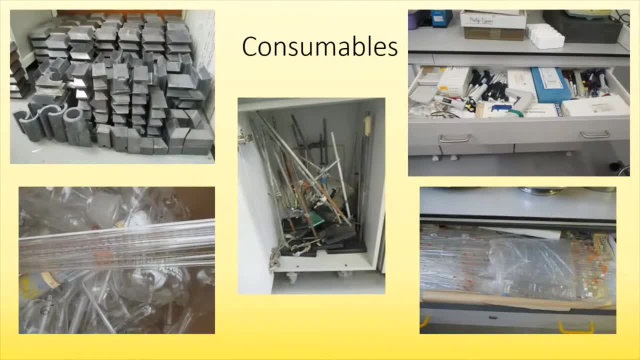 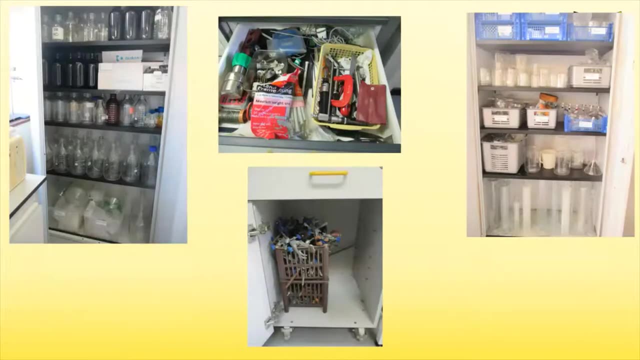 this about: the gamma emitters had to be wiped, test, checked and, if contaminated, washed with deconiety generally and retested again. everything had to be tested. and that goes through to the next section: large cupboards full of gerand, bottles, funnels, measuring cylinders, cupboards. 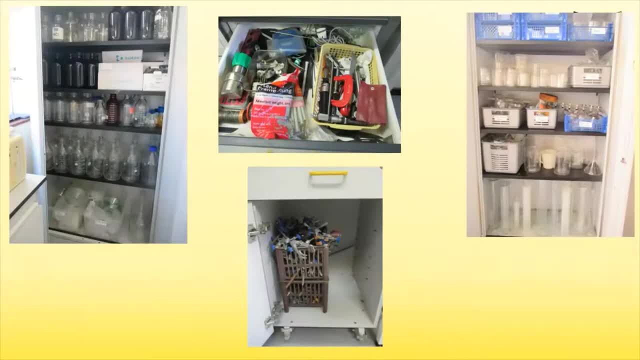 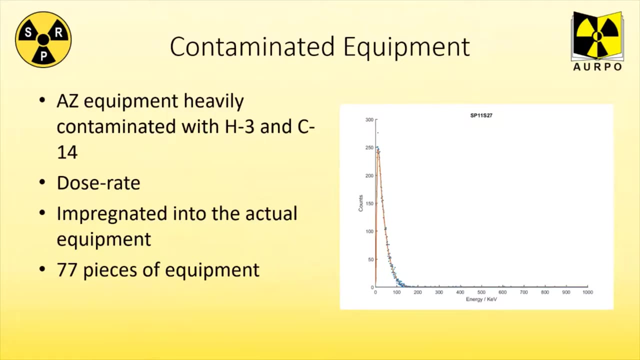 of tools. all of these things had to be checked and that was time consuming. we had a technician who was virtually just wipe testing all the time. we also had, unfortunately, contaminated equipment. so we had 77 items of equipment gifted from an ex-pharmaceutical plant in Loughborough. 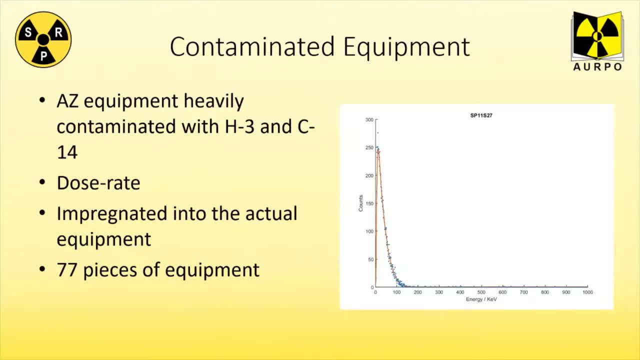 gifted from an ex-pharmaceutical plant in Loughborough, gifted to an academic, which was good because we needed the equipment at the time. but what was found is all this equipment was highly contaminated with tritium and carbon 14.. so contaminated it was. 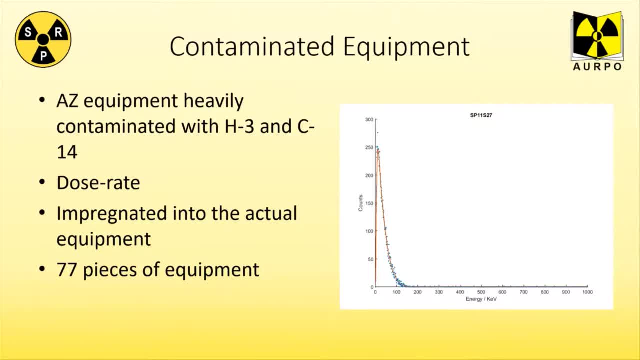 given quite high dose rates at the surface and the contamination was fixed. it was impregnated into the actual equipment. so we had a puzzle of how we were going to deal with this, because we couldn't take it for we so that's the electrical disposal route, because it was contaminated. what were we going to? 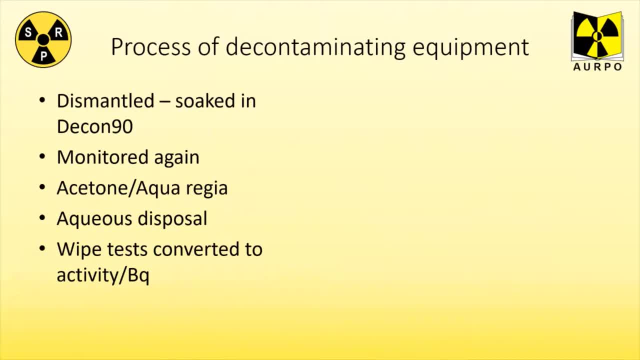 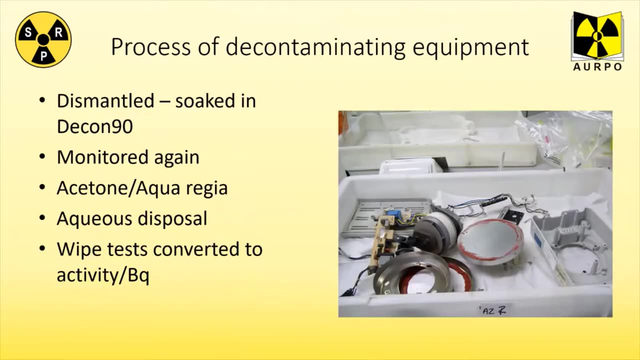 do so at the start. we would dismantle the item, and here I'm going to bring you up a picture. so this is a typical magnetic stirrer. we'd have monitored it. knowing that it's contaminated, we would dismantle it into pieces, soak it in decon 90, monitor it again. sometimes we would have to use 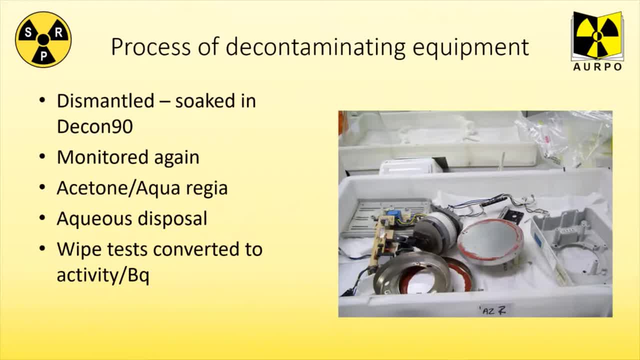 acetone to remove paint and on some occasions aqua regia, so that's nitric acid and hydrochloric acid, to actually strip off the contamination. if we use that we'd have to neutralize and then this liquid could be used as aqueous disposal. but 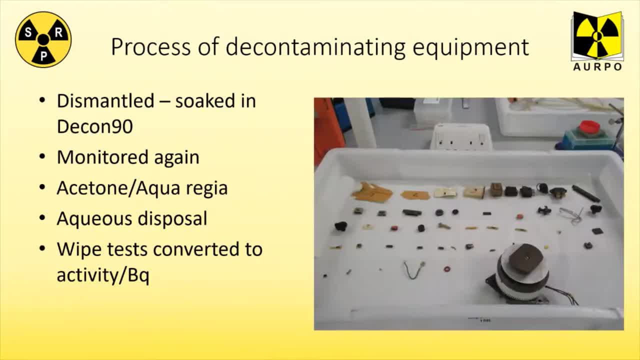 you can see from this photo, sometimes we'd have to go right down to the wiring of the equipment. it was that badly contaminated inside the equipment. the wipe test would convert to activity bird becquerel, as in the last webinar. if you joined us, I'll explain with the liquid scintillation counter. 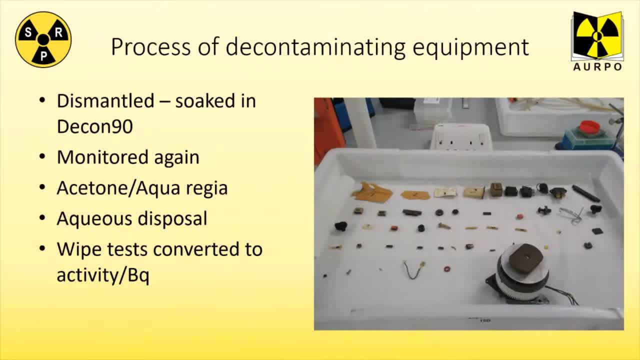 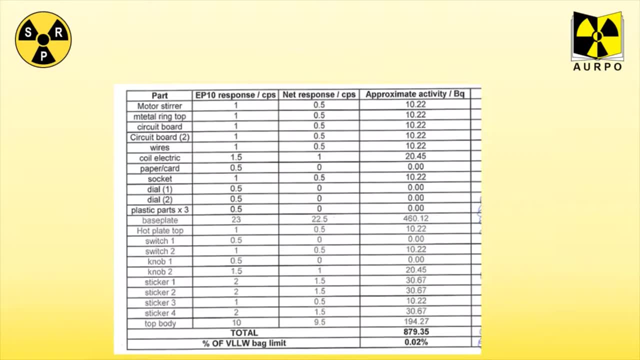 we use the most conservative efficiency for tritium rather than carbon 14, so we always over estimated the contamination rather than underestimated. and then at the end we'd always have a list like this which shows you the breakdown of the parts, the monitor response, the activity and becquerels and the total activity. so this went at very low level waste because the 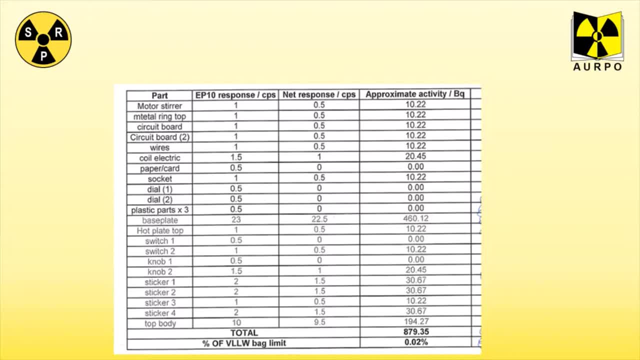 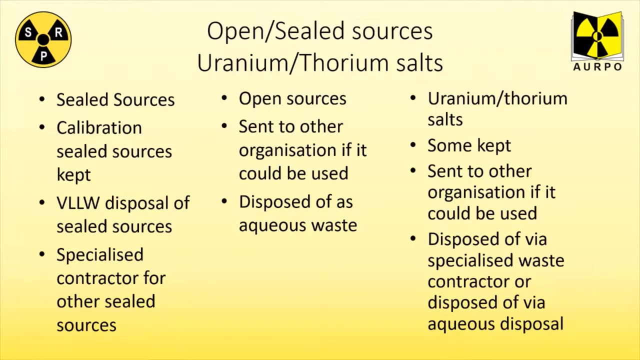 activity was less than one kilo becquerel and you see, although I've cut it off, there's my signature next to it. so I was as the rwa. I was signing off every single piece of disposal as well. then, surprisingly, the easiest things deal with were the actual radioactive sources, so the sealed sources on the left of this slide. 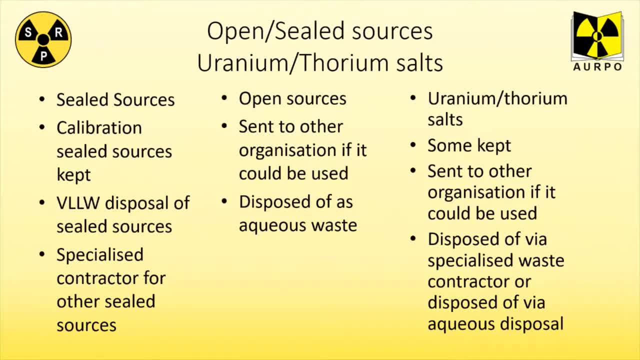 we kept the calibration sources because we need them. some sources that were only a few kilobec rules had decayed over the years, could be disposed of using the very low level waste exception. for sealed sources and others, over 185 kilobec rules had to be disposed of by a specialist. 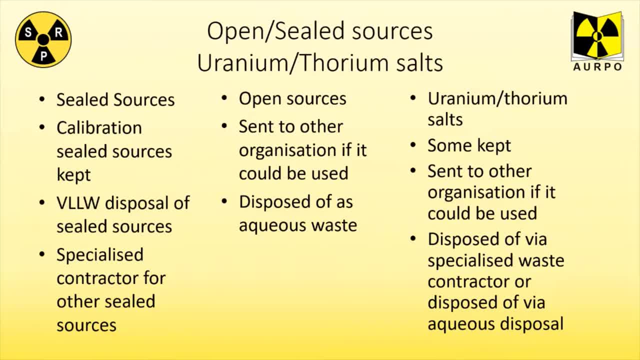 contractor and we had a couple of collections where they would come and collect those sources for us, the open sources, we didn't. by the time we started decommissioning we didn't have that many left, so with some of them we could dispose of as acus waste under our permit conditions that. 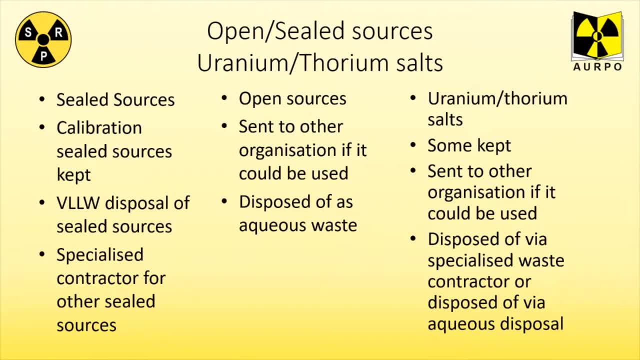 was fine and some of the other ones that particularly the expensive ones like uranium-233 and radium-226. we would donate those to other organizations if they had a need for them. uranium thorium salts: again, we kept some in case we needed some later on for electron microscopy. 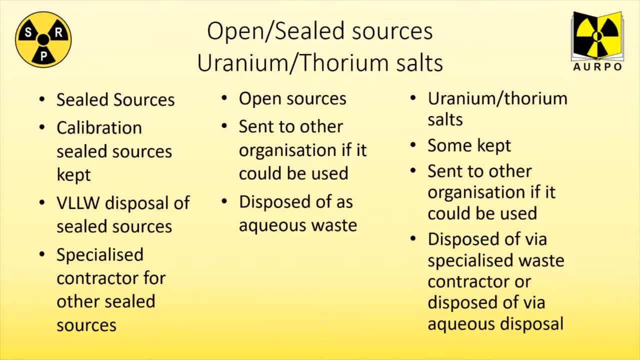 for example. others we said to organizations that might want them, and again the rest was sent, either by waste contractor etc. and we066 soch зн mk you some later on for electron microscopy, for example. others we said to organizations that might want them and again the rest was sent, either by waste contractor or. 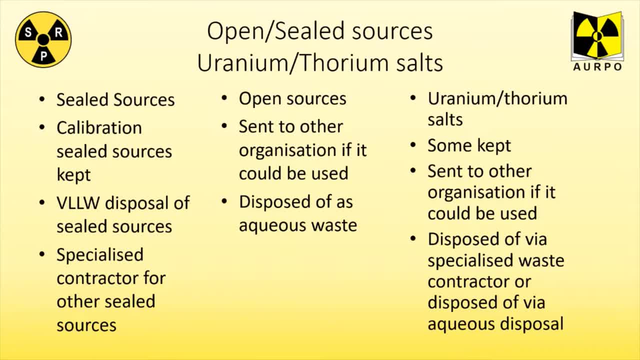 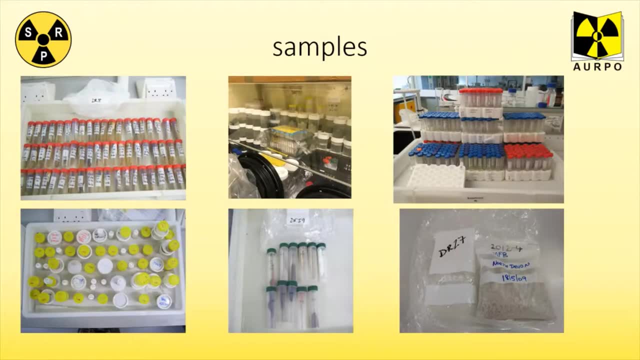 or disposed of via aqueous disposal if it was appropriate. so we had a mixture there, but these were all relatively easy compared to other areas. student samples- again not particularly problematic, but we needed to find out exactly what was in all of these tubes. so students are great. 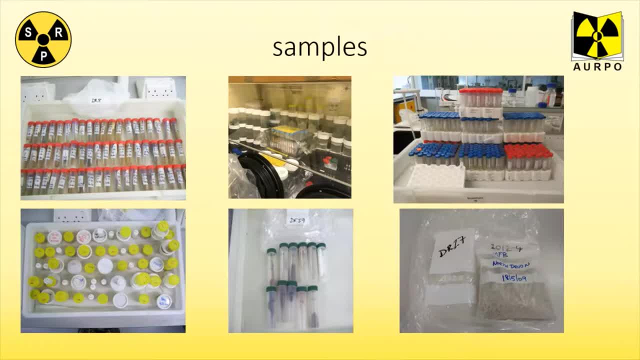 at labelling and say they've got 20 tubes and they've got 10 kilobeckels of nickel 63 in those 20 tubes. they had labels and say what was in what. but of course then those students left and us to interpret their labelling system, which proved quite difficult, so we had to individually check. 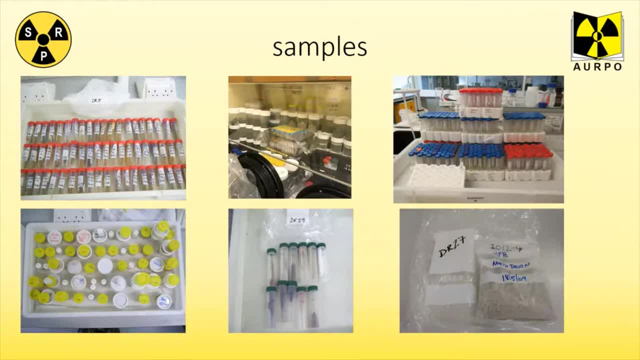 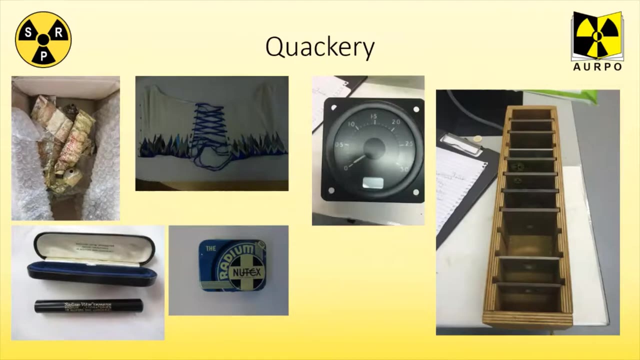 every sample to see what was in it, what needed to be done and how to dispose of it. we had lots of those samples, as you can imagine. then we also had quackery items. i'm sure we've all got these in some of our university areas- so suppository condom tubes, radioactive toothpaste, corsets. 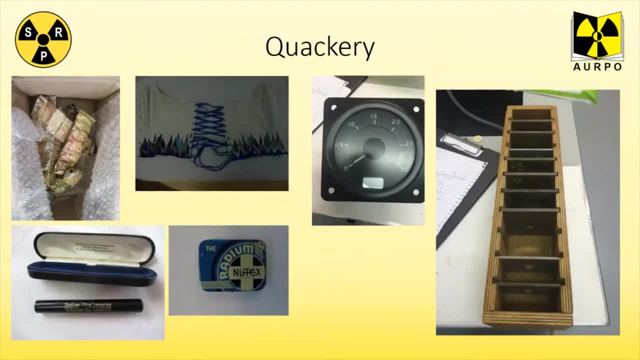 all sorts of things back scatter plates. now. a lot of these weren't radioactive and could be either donated to people who wanted them or just disposed of. the back scatter plates had to be decontaminated, and that was fairly easy, but what we did suffer from was some that were actually really very hard to dispose of. 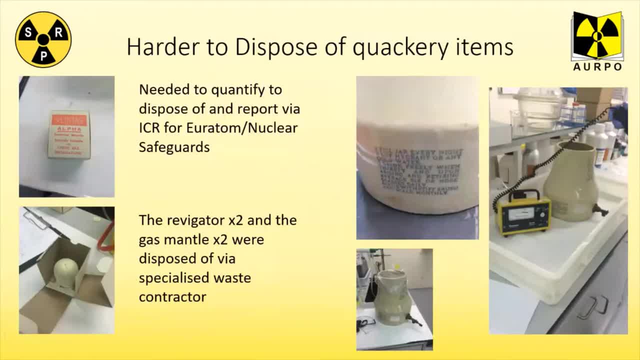 so, for example, we had gas mantles which were used in the 1900s to uh for lamps and lanterns and contained thorium- six to twelve percent weight of weight thorium in there. so for a 60 gram gas mantle you could imagine there'd be about 0.6 grams of thorium. now the problem is: 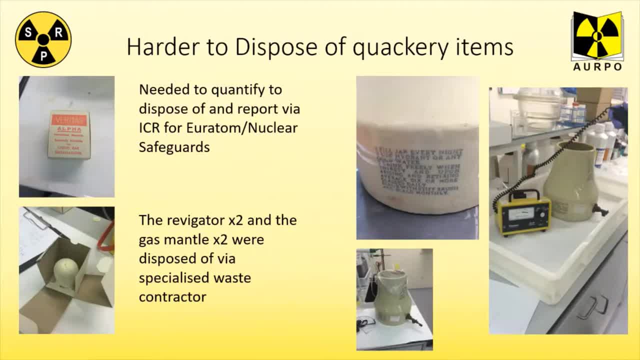 that we had to dispose of all of these. so we had to report to your atom and nuclear safeguards for all our nuclear material. so we had to report that we had these and also that we disposed of them and we had to tie that in with our specialist waste contractor. so those figures match, so that 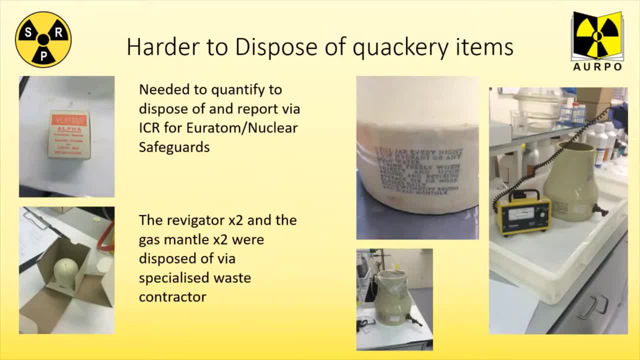 was quite expensive to dispose of this. so i would say, if you have academics who want quackery items, do consider how you will dispose of them when you need to. the other issue we had is the revigorators here on the right hand side, which is basically a ceramic pot which has been impregnated with uranium. 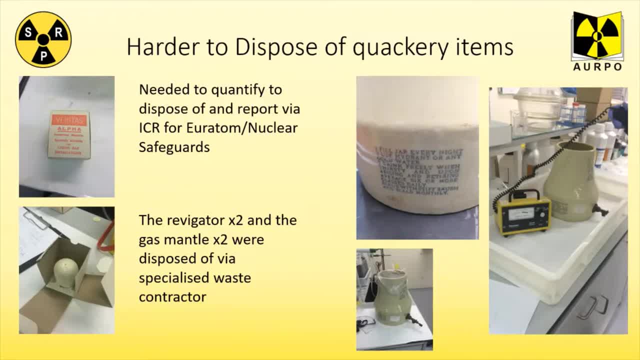 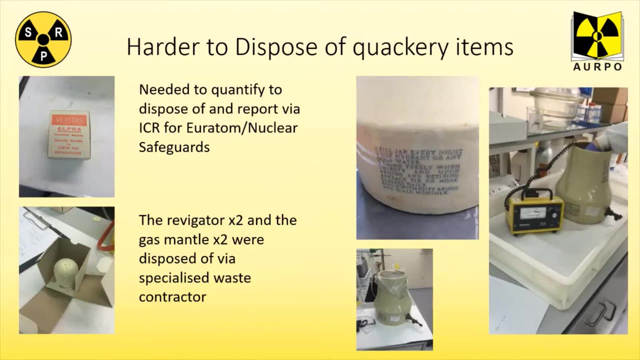 they actually give off quite a high radiation dose and and if i just click on the slide at the right, you'll see the monitor. you won't have any sound, but you'll see the monitor go up as the as it's dosed. i can hear the guy character going off. also, it gives off a lot of radon, so you. 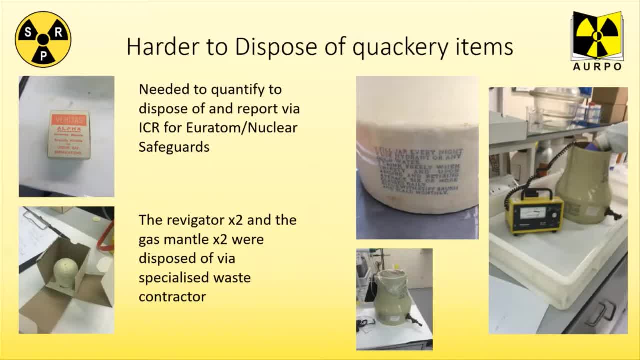 have to be careful of your work level exposure for radon with these items. we have to dispose of that. but the waste contractor and the um, you have to be needed to know how much uranium was in these products. so that was difficult to tell, so we had to weigh them. we had. 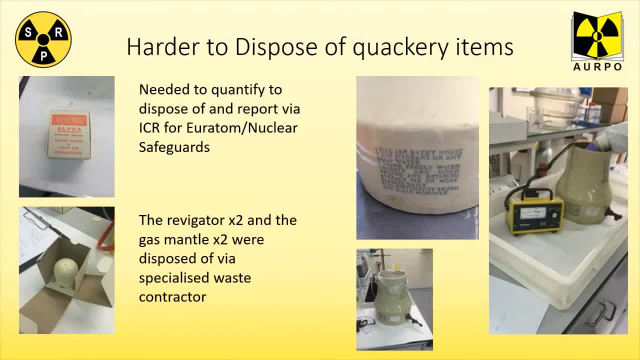 to measure them and we had to use them on the gamma spec and actually work out the activity. and it was worked out to be around 42 kilo beckles of natural uranium. so when you take in the specific activity, we could work out that each of these revaluables had 1.6 grams of natural uranium. 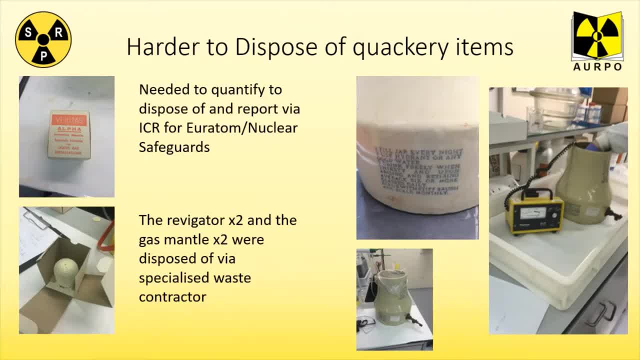 but that took a lot of effort for something that was really just there to show, to amuse the students, PVSCC, about the strange quackery items you use in a Projections available at achでも used to have. so really consider before you have any of these items in. then of course we have. 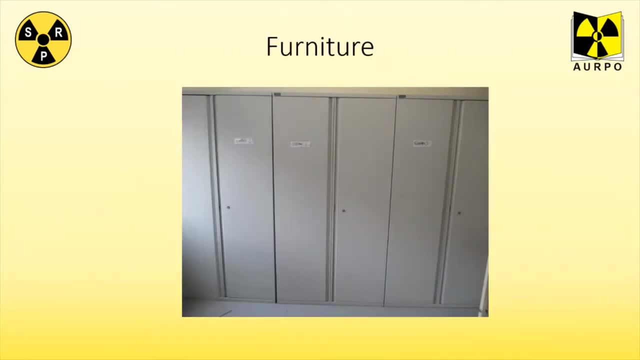 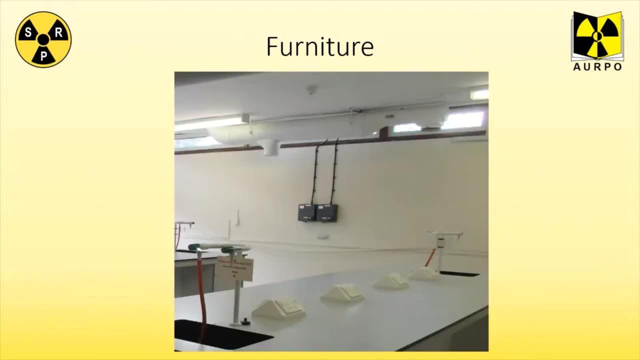 furniture, hopefully nice and easy to decontaminate and clean. unfortunately, every time we removed floor to ceiling furniture, we would have surprises. for example, we found old extraction systems which now need to be wiped, test and checked just like everything else. so that was always a little. 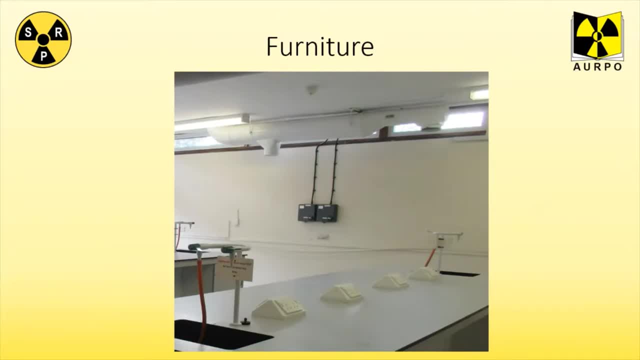 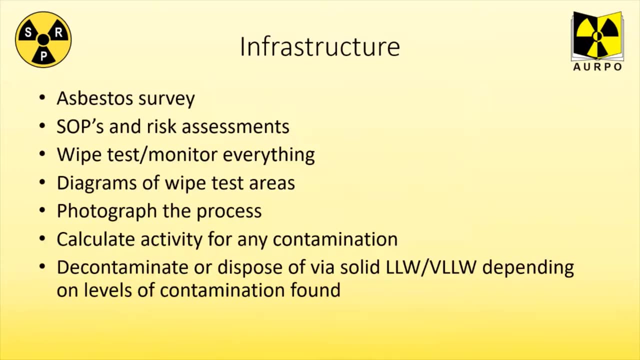 bit of a shame. so then, lastly, and this is sort of the more difficult areas, is the infrastructure. so you, I will go through the things we did automatically so I don't have to keep repeating it. we did a full demolition asbestos survey. it's very important with a building from 1958 to know. 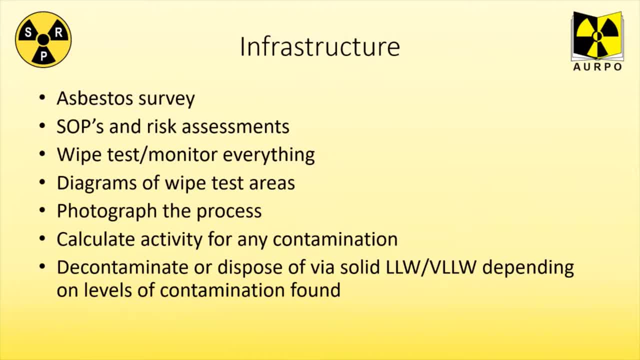 what asbestos is in that building. so we did that first really thoroughly. we had to know that we did standard operating procedures and risk assessments for every sexual, every single element. so we had one for fumes, we had one for extraction, we had one for benches, we had a policy would wipe, test and monitor everything before it left. we'd. 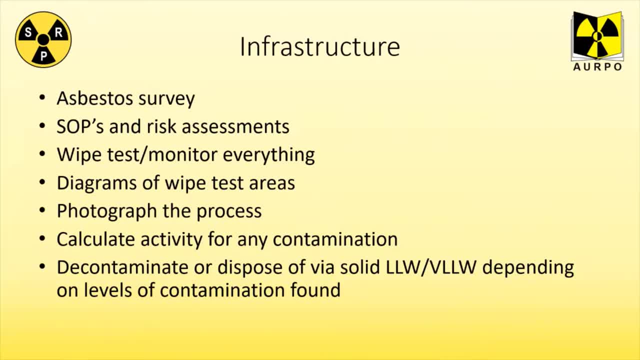 draw the diagram of the wipe test area so we could so go back if we had any areas of contamination, and we'd photograph everything. I have bored my team sensors with telling them to photograph everything. we photographed literally every single thing, but a photograph tells you so much. 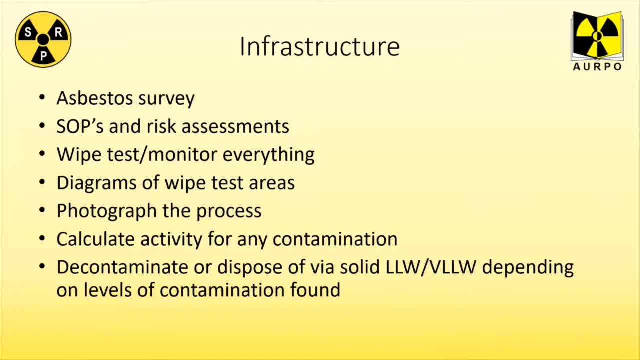 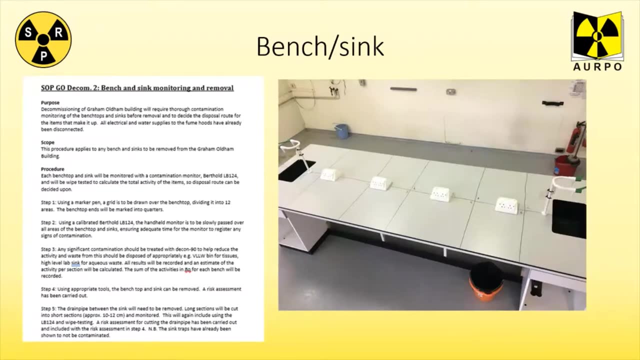 we would calculate the activity for any contamination and then decontaminate or dispose as required. so here's a, here's a SOP that we had for the bench and the little sinks in the benches. the little sinks within the benches wouldn't never supposed to be used for active. 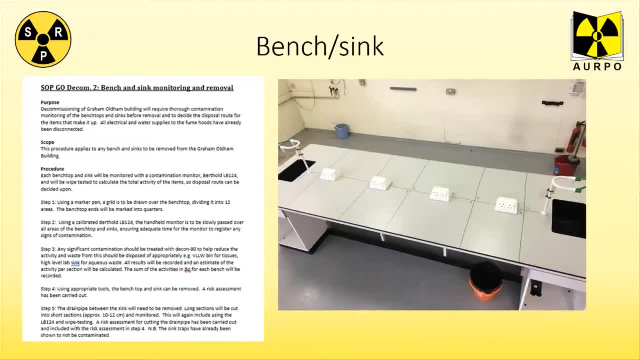 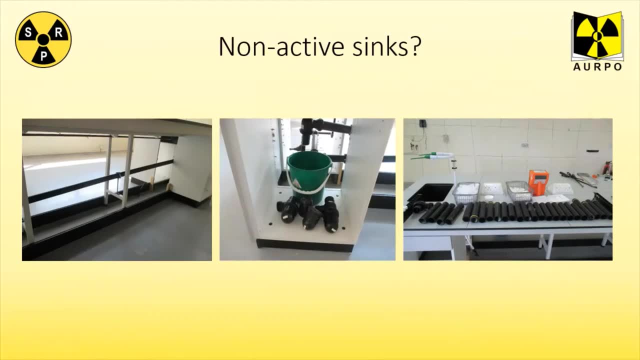 radiation. but of course we need to check to make sure. we would divide the benches up into sections so we could wipe test a monitor. we would then deal with the sink, the pipe underneath the sink, start cutting that pipework down so we could monitor every section of the pipework as you. 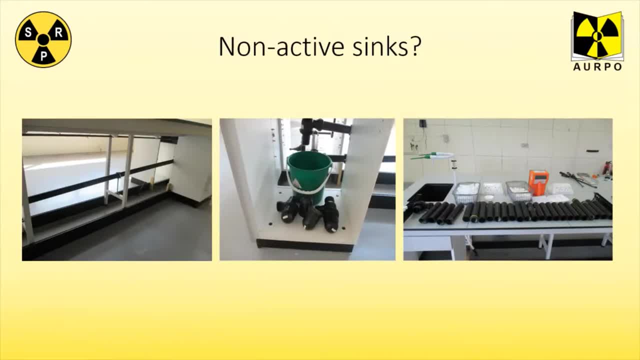 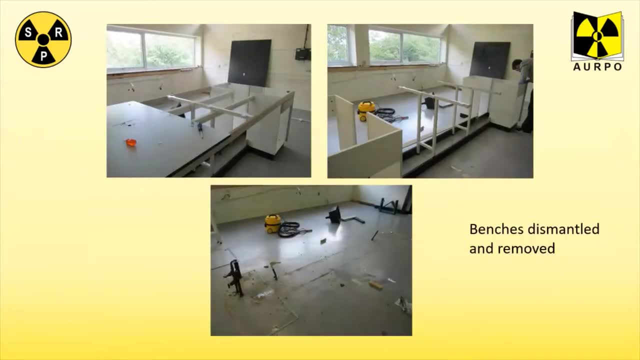 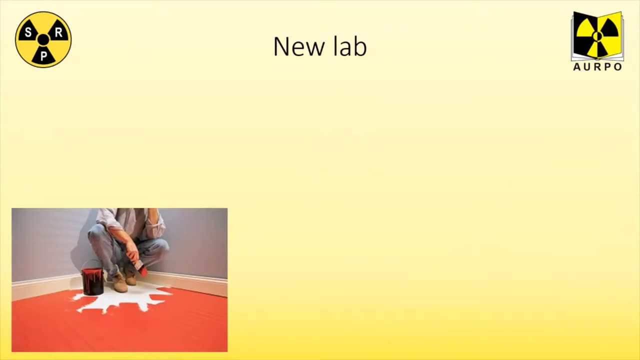 can see these diagrams. and then finally, when we knew it was ok, we'd start actually removing the benches, the trespass bench being made up. these pictures show you how it's taken down. but then we noticed we were starting to paint ourselves into a corner, because how do you test? 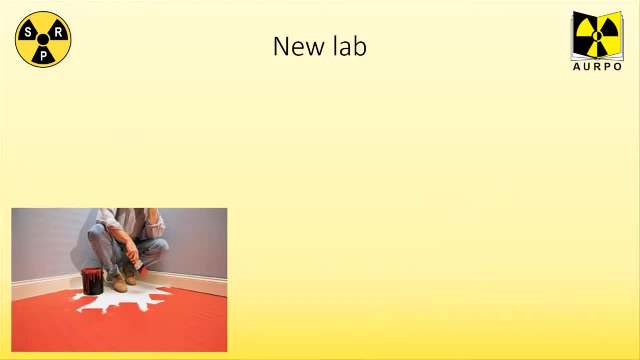 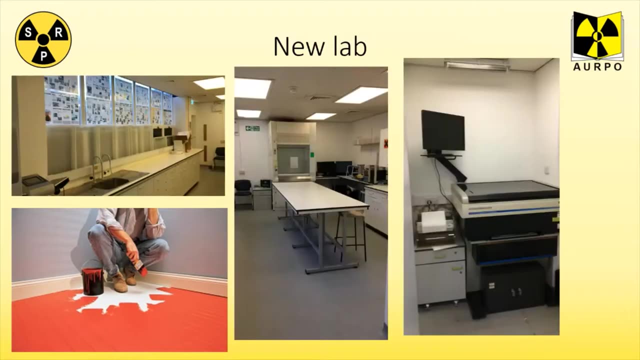 all the all the wipe tests. how do you run them through your instruments if you're trying to decommission the building? so we were luckily given a small health and safety lab, if you like, which could have our liquid scintillation counters and our gamma spec in where we could take self. 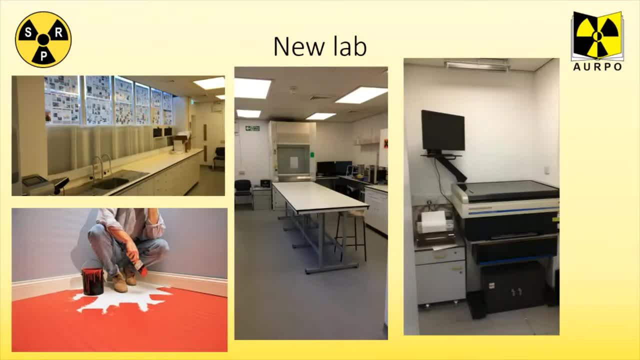 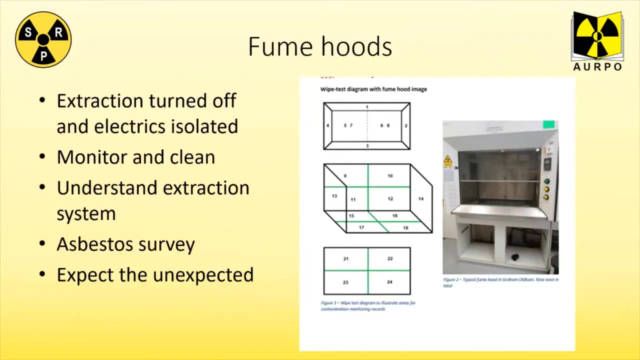 contained samples over, test them and then take them back to be disposed of. so there's no discharges in this area, but it does leave us a place to do the dry testing, which was great. so then we started with the fume hoods and, of course, the only thing that should have been up. 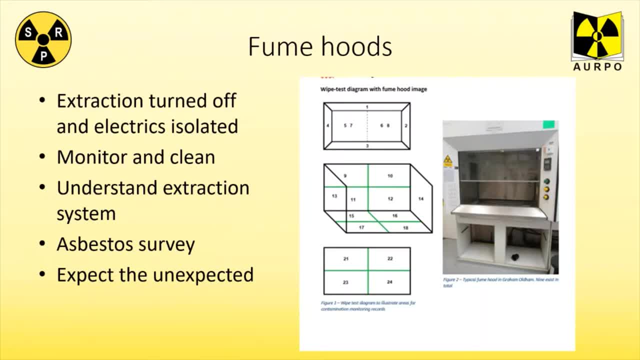 the fume hoods is tritium and carbon 14, but we did, of course, check for everything. in case you need to make sure the all the extraction is turned off, the electrics and the water are also isolated. because you need to make sure the all the extraction is turned off, the electrics and the water are also. 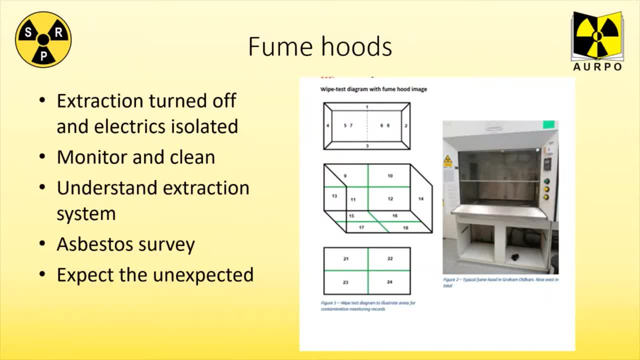 isolated because, of course, the fume hoods are plumbed into everything. you'll see on this, on the right hand side, we dye. we drew diagrams of all the areas that we wipe, tested. we had, as i mentioned, the special survey, and what we know now is to expect the unexpected, and i'll tell you about. 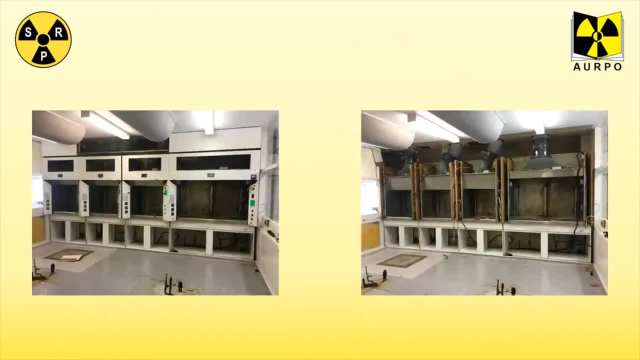 that in a moment. so here's a slide of the fume hoods started to be broken down on the left hand side. you can see we've removed the sort of the top plates. as we go further, we're removing the facings of it. you can see the wooden panels between these are quite old fume hoods, as you can tell. 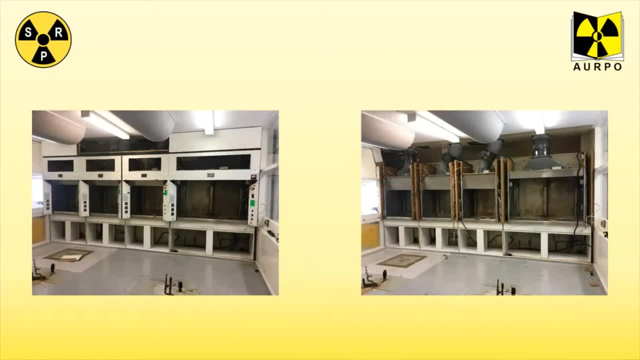 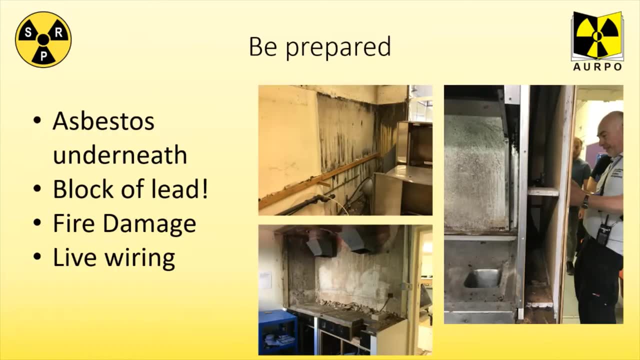 but what we did find. so what did we find that we were expecting? although we had an asbestos survey underneath the fume hood cupboards, when that was removed there were old asbestos tiles. so even though we have a demolition survey, we still found asbestos. that was fine. we had the 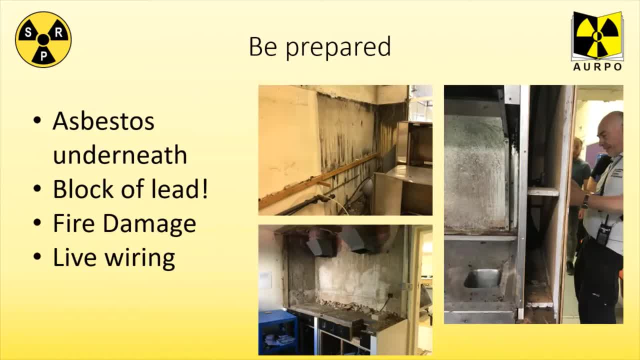 good risk assessments. that said, if you stop and notice anything, all my decommissioning staff were on how to deal with asbestos, so they knew to leave it and call in the contractors to deal with it and do the skeleton mapping and the image呢, Because we knew that in the loudest way. we knew we needed. 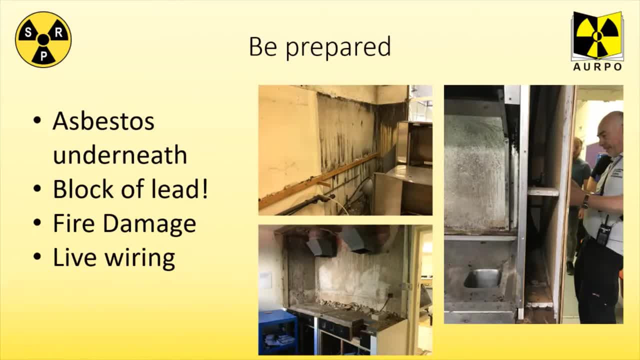 surveys- the air surveys- we also found fire damage. so if we hadn't known about the fire in 1988, now we know about it because as we removed the fume hoods we saw the fire damage left behind, which is interesting because it means in 1988 they didn't bother painting the walls after the. 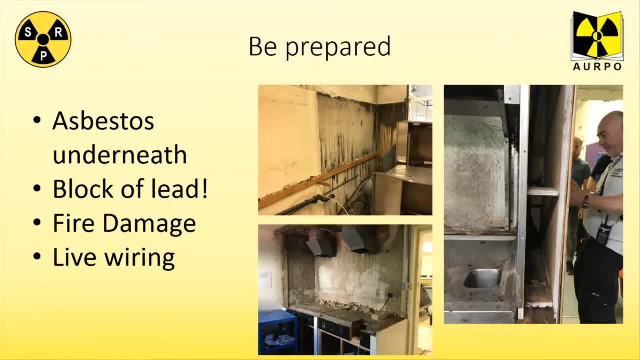 fire. we also found a block of lead at the bottom of the top part of the fume hood in our high activity lab and we would expect it to find lead in a fume hood, um, and they were really heavy to take out, so that was surprising, but the most, probably the most worrying is the live wire that 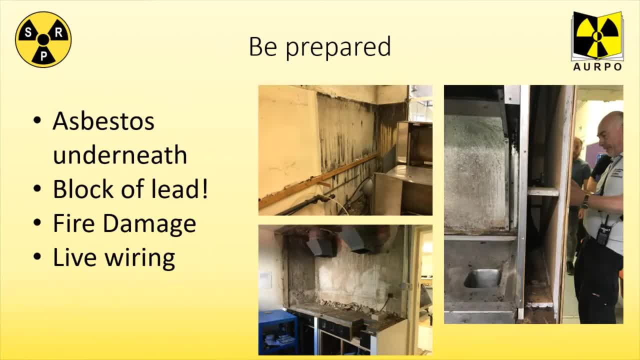 we found within one of our fume hoods. so, even though all the electrics were turned off, the electricians came over and did that as, as the decommissioning team were taking it apart, they noticed a wire that didn't look right. they called in the electricians and indeed it was live. 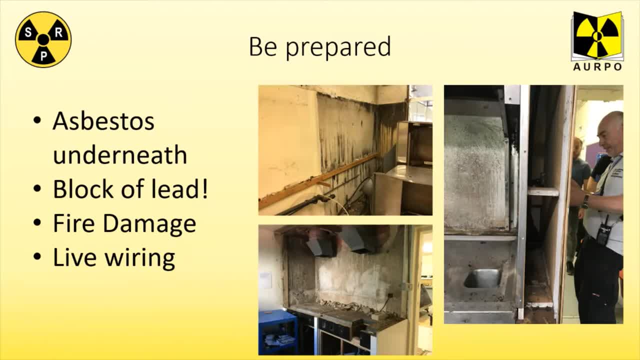 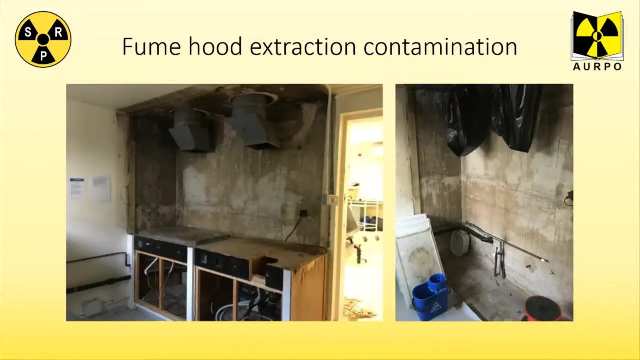 but it was from a legacy light that had been turned off- a decommission. but the wiring was buried within the fume hood so no one knew it was there. so that shows the real importance of the risk assessments and training of your fume hoods. so we did find contamination, as you kind of expect, and it was carbon 14. it was in the top. 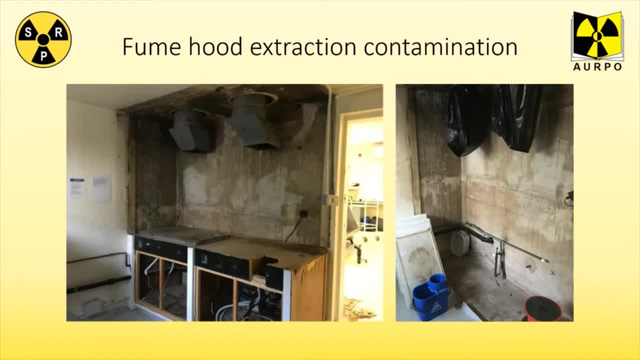 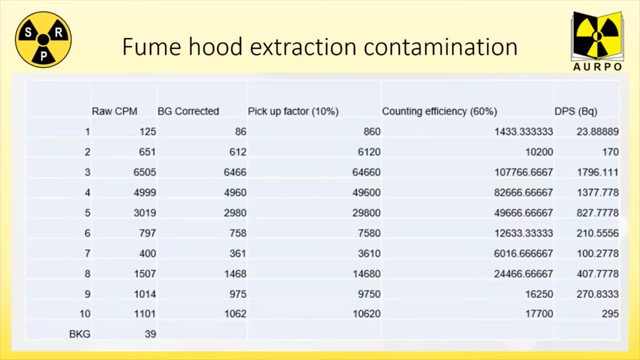 of the extraction coming into the fume hoods. so on the left hand side you can see those joints there. that's where it was. it was very low level and it was calculated, but then it was cleaned with decon 90 and completely removed. it was very easy to remove, which was 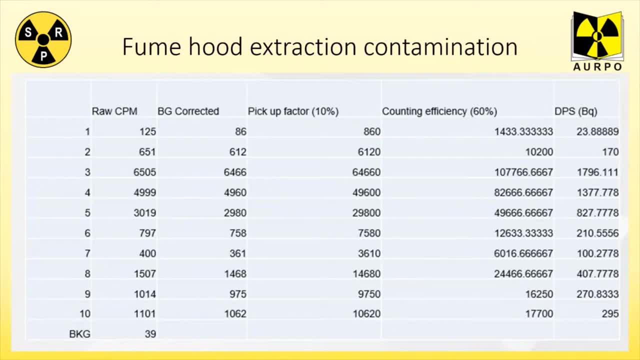 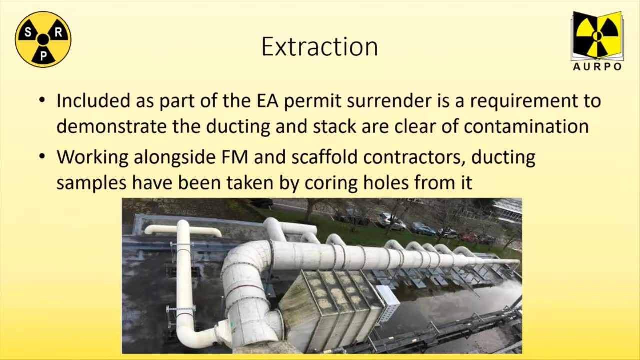 nice. so then we moved on to the roof. so this is a photo of the extraction system and if you remember that CAD plan from the start of the talk, it very much represented that we had to work with our facilities team and scaffold contractors because we've got chimney stack on there and we needed to. 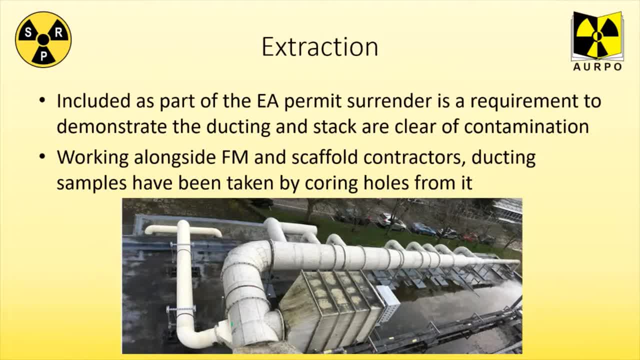 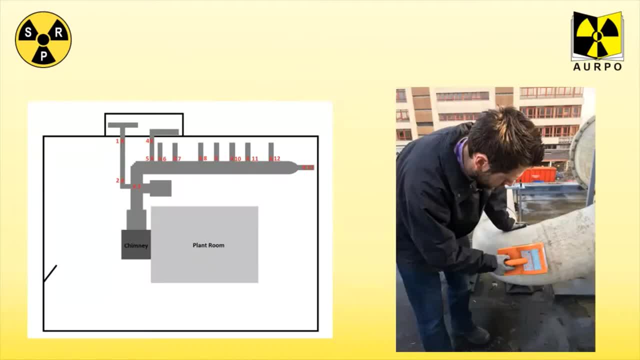 take core samples. so we had lots of extraction and lots of scaffolding put in. you'll see James- who's going to do some of the questions later- monitoring the outside of the stack, and this was a diagram that we drew showing where all the core samples were taken, so we knew exactly where. 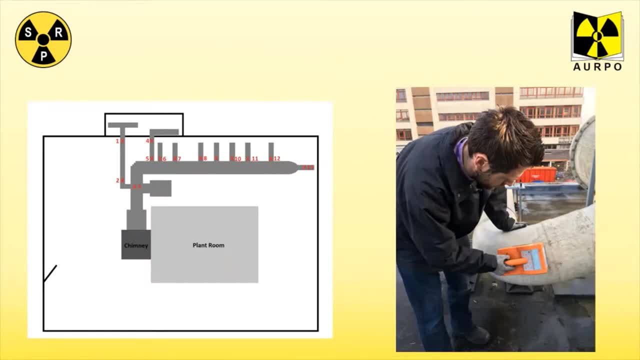 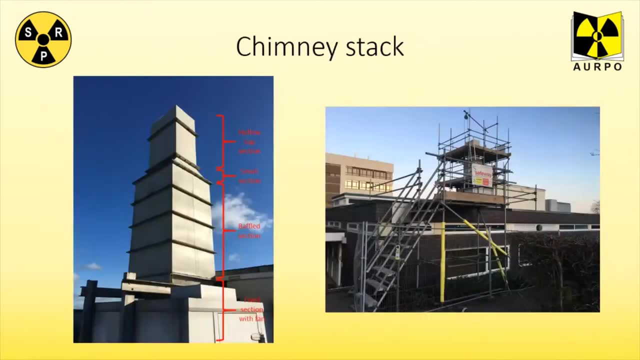 we take them all. on this slide you can see those core samples. these were all monitored and tested to make sure that we couldn't find any contamination, and then we moved on to the chimney stack. so, as mentioned, we had to have the scaffold in- and the right shows you that- and the chimney can be broken. 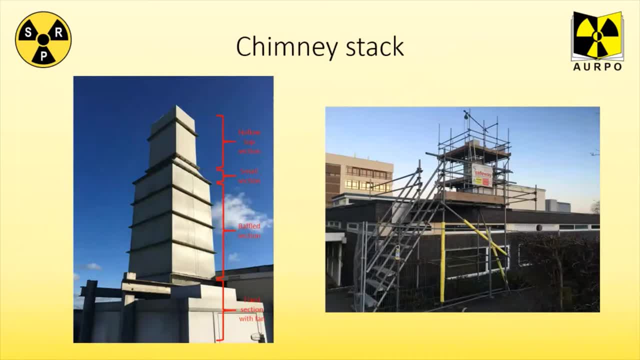 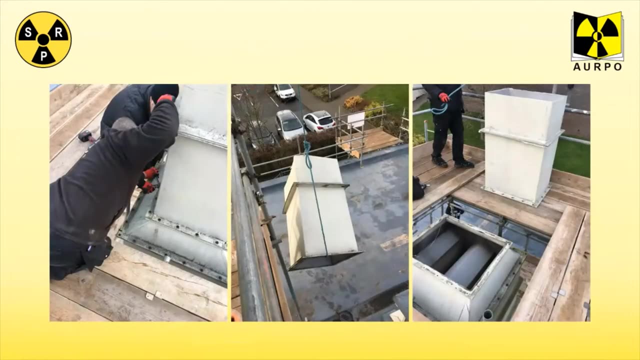 into several sections: the thick section with the fan, integral to the roof and really can't be moved, and the top sections, which are much smaller but are pretty hollow. so what did we do? you can see our facilities staff. so the chimney was monitored on the outside to make sure it was reasonably okay. 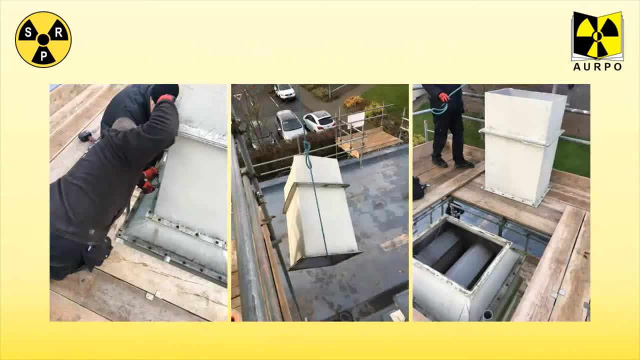 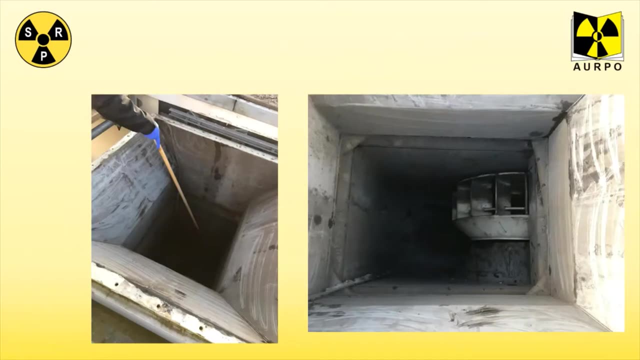 for our facility staff to go up there. it was dismantled and sections were levered off the side of the building, on the right hand side, you can see some of the baffled sections there. so of course the fan section we couldn't remove, but we could get down and wipe test sections of. 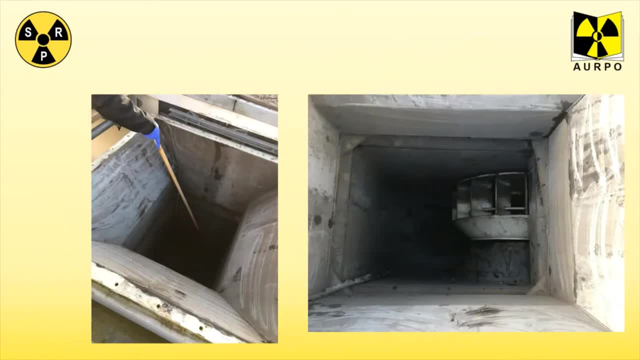 it and on the right hand side there's the fan. you can see very old looking but actually not contaminated, which was really pleasing. here are some of the sections that we had in the lab that we can now test properly. so we monitored the outside when we were dismantling, but now we wanted 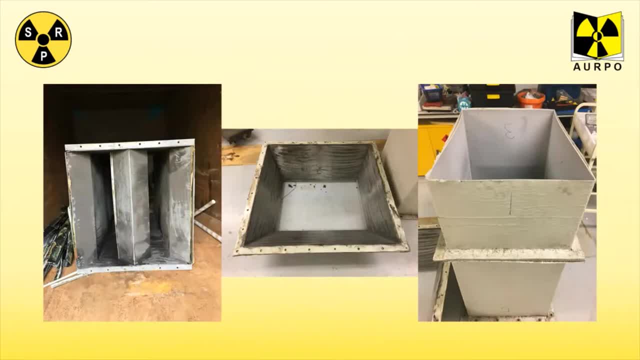 to wipe test all the sections to make sure there really wasn't any contamination, and we'll just wait for my computer to catch up. bear with me one moment. so the next slide. we'll show you, when it gets to it, a diagram of the baffled section of a chimney and also the photograph and the wipe test results that we got. 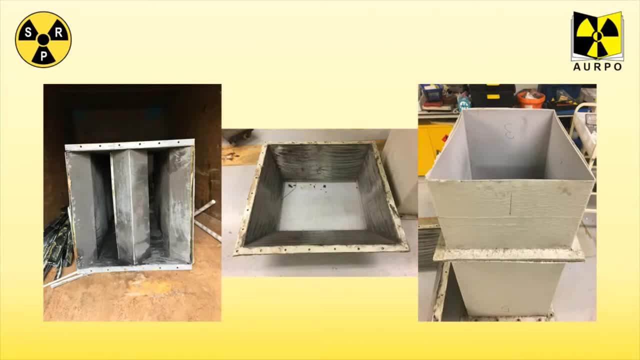 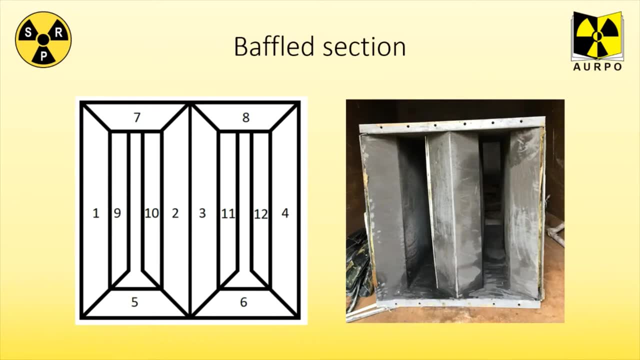 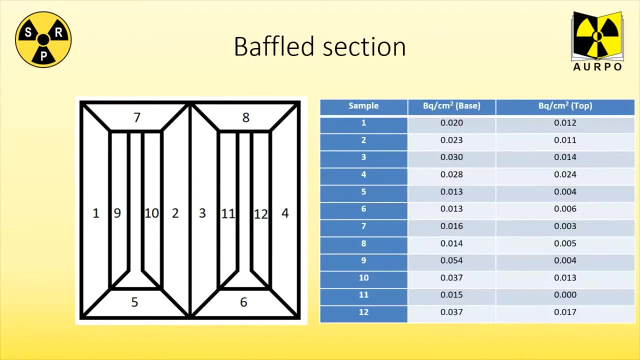 for it. here it is eventually, so you can see the diagram represents that baffled section. and then all the wipe tests. we would label one, two, seven, etc. so we could correspond that to the results to make sure that we knew what was contaminated and what wasn't. and here you've got those samples. 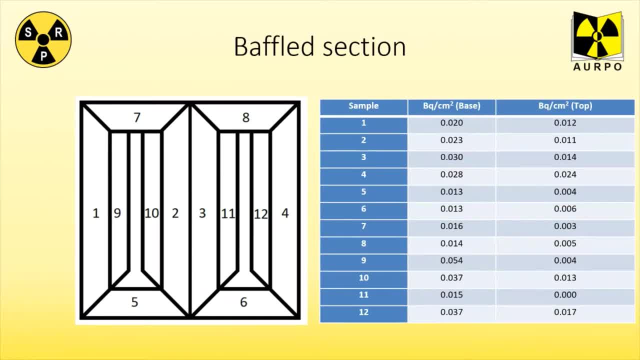 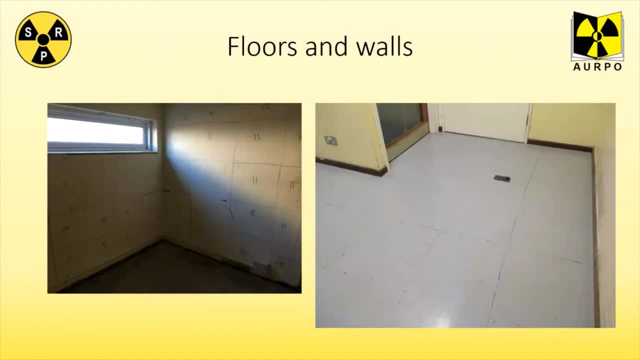 beck was per centimeter cube for the base and on the top. so very clear, very. and there was a few areas which were slightly contaminated, but once cleaned with decon, completely fine. then the floors and walls were done in parallel with some of the other work, but i just kept this at the end, so you 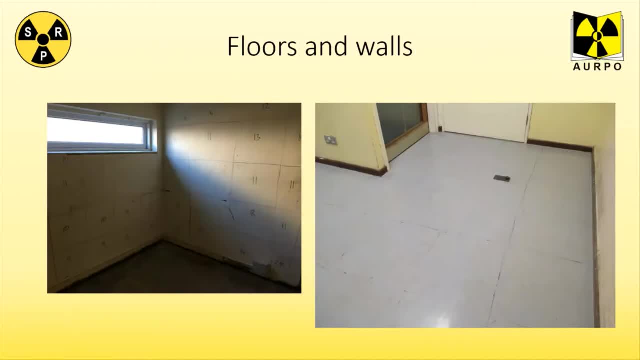 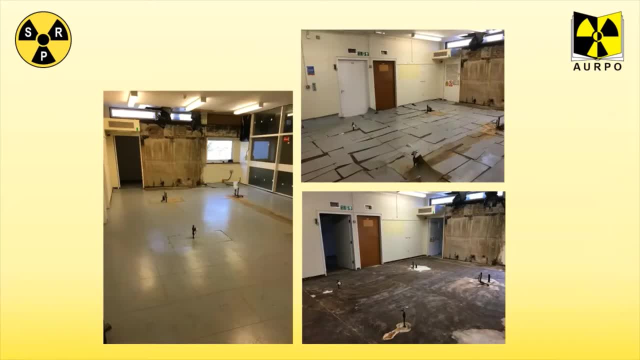 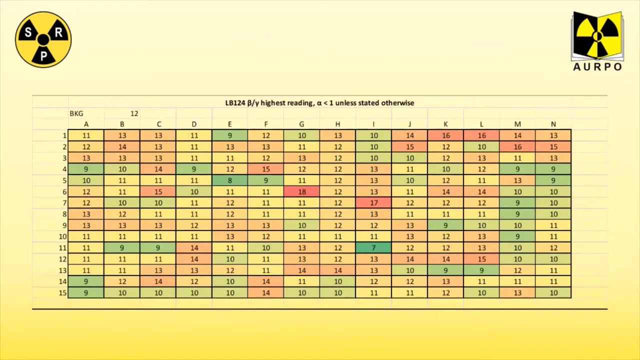 we could monitor the underneath of the floor to make sure the concrete wasn't contaminated as well. each x section would have tables like this, so this is a section of one of the labs and this is the monitoring done by the alb124 monitor, and there'll also be 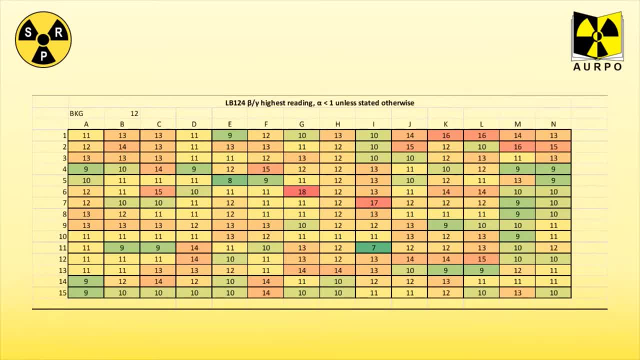 another one for the liquid scintillation results. so where it's slightly redder is where we had slightly higher elements, but you notice the background was 12 and the highest one we got was a count of 18 on the dose rate meter, so the contamination monitor. but we also had liquid. 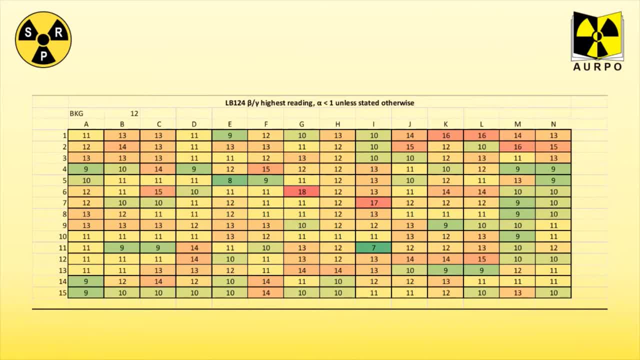 scintillation counting done at the same time. my wi-fi is really not happy today, so, unfortunately, what we did find while we're doing the survey of the concrete floor is contamination within the concrete underneath one of the fume hoods, and once we get the slide, i'll be able to show you. 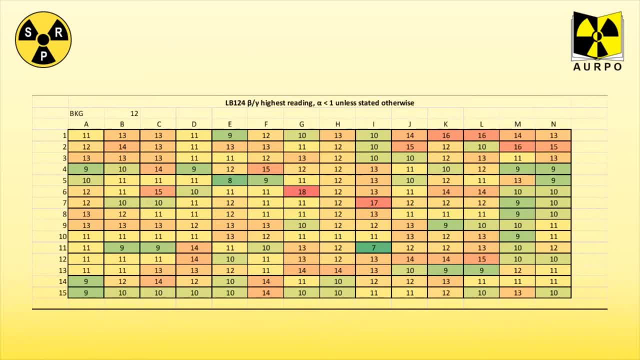 let me just get it so while we're waiting, the contamination measured 14 microsieverts an hour on the dose rate meter and 950 counts per second on the alb124. so it wasn't a massive contamination, but it was there. the spectrum analysis confirmed it to be nickel 63 and of 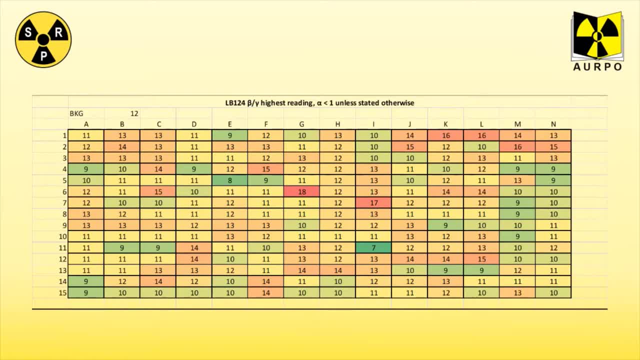 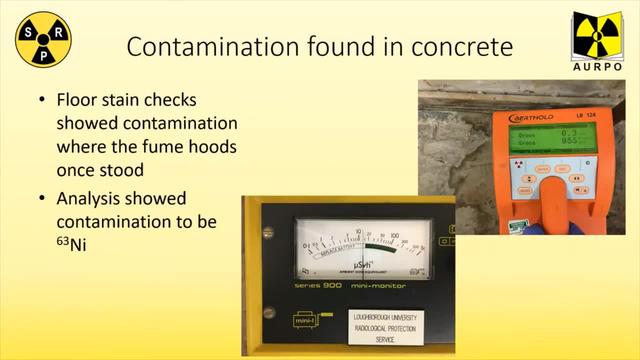 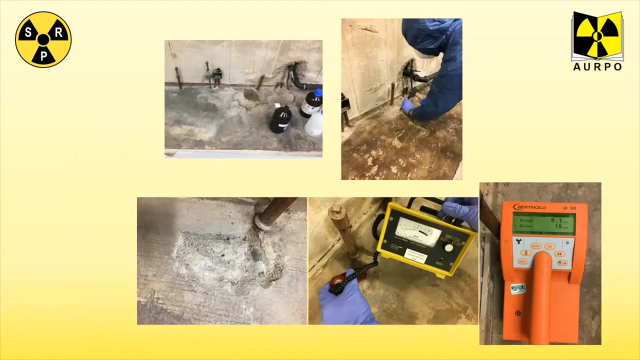 course we did use nickel 63 quite a lot in the um since the 1970 something, so it was a little bit more time used. but it's worth mentioning that i took a lot of work here, so the more we looked at, the every time we found contamination. we take photographs of the 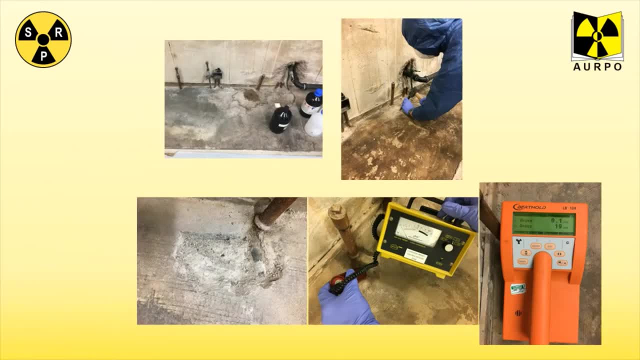 monitors and say this is what we found, monitored the flooring to make sure it was now background levels, as you can see in these pictures here. So for drains: so in 2012 we had a survey of our drains to see what type of contamination we 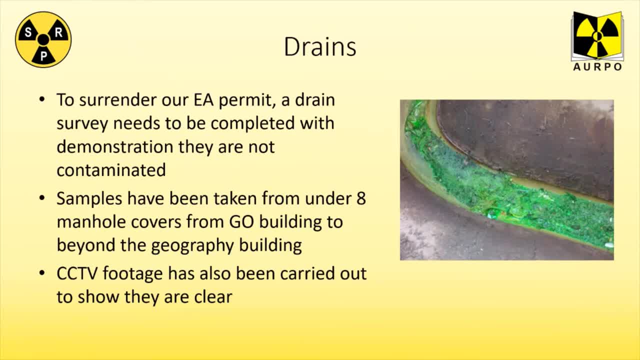 had and the only contamination it showed was the manhole directly outside the building. There was a little bit of sediment, a little bit of contamination. that was removed and dealt with at the time. What we also did was put coloured dye into the drains to make sure that the map we had 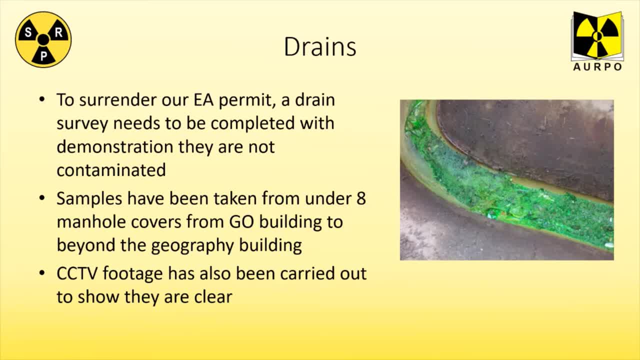 of the drains was actually accurate so we could see where the coloured water would go to. So what we've done since is we've had a camera footage down there and we've also taken core samples of all of our manholes. So in this slide coming up now you've got the 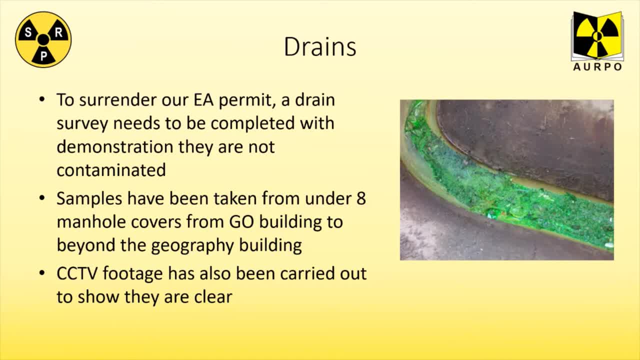 Graham Oldham building, which is on the left of the map and, as you'll see slowly in your slides, all the manhole covers coming up here. we opened and took samples of So 107, which is the one we were expecting to be the most contaminated, all the way round past the old 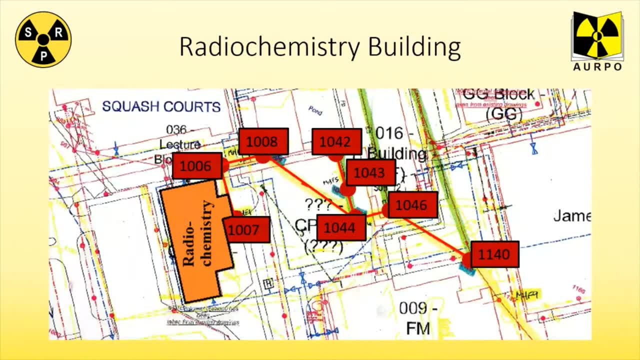 chemistry building down into the car park. We needed to check everything to make sure no contamination had gone down. We also wanted to check for heavy metals as well. So here's a couple of photos of some of the manhole covers. Some of them were deeper than others and there were the 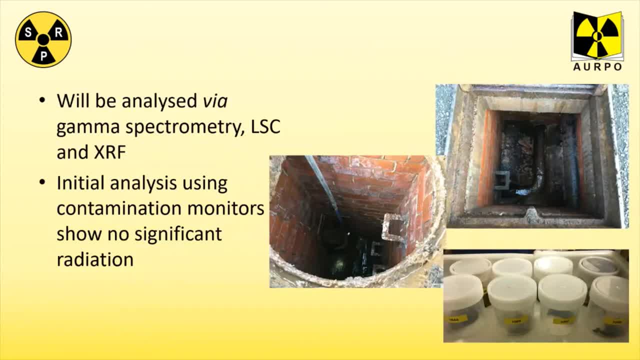 core samples, some of the samples that we'd taken from those drains. The initial analysis shows they're not contaminated, but we also wanted to do gamma spectrometry, liquid scintillation and XRF on those samples. still, too, The camera survey. so we've got a video of what the drains look like. 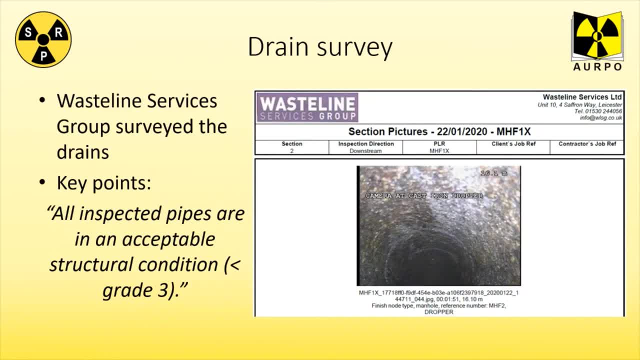 from the inside and here's a photo of one of them. The waistline service group said all the drains were in acceptable structural conditions. So we know the drains aren't leaking or having any issues, which is really reassuring. So this is just very briefly to show you now what the radio 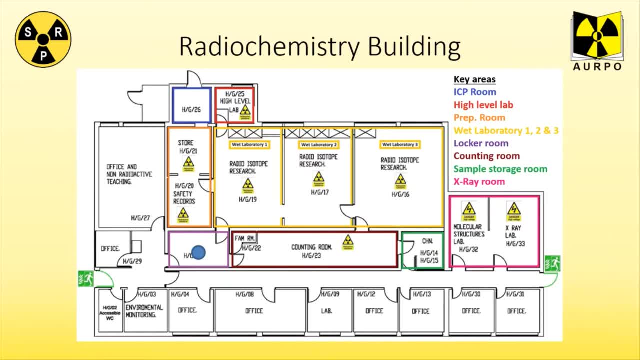 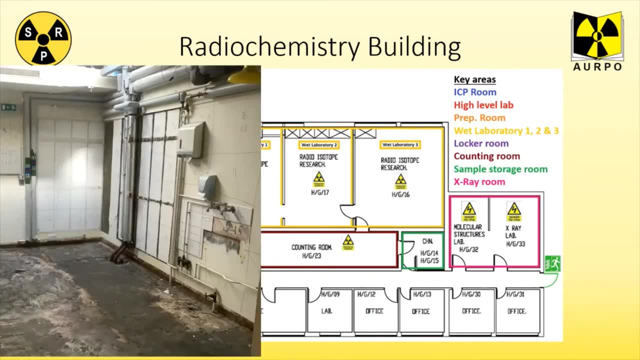 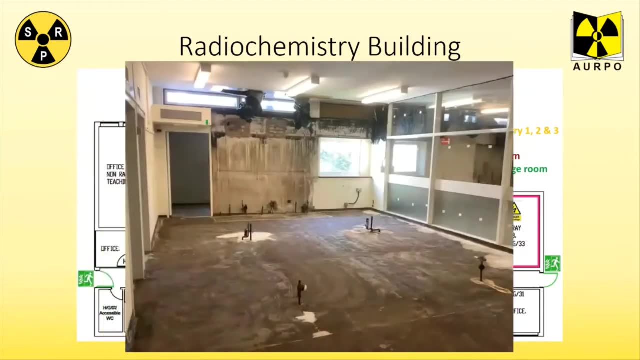 chemistry building looks like As previously, where I showed you the photos. So that was our locker room. now just a picture of grids and concrete floor. Don't worry if I whiz through some of these too quickly, because it's now just basically empty floors. That's our first lab, So you can see the pipe coming up from where. 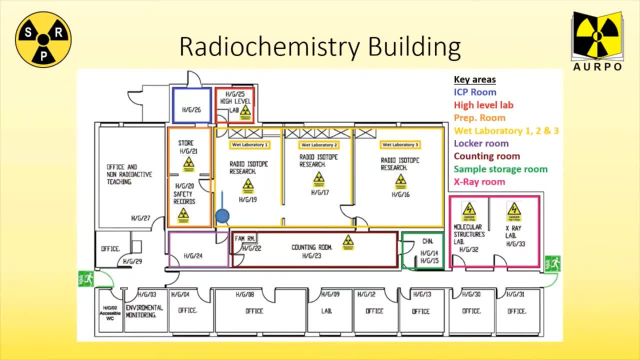 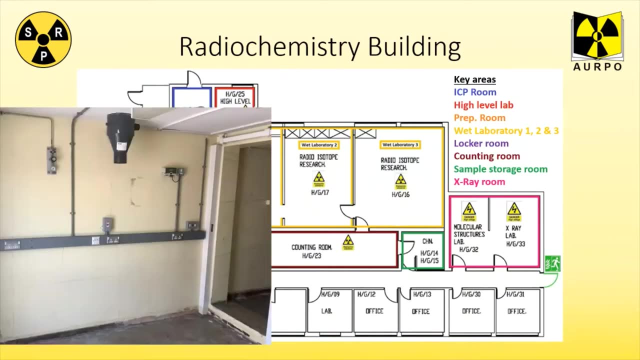 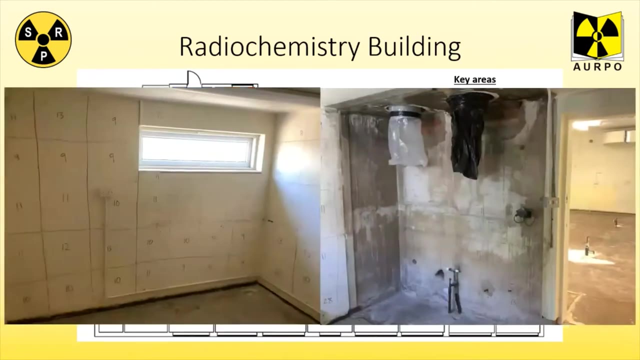 the sinks would have been into what was our prep area- completely empty both sides- And the ICP area now completely empty. But this just gives you an example of just how much wipe testing monitoring has been carried out in this building. That's our high activity lab. 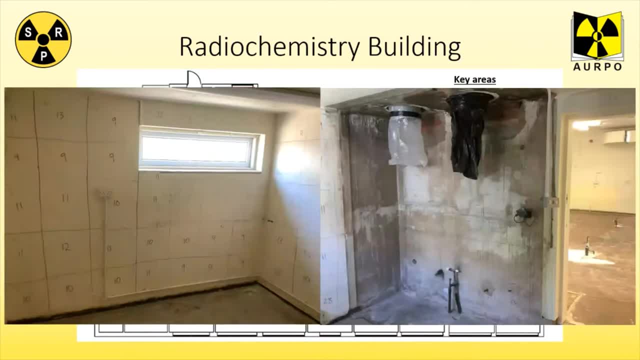 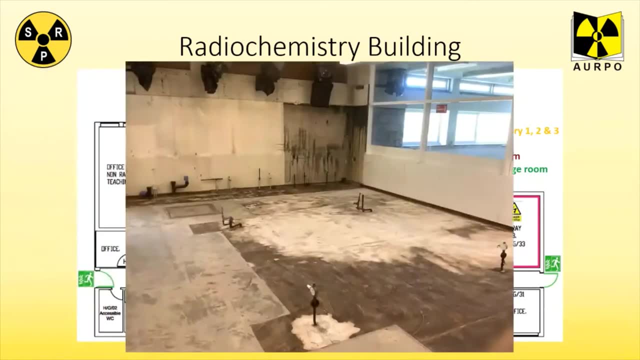 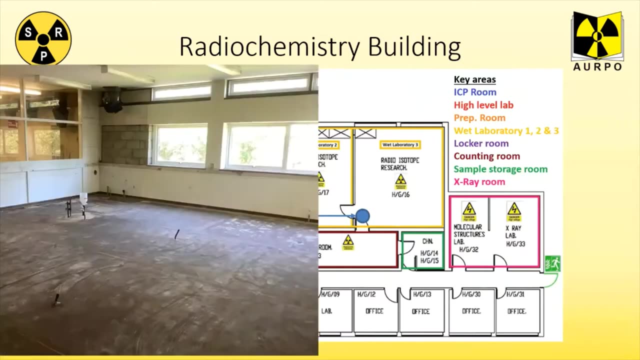 no longer got the sink, no longer got the fume hoods. Our second main research area, completely empty. This is where you can see some of that fire damage again. And our third research area, The counting room. now all the equipment has moved to our new health and safety lab, so that could. 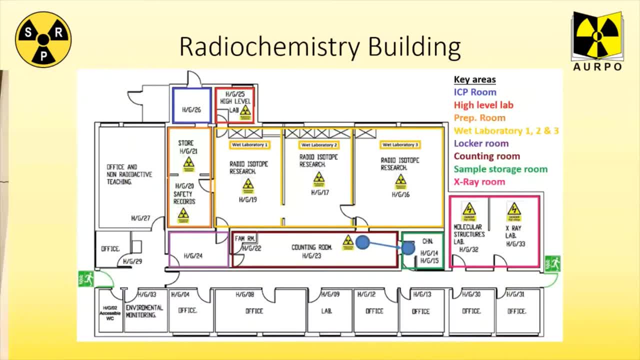 be emptied And of course the storeroom. that was pretty empty anyway, but now is too. The XRD area had four XRDs. two of them went up to our new chemistry facility, the other two were decommissioned, So the X-ray head was taken by hazardous waste because it contains beryllium. 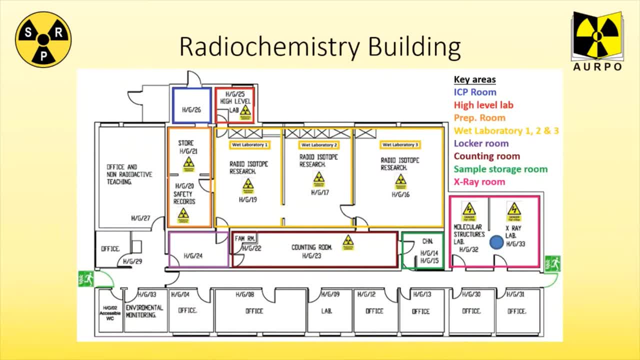 and the rest went by wee. But that room was also wiped, test and checked because occasionally they did run radioactivity monitoring. So that's where you can see the XRDs and the XRDs were also wiped samples in there. So we just wanted to be thorough, so we did wipe, test and check that room as well. 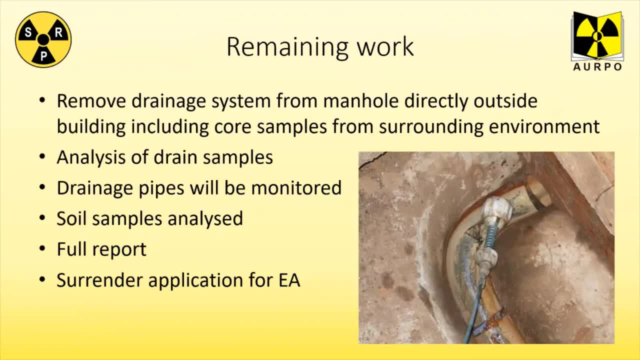 So what we have left to do not very much anymore. All we need to do is analysis of the drain samples. We need to remove the drainage system from the manhole cover directly outside the building. We decided. although we're not picking up much contamination, it would be good practice. 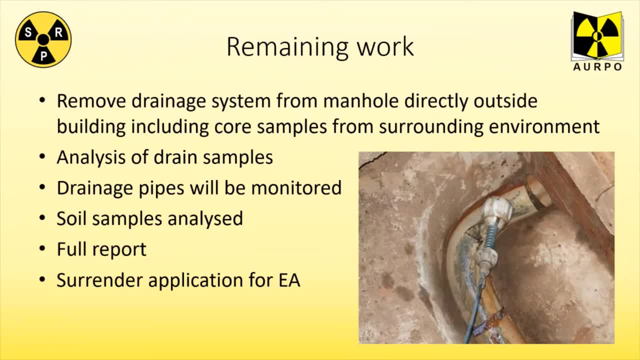 best practice to remove that and thoroughly check it within the lab. So all that on this picture here you can see all this pipework. we're going to take it all up. The pipework you see on the photo is from a manhole cover when it came loose. So we're going. 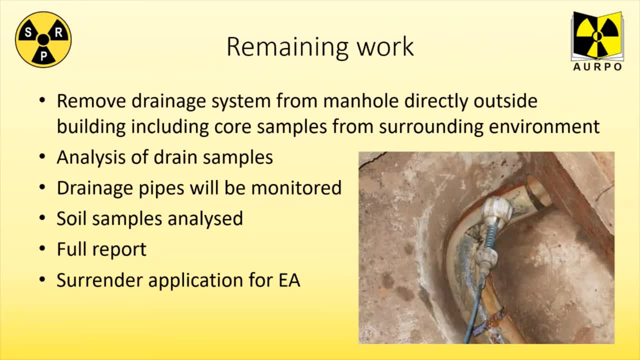 to take all of that up and do the analysis of it, of the gamma spec, alpha spec, etc. We are going to take soil samples from around to make sure that that's okay and finish all the drainage. We're then going to do a full report for our records. 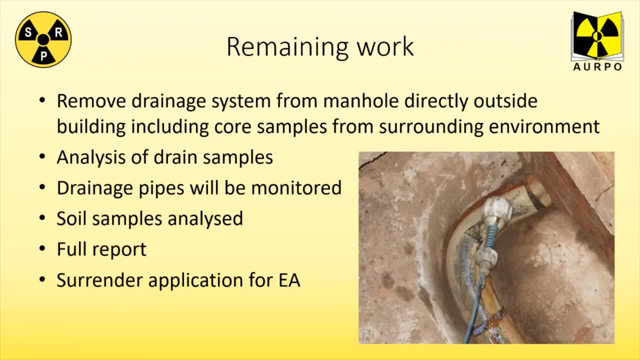 which is going to have all the photographs in all the wipe test records. So we have got a historical report that if someone in 20 years comes back and asks that question, we've got it all. And then we're going to go through the surrender application process for the Environment Agency. 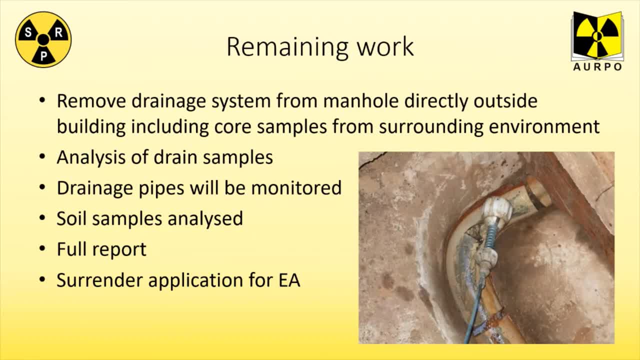 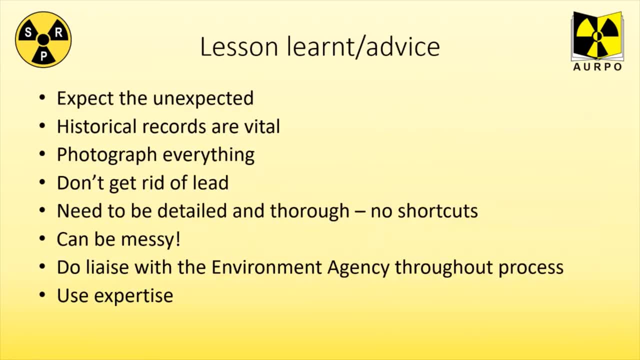 with their documentation and provide the Environment Agency what they've asked us for, Just some key lessons learned. Do expect the unexpected. We have found that contamination in strange places, we found that fire damage, we found asbestos. we found interesting things. But the most important thing it's shown is that historical records are vital. 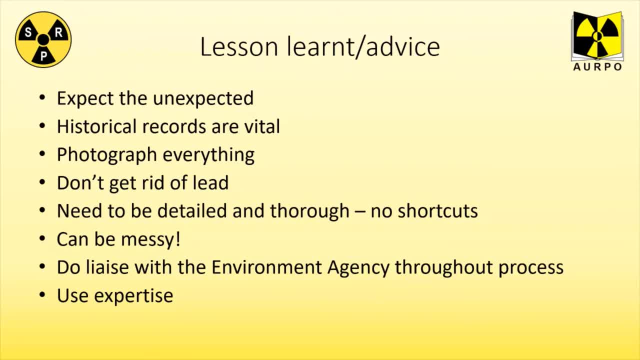 So if you're a new RPO, now look at what you're doing now. Now record it, photograph and keep it, because it is so useful. Photograph everything. Really can't tell you how brilliant it is to do that. Another lesson is: don't get rid of that two ton of lead that we got rid of because after we disposed of it through a lead merchant.